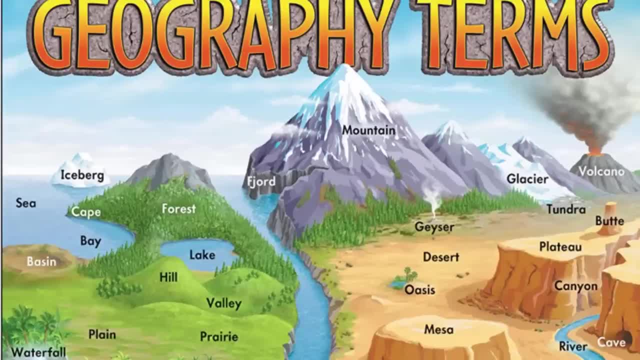 Alright, then, without any further ado, let's begin. I am going to use this picture as a reference and I will explain properly all the terms that you see in this picture. Please bear with me for the next few minutes. I know you will have many questions regarding these landforms and their different types. I will keep my 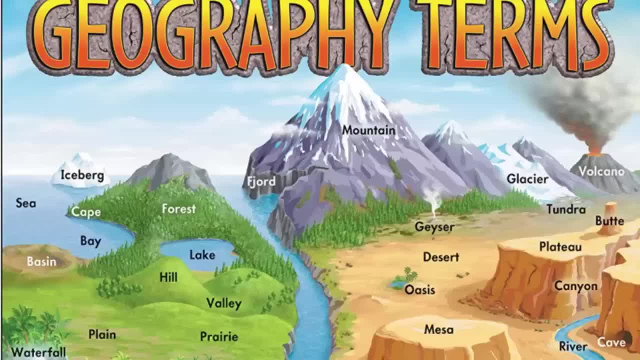 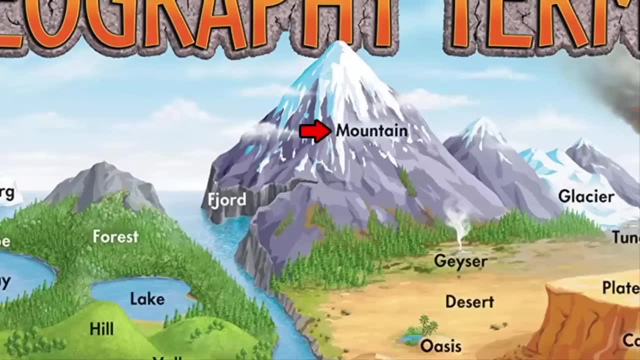 explanation strictly to all that you can see in this picture for the benefit of keeping it short and crisp. So if you have any question, put it down in the comments section. If you look at a mountain, they are formed due to the movements of tectonic plates. They 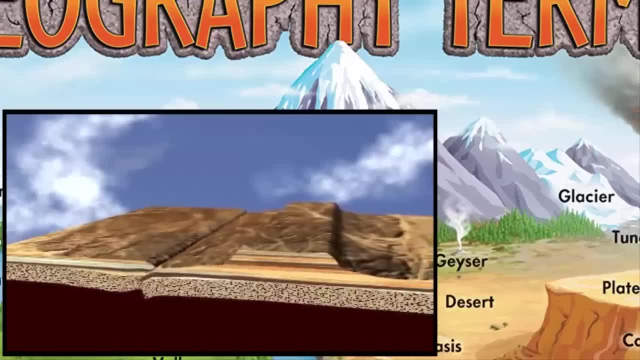 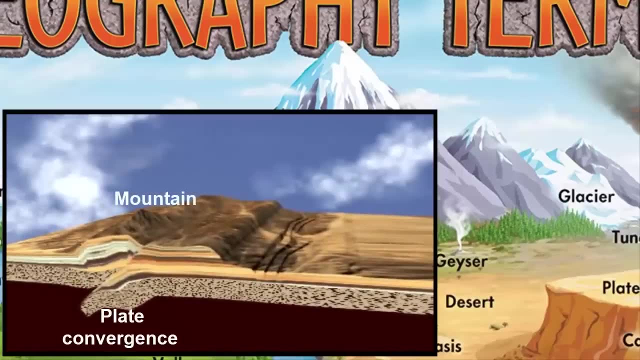 are formed by slow but gigantic movement of the earth's crust. This is called plate convergence. When two continental plates collide, it pushes the rocks upward and that forms a mountain range. A good example is the Himalayan mountain range. They were formed as a result of the collision. 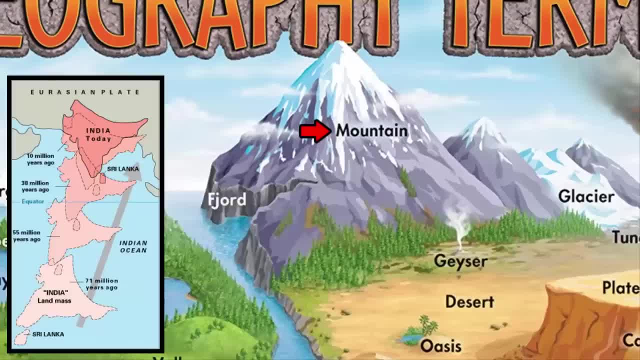 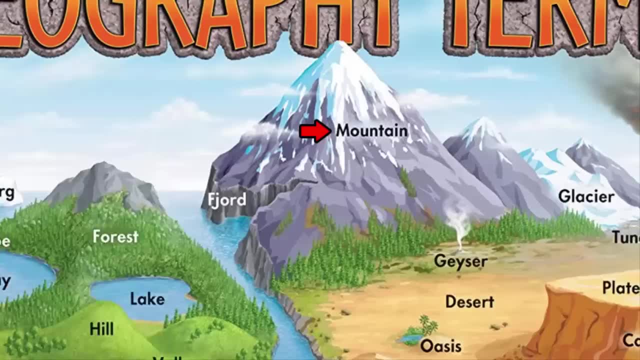 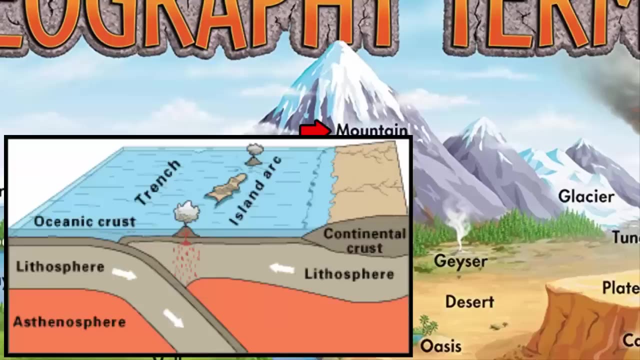 between the Indian plate and the Eurasian plate, which began 50 million years ago and it still continues today. So this is how the mountains are formed. You will also find many mountains near coastal areas. These are formed when heavy oceanic plate collides with a lighter continental plate. The oceanic plate sinks beneath the 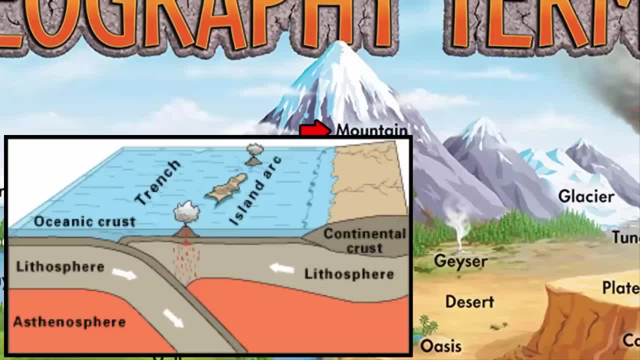 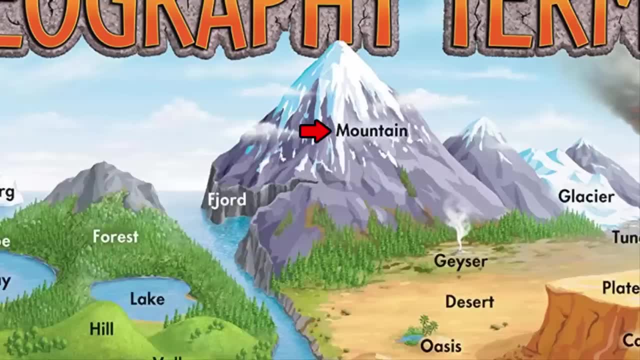 lighter continental plate, which results in coastal mountain ranges like the Andes, the Western Ghats, the Aleutians, the Japanese and the Southern Alps. Now the next question is why there is a snow on top of the mountains. These are called snow-capped mountains. The top of the mountain is actually its coldest spot. Now you might. 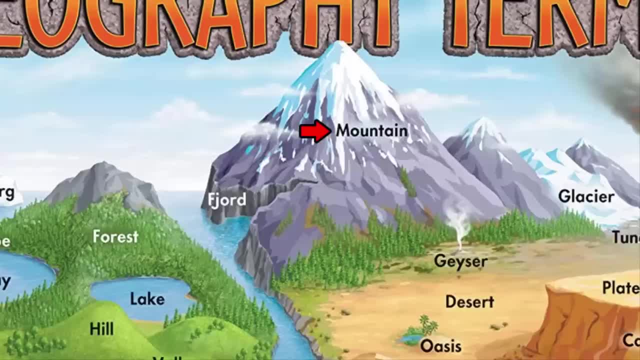 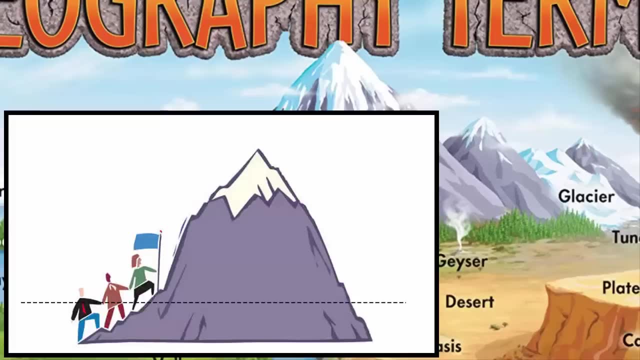 have another question. since the top of a mountain is closer to the sun, it should be warm, And doesn't the heat rise? so why is there snow Now? if you climb a mountain to a higher altitude, the atmosphere gets thinner and thinner, So 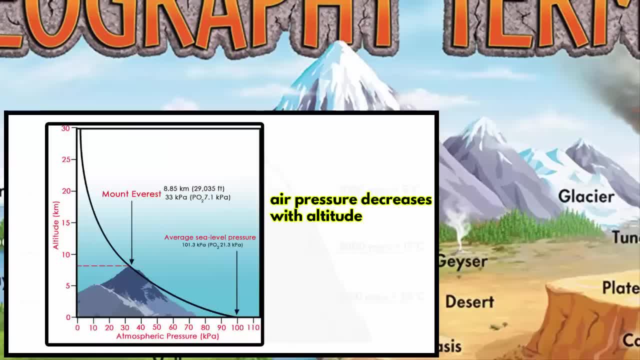 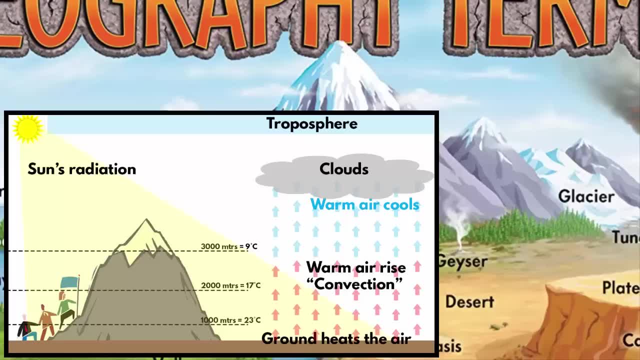 this is because air pressure decreases with altitude. When warm air rises, it expands and cools as the altitude increases. Due to that, the warm air cannot absorb and retain the heat the way it does at the bottom of the mountain, Although mountain tops are closer. 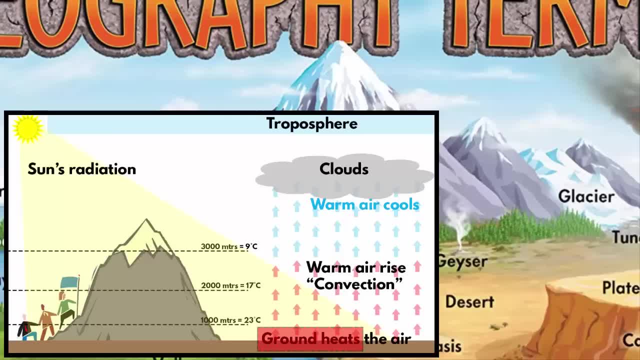 to the sun. they are also farther away from the thermal heat of the earth's core that keeps the ground warm, So the top of the mountain can be much colder than the bottom. Cooler than the bottom means that there is less evaporation taking place. This leads to greater amounts. 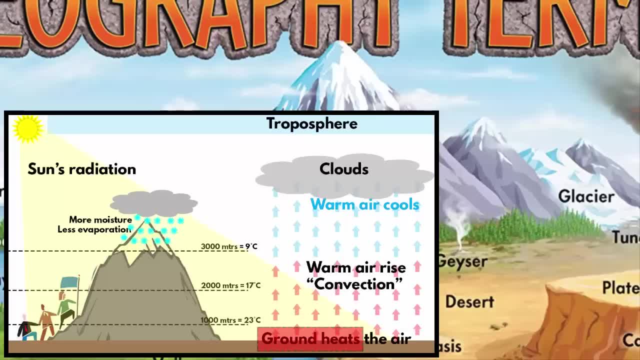 of moisture in the air. More moisture means more rain, But when you are at the top of a mountain, instead of rain it snows, And that's how you get a snow-capped mountain. By the way, not all mountains have snow caps and not all mountains that get snow have. 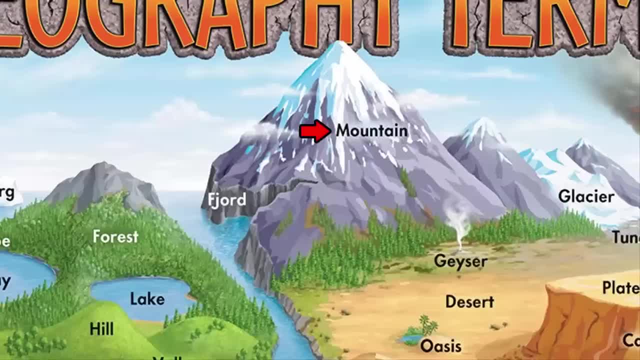 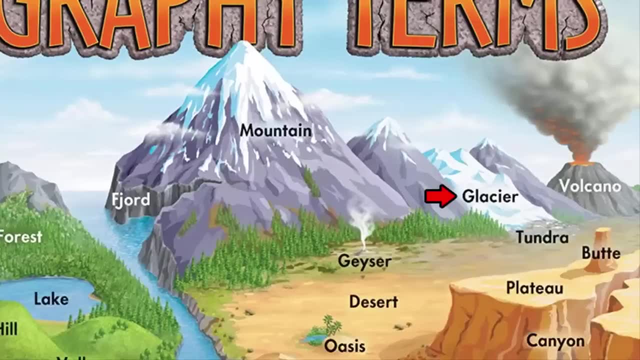 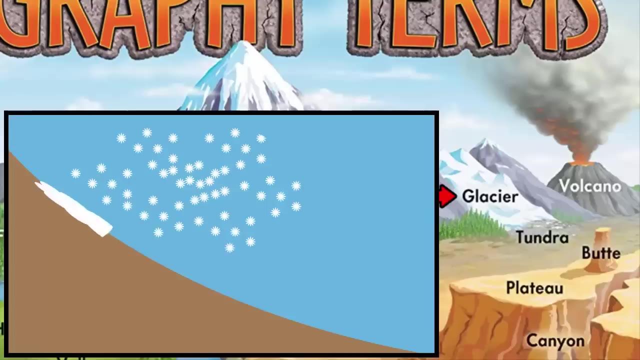 snow caps throughout the year. It all depends upon the location and how tall they are. Now coming to glaciers. How are glaciers formed? It is very easy to understand: Glaciers begin to form when snow remains in the same area for a very long time. I am talking about an entire year This way. each year, a new layer. 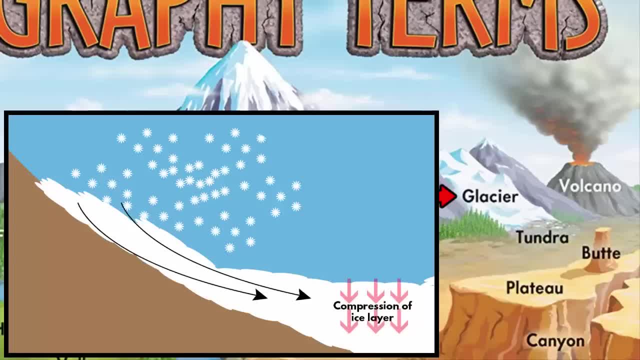 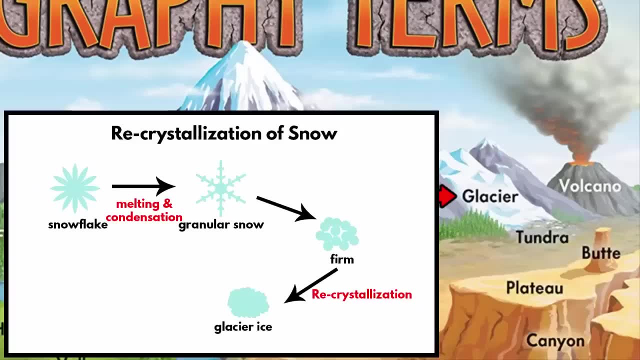 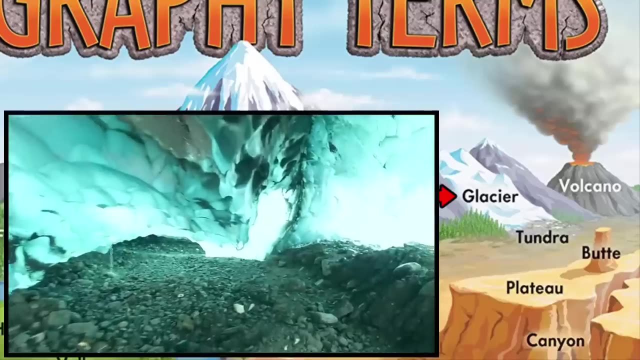 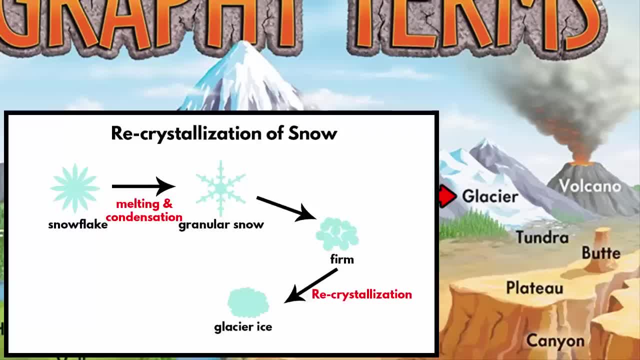 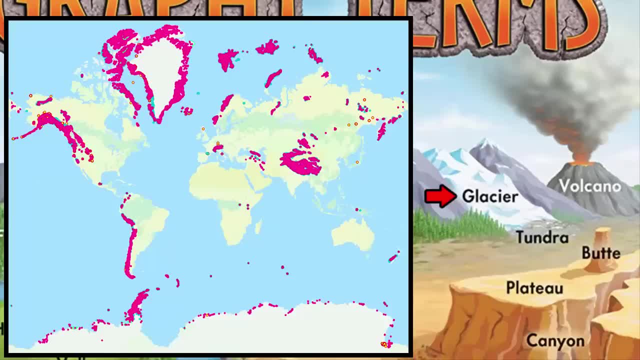 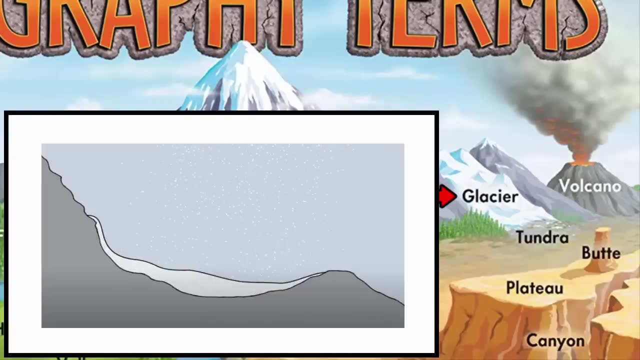 of a glacier is a layer of snow. Most of the water recrystallizes before it melts. Here is the map that shows where in the world you will find glaciers. Mostly, glaciers occur in high latitude and high altitude regions. Glaciers are usually formed on steep slopes. I mean, this is the place of their accumulation. 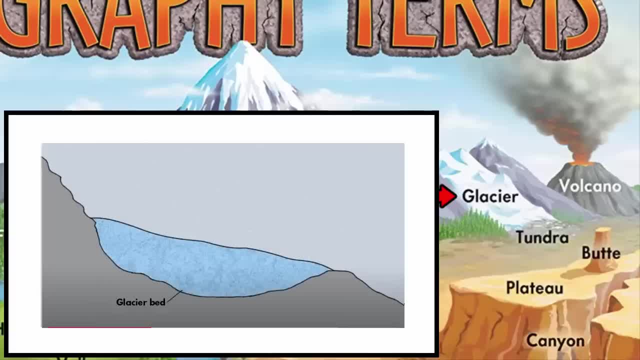 And if you look at the movement of glaciers- the bottom layer of the glacier, which is also called the glacier bed- it starts to melt And that reduces the friction between the glacier and the snow, the bedrock, making the entire glacier slowly move. Now, when a big piece of ice 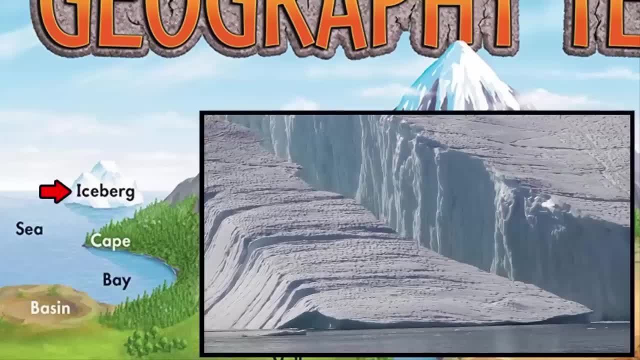 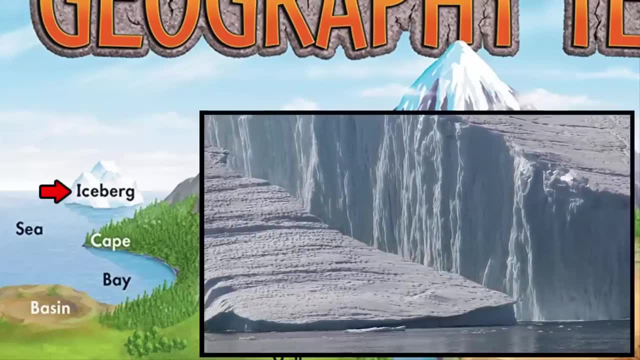 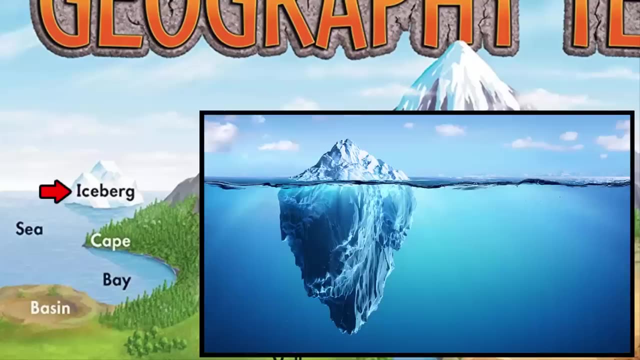 breaks from a glacier and reaches open sea or ocean water. that is known as iceberg. By the way, glacier is a freshwater source. Please keep that in mind. So iceberg is a large piece of freshwater ice floating in the open water. If you ever see an iceberg, only the tip of the iceberg is visible above. 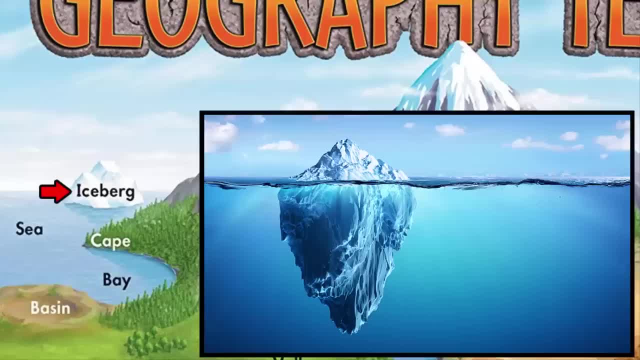 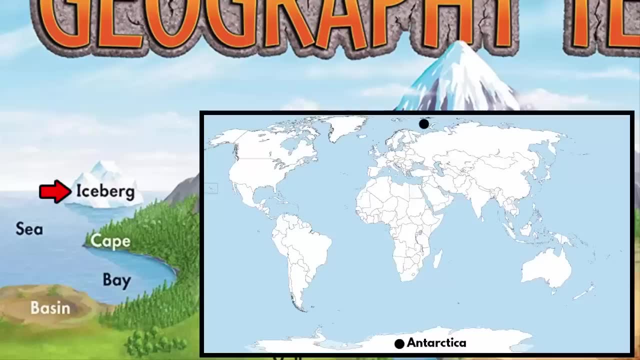 water, while nearly 90% of it is underwater. After all, it's a heavy piece of glacier. Glaciers are commonly found in high latitude regions like Antarctica and Arctic region, which consists of places like Alaska, Finland, Greenland, Iceland, Northern Canada. 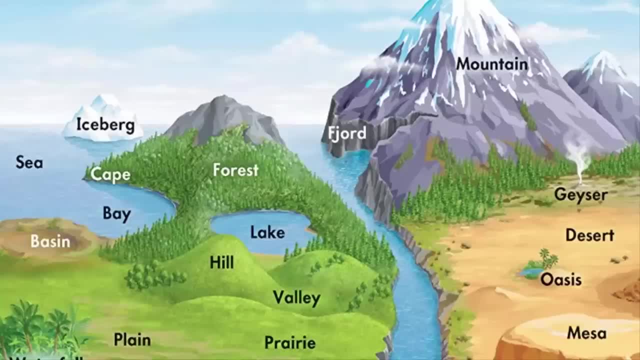 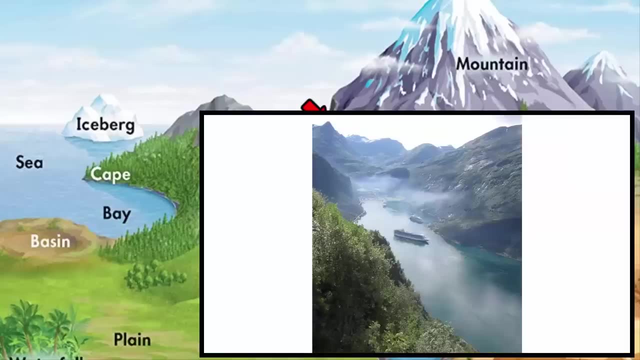 Norway, Russia and Sweden. The next one is Jord. The F word is silent when you pronounce it. These are a long, narrow, deep inlet of the sea between high altitudes and high- nice quote guys- high cliffs. How are they formed? They are created by glaciers. I just told you how glaciers 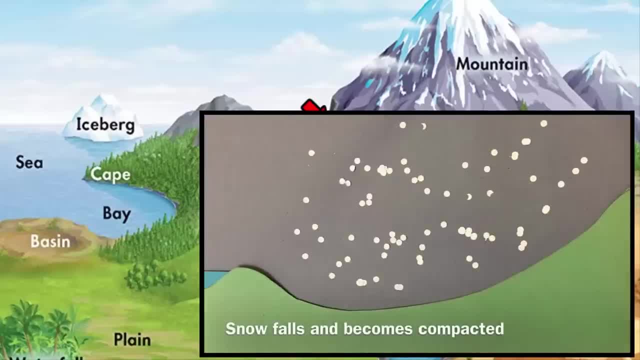 are formed right. Glaciers move downslope very slowly over time and can greatly alter the landscape once they have moved through an area. When a glacier starts to move, it starts to carve the valley and forms a land depression. This carving of the steep valley- 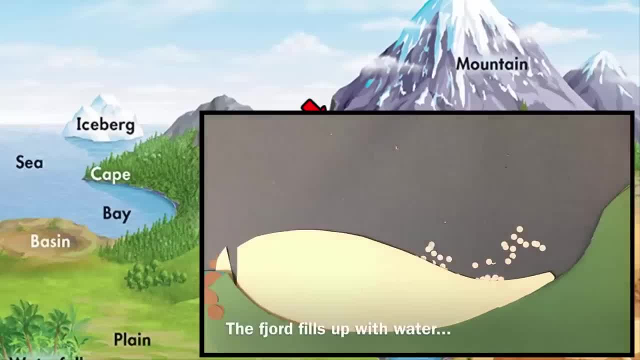 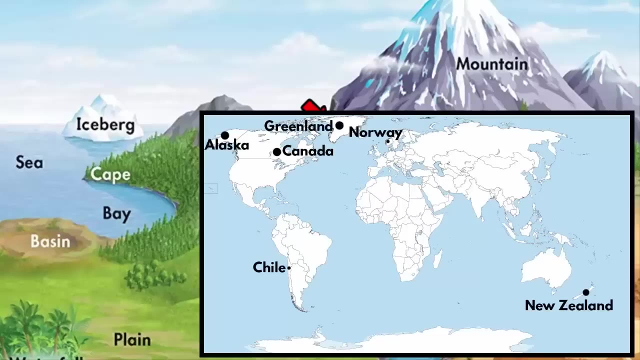 is known as jod. A jod is often deeper than the open sea. It can be thousands of meters deep. As a result, water fills up and forms a deep inlet of the sea. Jods are found mainly in Norway, Chile, New Zealand, Canada, Greenland and the state of Alaska in US. Jods are home. 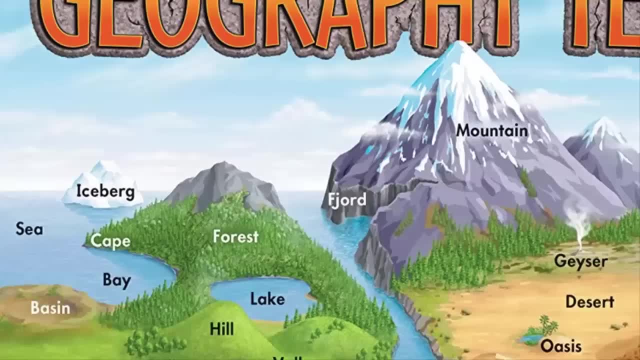 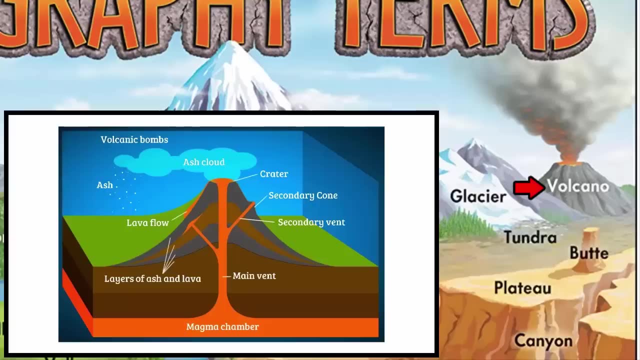 to several types of fish: plankton and coral reefs. Now coming to a volcano. Volcanoes are found when magma comes out within the earth's upper mantle. Now how does magma comes out of the earth's crust? It can happen in two. 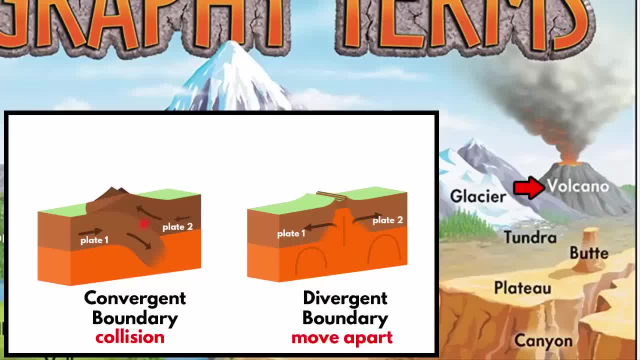 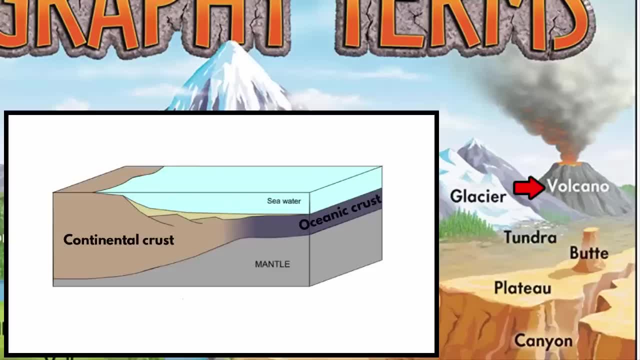 ways When two tectonic plates collide Or when two tectonic plates move apart. Now you need to understand that tectonic plates are of two types: One is a continental plate and the other is an oceanic plate. When these 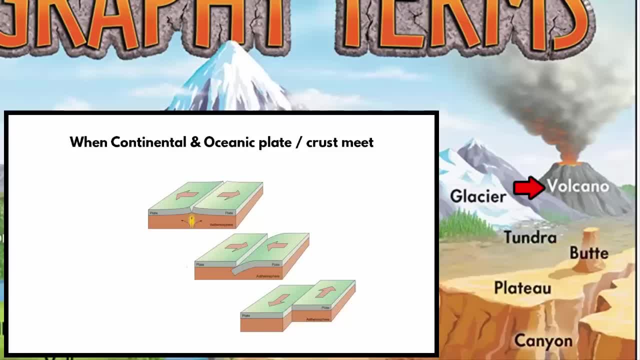 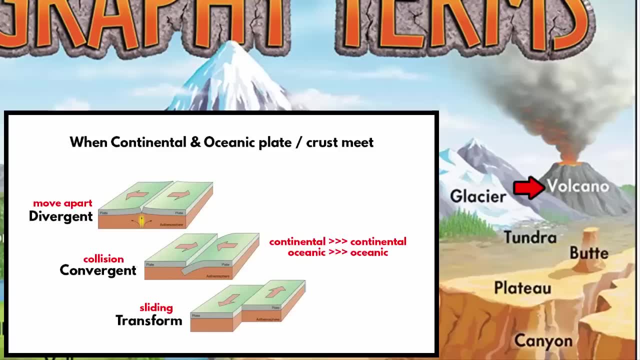 two tectonic plates meet. three types of boundaries are found: Convergent, Divergent and Transform. Several events can occur. The collision can occur between two continental plates, two oceanic plates, or between an oceanic plate and a continental plate. Mountains are usually. 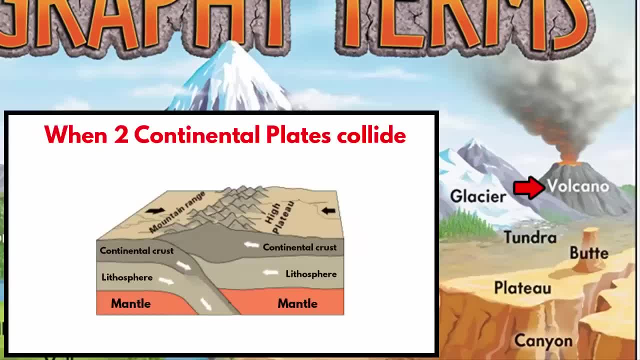 formed when two continental plates converge or collide. So what happens when two tectonic plates collide? When two tectonic plates collide, they crash like cars. If the same kind of plate collides, they crash like cars. They typically bend, break and crumble, creating folds and mountain ranges like the Andes. 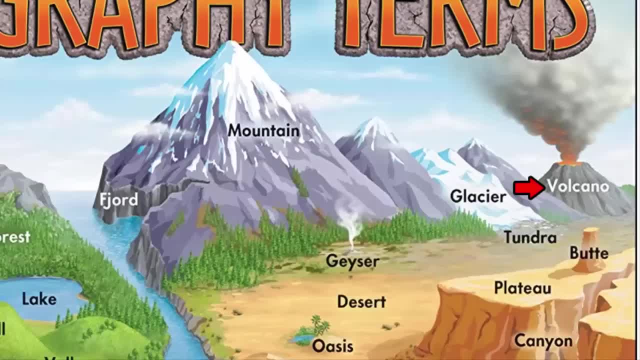 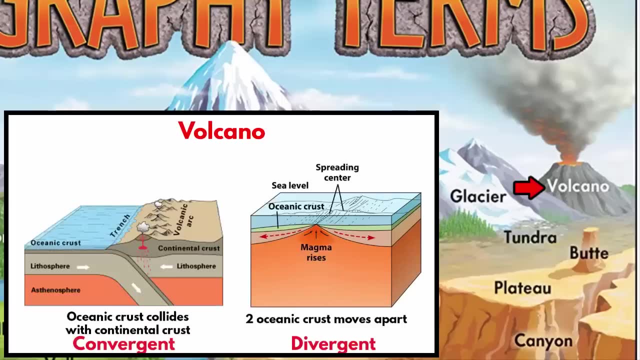 Swiss Alps and the Himalayas. When it comes to a volcano, it occurs in area where oceanic plate collides with continental plates, Or when two oceanic plates collide as well as move apart from each other. When an oceanic plate collides with a continental plate, since 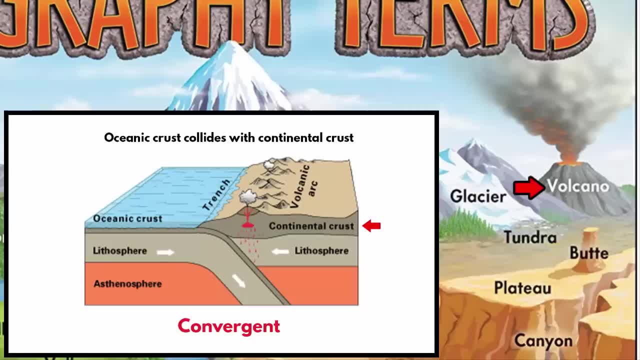 the oceanic plate is denser and heavier than the continental plate. it sinks into the mantle. The mantle is the layer that has magma. When the oceanic plate comes in contact with the magma, it creates huge pressure that causes the magma to push through holes or cracks. 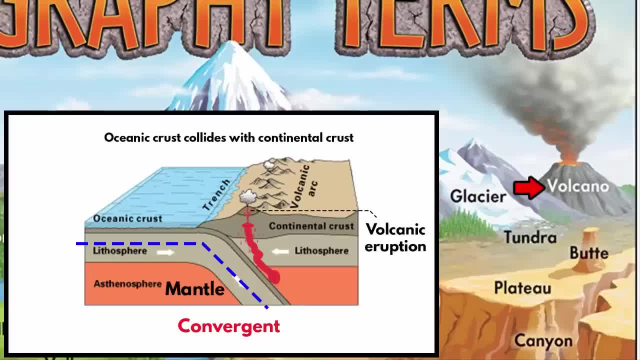 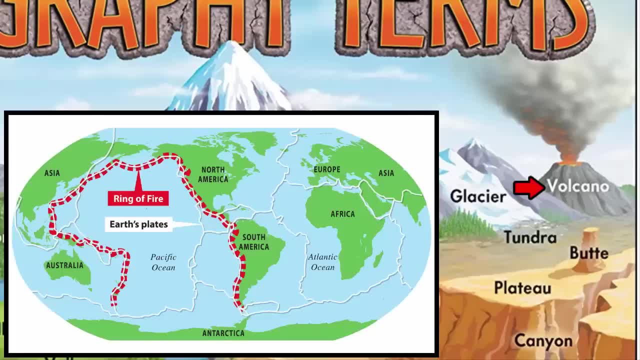 of the continental crust, causing a volcanic eruption. A good example is the ring of fire in the pacific ocean. The ring of fire is a ring of volcanoes around the pacific ocean that result from collision of oceanic plates with lighter continental plates. 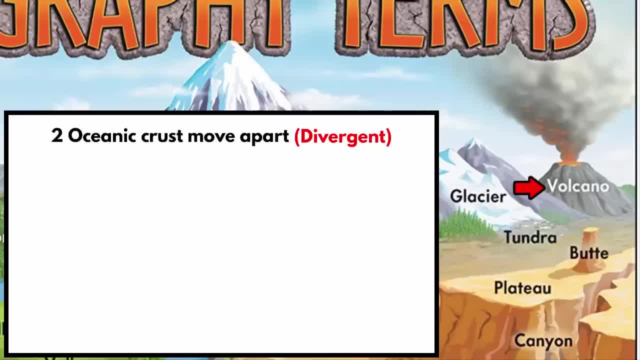 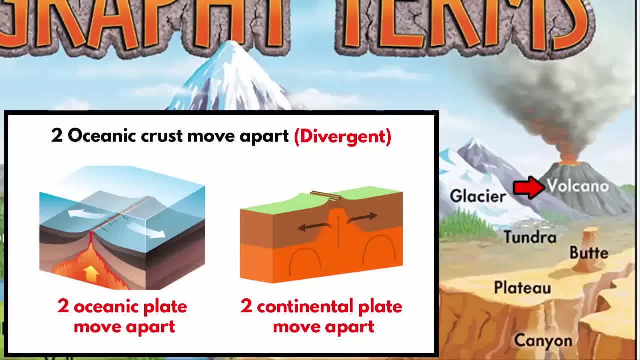 Second scenario: When two tectonic plates move apart from each other, It is called a divergent boundary. It can occur between two oceanic plates or two continental plates. When there is a divergent plate boundary in the ocean, in other words when two oceanic plates are moving away from, 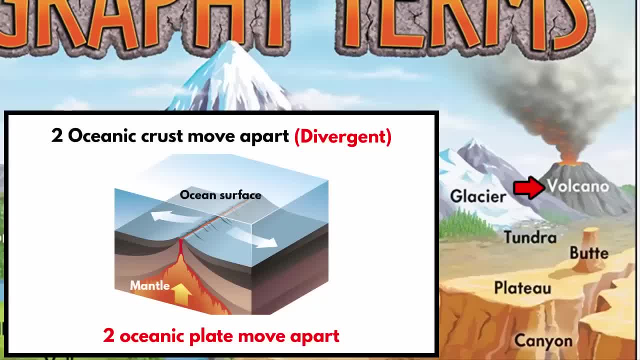 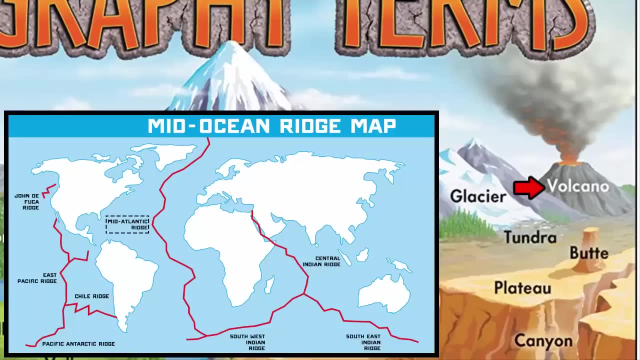 each other. molten basaltic magma from mantle comes up and spreads on the ocean's surface. It is also called a mid-oceanic ridge. When magma comes out, it forms underwater volcano or submarine volcano. In this scenario, it is called a mid-oceanic ridge of Atlantic Ocean, which divides the 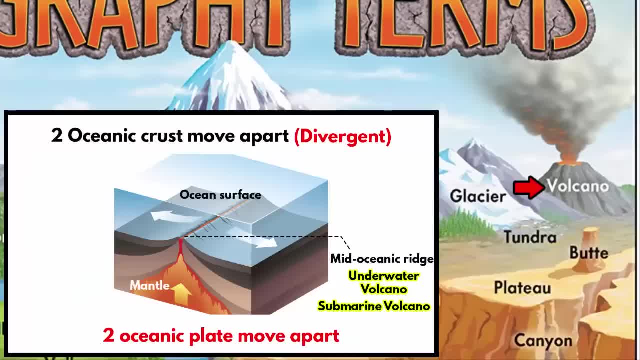 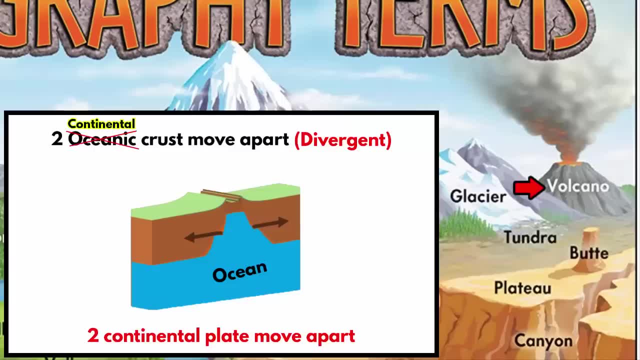 Eurasian plate and the North American plate. Divergence happens in two continental plates too. That's how new ocean forms. Volcanoes are not formed. oceans are formed. The exact reasons as to why it happens where it happens and how it happens are still being studied. The best example on earth today is the narrow. 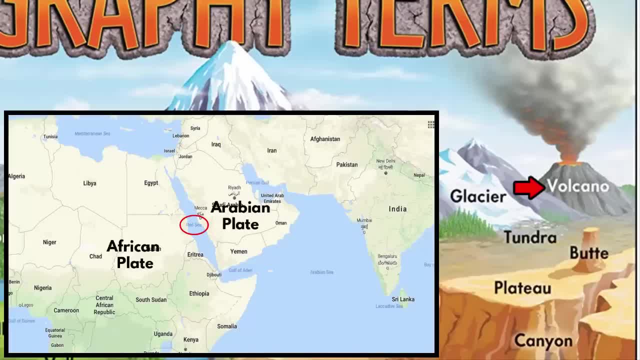 red sea, where the Arabian plate has pulled away from the African plate. It is a perfect example of what happened when two continental plates are in contact. Ten years ago, the Vulcanic plate in the African plate was not formed When a retrophic of the 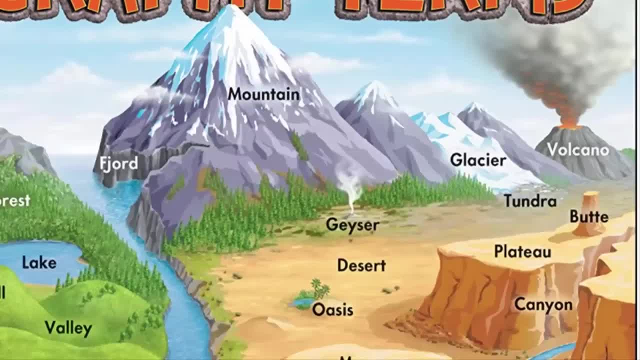 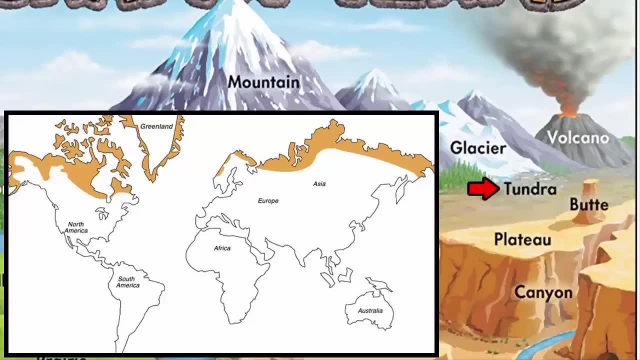 continental plates are moving apart from each other. The next one is tundra region. Now, these are places with low temperature, and you will find them in the north pole, that is, in the earth's northern hemisphere, and also places with high altitude. The land area of North America, Europe and Asia together are often referred to as the 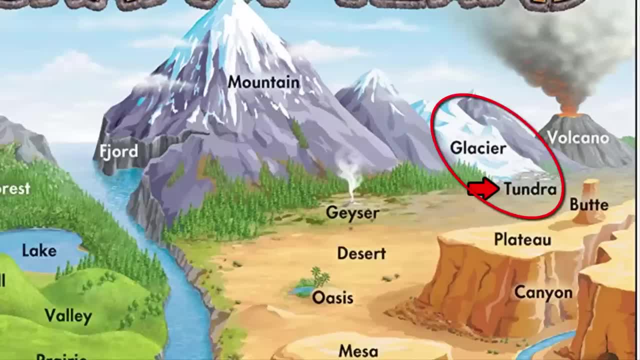 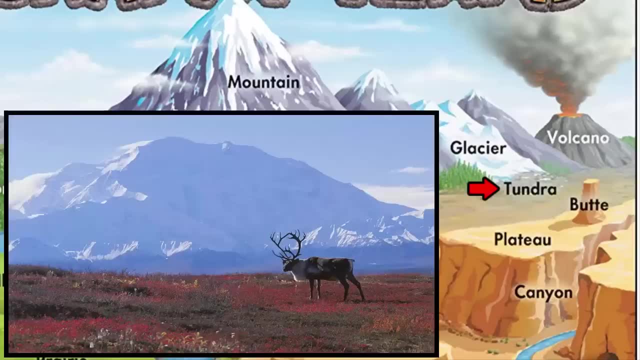 tundra region. In this picture, you can see this region being located just at the bottom of snow capped mountains or glaciers. This is called the alpine tundra region. The word alpine means mountain. In this ecosystem, you will rarely find trees. 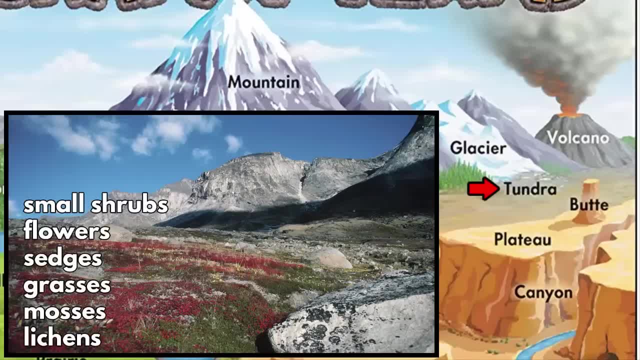 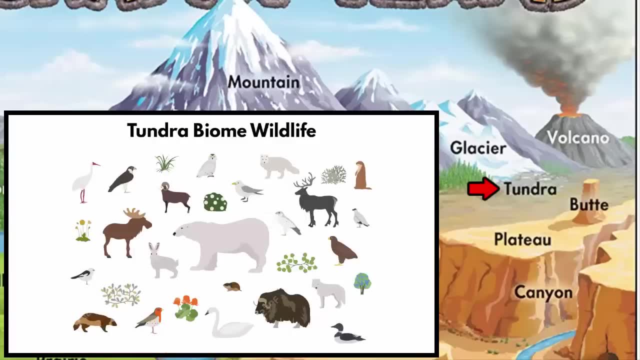 Mostly, you will find small shrubs, flowers, sedges, grasses, mosses and lichens. The wildlife in this region consists of musk, ox, yaks, mountain goats, snowy owls, arctic foxes, polar bear, etc. 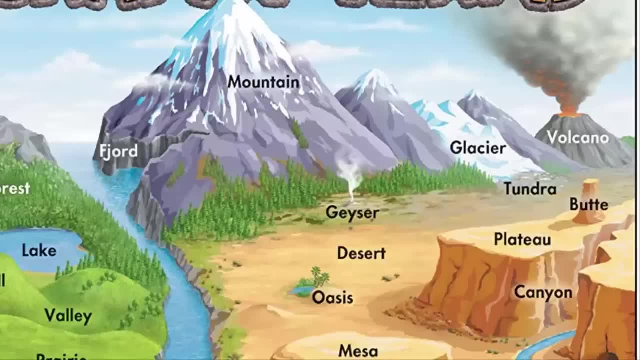 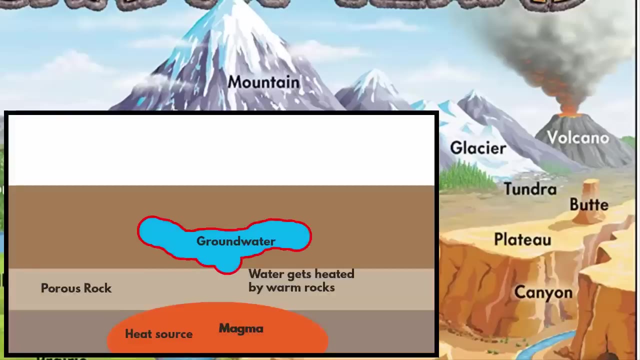 The temperature of this region is mostly dry, cold temperatures. The next one is geyser. Now, geysers are like hot springs, where warm surface water comes out of the ground. So how does the water become so warm When surface water comes in contact with rocks that are heated by magma? 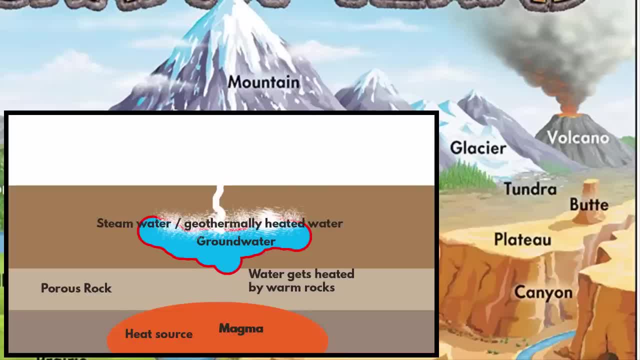 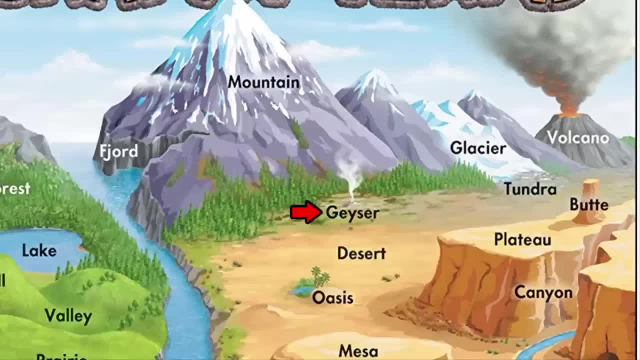 This is called geothermally heated water. It then rises towards the surface by the process of convection, And this warm water comes out of the surface through porous and fractured rocks. You will find many geysers around the world located near rivers, because that is where the groundwater is adequate. If you want to trace the source of these geysers, you will have to go deep into the earth's crust, Because the water in geyser is heated by magma and that lies at least 5 km beneath the surface. 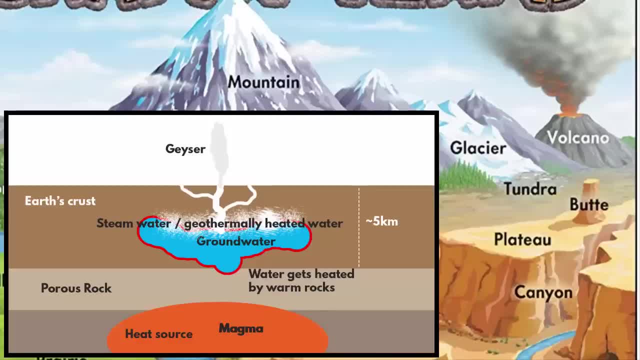 of the earth. At some places, it is not because of the magma, but it is because of the solidification of magma, which turns into igneous rock, And the heat of that rock makes the water boil. One more point you will have to remember is that many geysers are located at the edges. 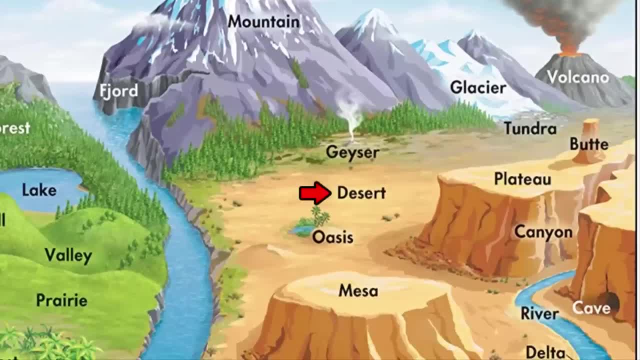 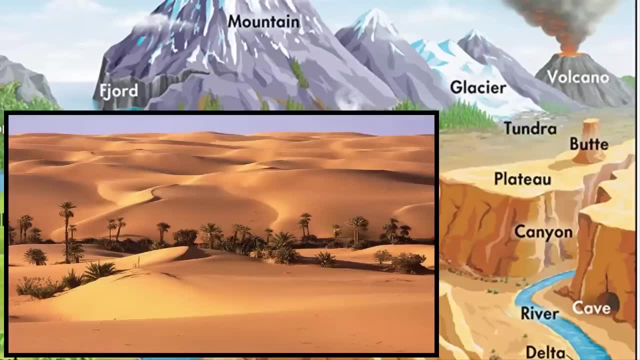 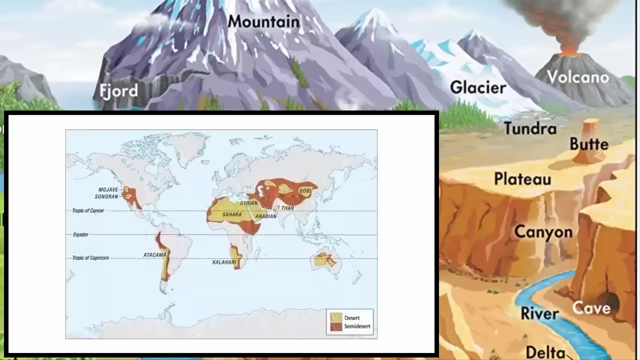 of tectonic plates. The next one is desert. When we think of desert, This kind of a sandy picture comes to our mind. right, But then that's not the only desert. There are basically four types of deserts. The first one is hot and dry desert, which exist in the subtropical region. 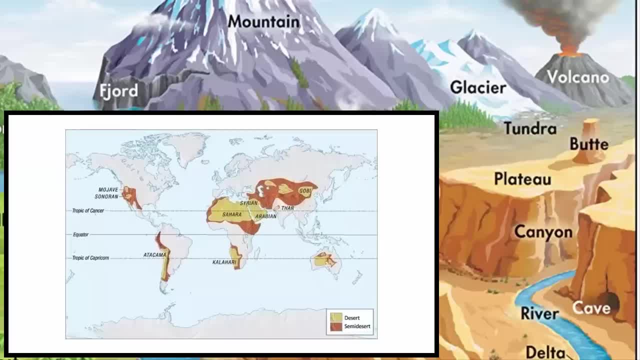 They are along the Tropic of Cancer and Tropic of Capricorn. At subtropical region it is due to pressure differences, and circulation patterns of air masses hinders the formation of clouds. That is why there is very little rainfall on the land, which eventually causes subtropical 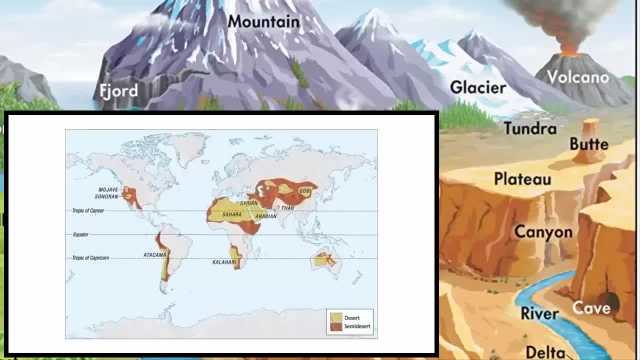 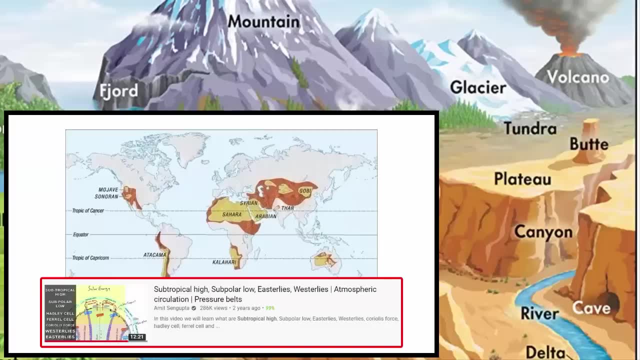 deserts. Basically, a subtropical region is a high-pressure zone. If you want to know why it is, then please watch this video. in this I have explained why subtropical region has high pressure. The link to this video will be there in the description. 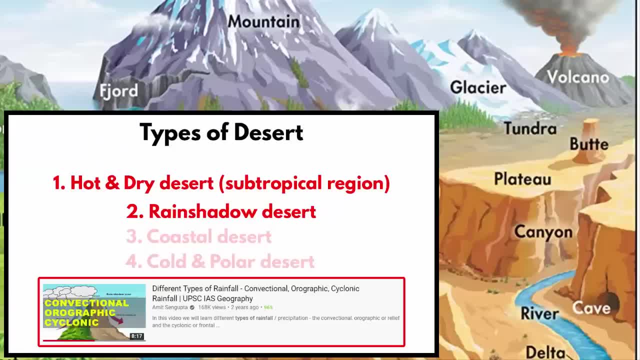 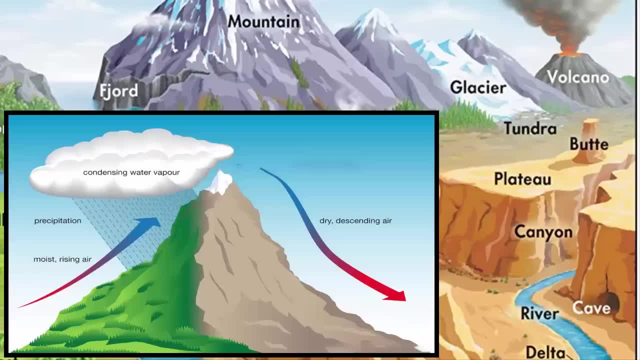 The second type of desert is 7. Rain shadow desert. I want you to watch a video where I have explained different types of rainfall. in that I have explained about aurographic rainfall. So there are two sides of a mountain. one is the Windward side and the other is a Leeward. 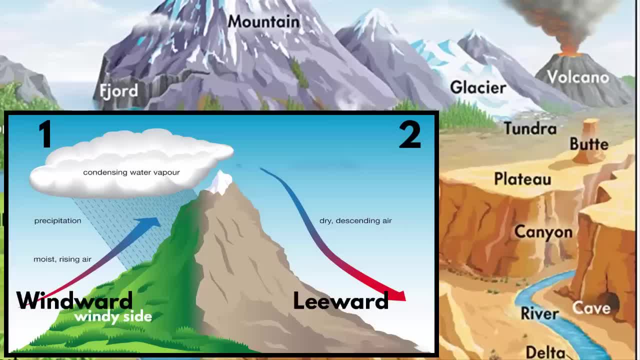 side the name. you can easily figure out that windward means the side of the mountain which faces a lot of wind. As a result, rainfall occurs. And leeward side is the opposite side, where it is dry and there is no wind. That means there is very little or no rainfall at all. 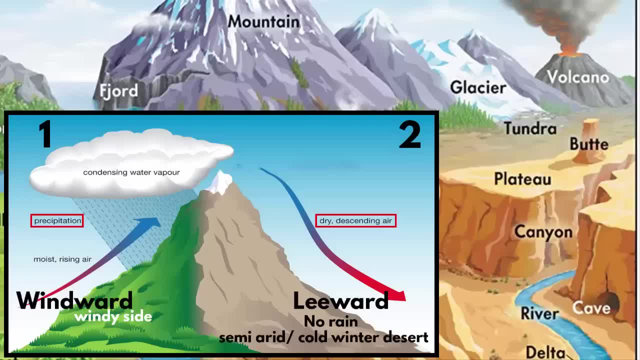 on the leeward side of a mountain. So these semi-arid and cold winter deserts are found on the leeward side of a mountain, which are also known as rain shadow deserts. When moisture hits a mountain range, it is forced to rise. As a result, the air cools and forms cloud. 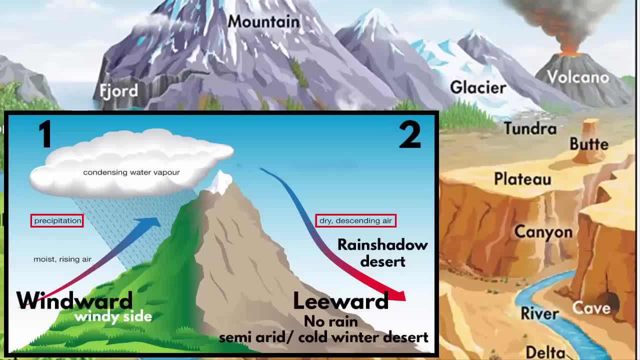 Because of that, it rains on the windward side of the mountain. After that, when the air moves over the mountain top and begins to descend on the other side, there is very little moisture left. That descending air warms up, making it difficult to form clouds. 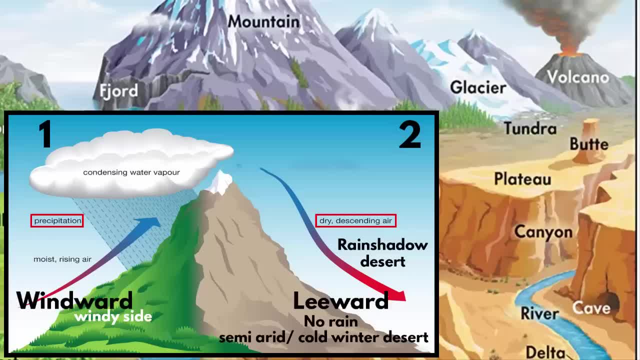 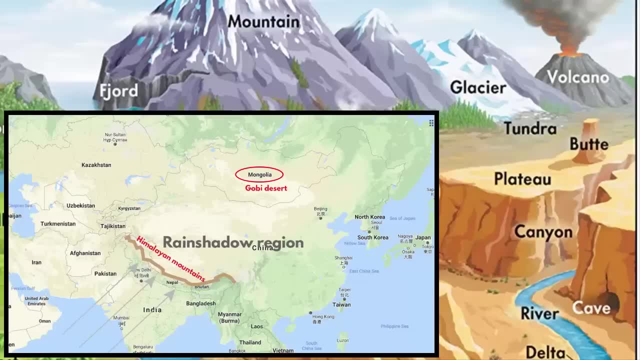 Hence there is no rain on the leeward side of the mountain, So the region on the leeward side of a mountain also becomes a desert. Some examples of rain shadow deserts are the following: Rain shadow deserts are Mongolia's Gobi Desert, the eastern part of Western Ghats, If you look. 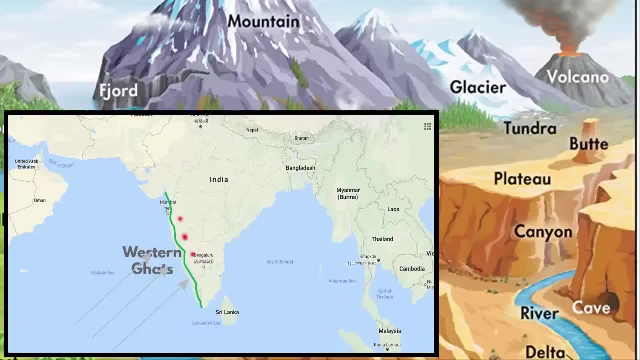 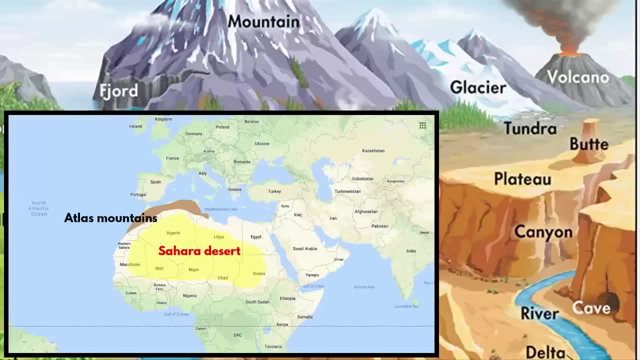 at the state of Karnataka, you will find many mini-deserts which are located on the eastern side of Western Ghats. Another example is the Sahara Desert, where the northern part of the African continent is covered with Atlas Mountains that blocks the wind from the Atlantic. 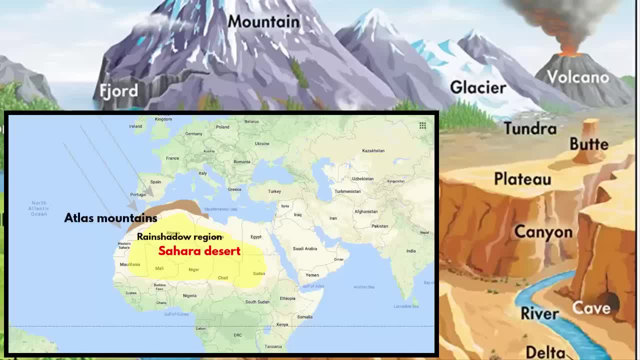 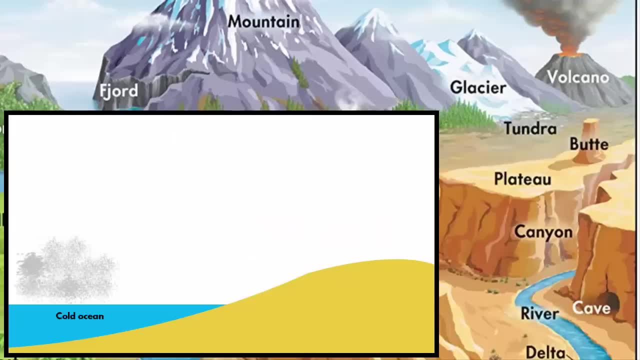 Ocean and the Mediterranean Sea, And that's what makes the Sahara Desert a rain shadow desert. The third type of desert is coastal deserts, When cold ocean currents blow towards the shore. these winds are cold because they are in contact with cold water And they produce a layer of fog which is a thick cloud of. 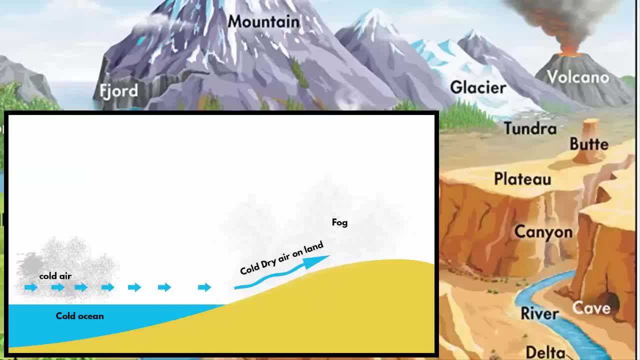 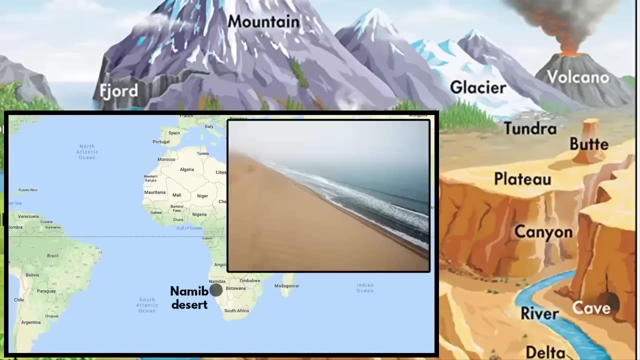 tiny water droplets that are too small to fall as rain. Now this heavy fog moves onto the land, but the sun's heat makes them disappear during the day. Since there is no rain, the coastal region turns into a desert. Some examples of coastal deserts includes the Namib desert in southwestern Africa and. 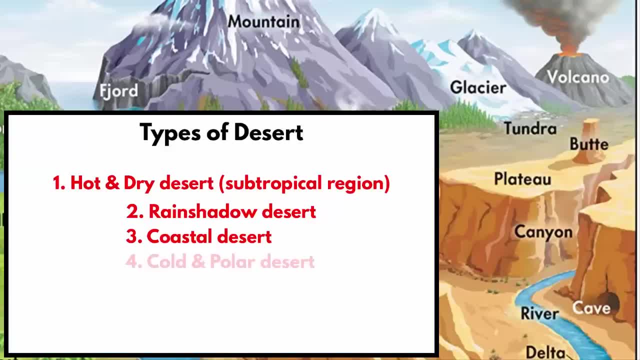 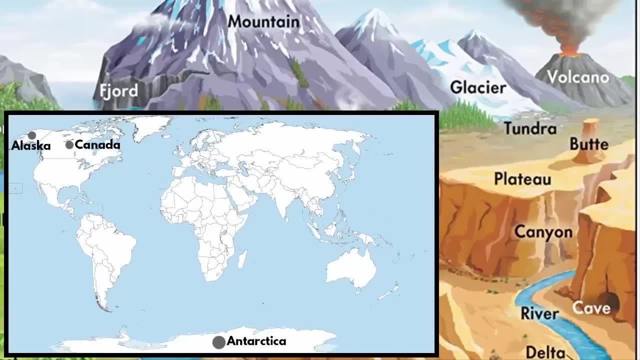 Atacama. desert in Chile. desert in Chile. The fourth type of desert is cold and polar desert. Examples of polar deserts are Antarctica, Alaska, Canada, Greenland, Iceland, Norway, Sweden, Finland, Russia. In India we have Ladakh, which is a cold desert. 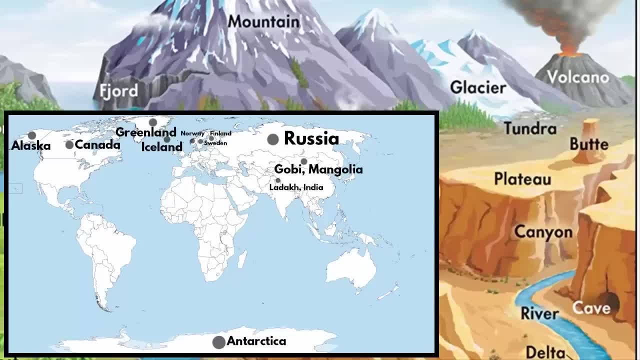 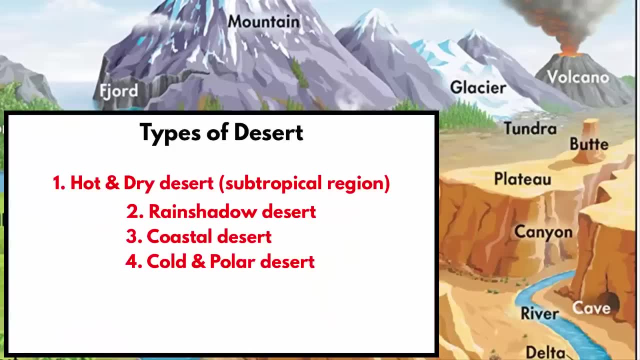 Even Mongolia's Gobi desert is a cold desert, But it is also a rain shadow desert. Patagonian desert in Argentina is also a cold desert. So the important point that you have to remember is that all these different types of deserts have one thing in common: 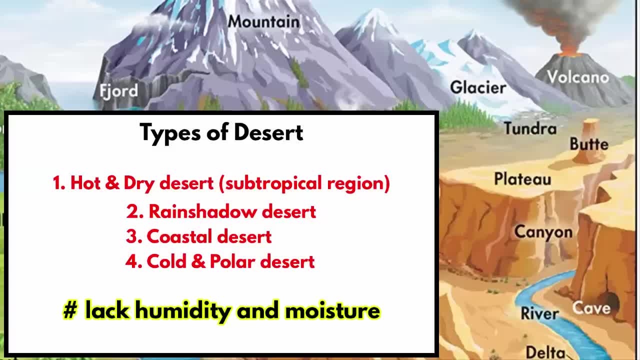 They lack humidity and moisture. When there is less of humidity or moisture, that's when there is a shortage of rain, And deserts are areas that receive very little precipitation. Now that you know what is a desert, in a desert, you will also find oasis. 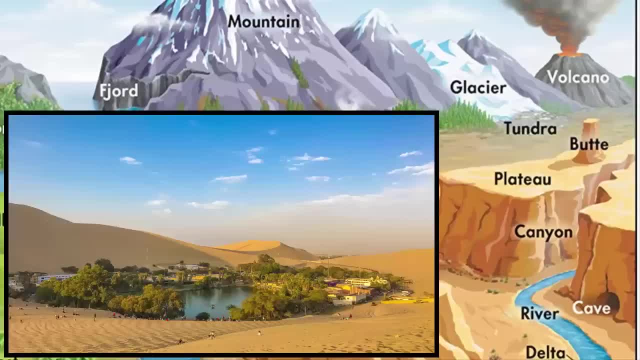 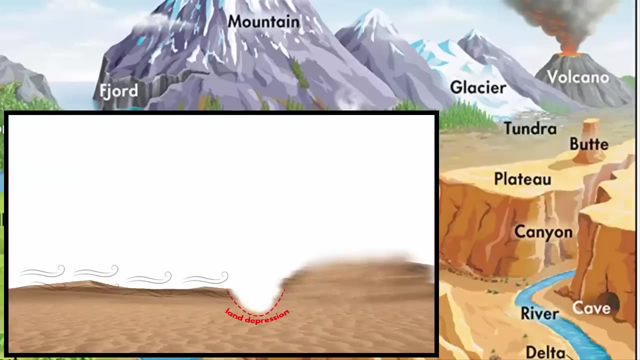 Oasis can be naturally formed or manmade, Basically in a desert. if you find a small region where there is water on the surface, it is called oasis In a desert. you will notice that the winds carry large amounts of sand In many areas of desert. this kind of natural action creates land depression. 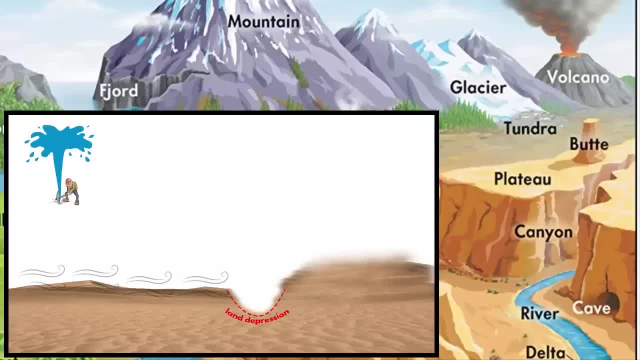 Water from the ground is basically obtained if you start digging the earth's surface. When it is manually done, it is called a manmade oasis, And when it occurs naturally, you know, due to wind, blowing, erosion or any kind of landslide which creates fault and that allows the water from the ground to reach the surface, 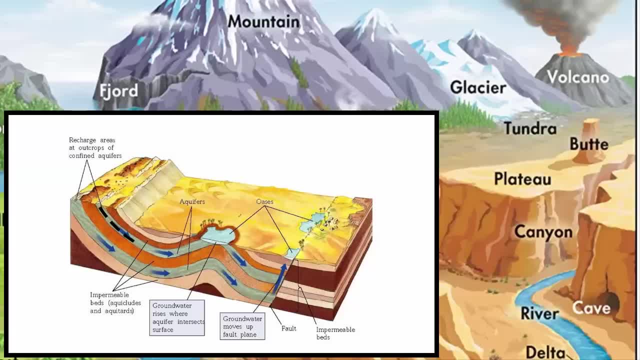 So what is a desert? If you look at this picture, you will see that the groundwater rises due to change in land elevation. If the groundwater is closer to the surface, then oasis are easier to form due to natural reasons like strong wind, blowing, erosion, landslide, etc. 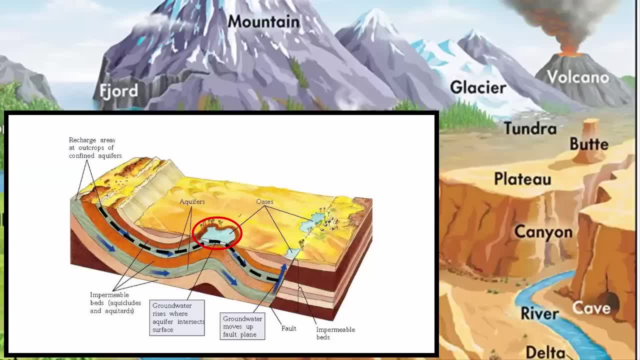 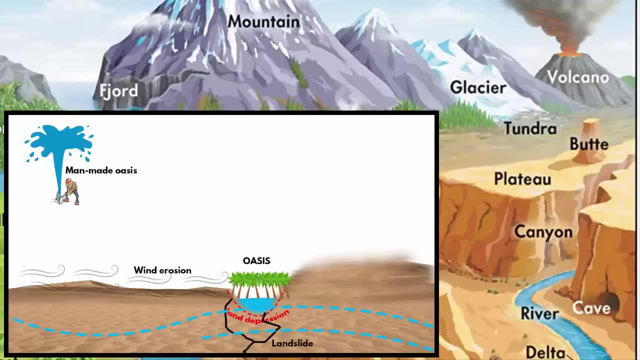 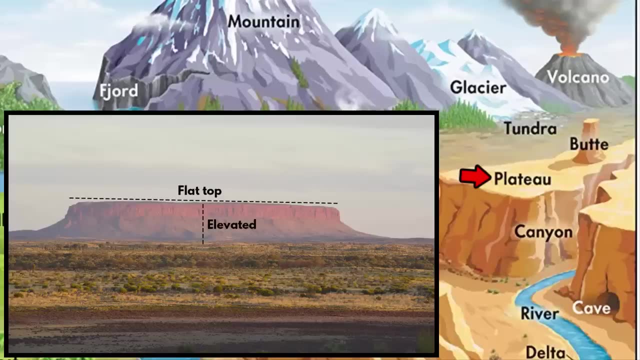 Because all it requires is to breach the upper thin layer of the ground that covers the layer that has water. Once it's done, the water comes out on the surface, and that is how an oasis is formed. The next one is plateau. A plateau is a flat, elevated piece of land that is higher to the surrounding land area. 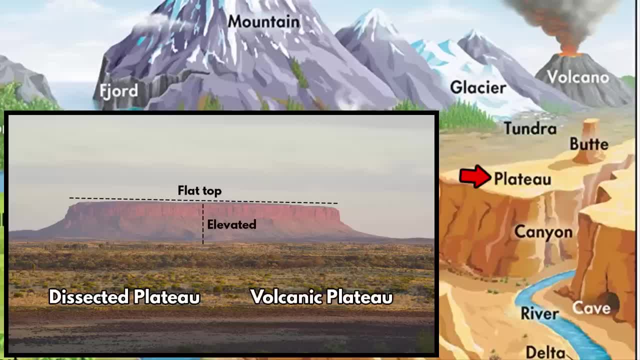 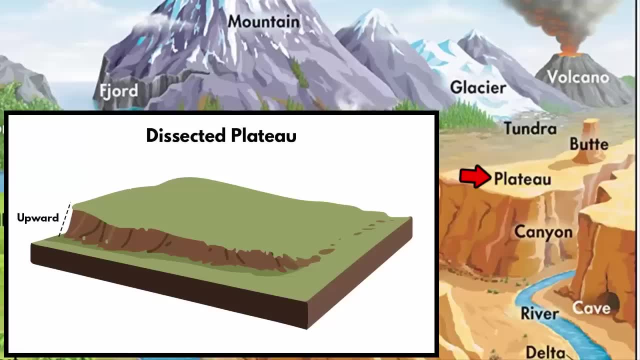 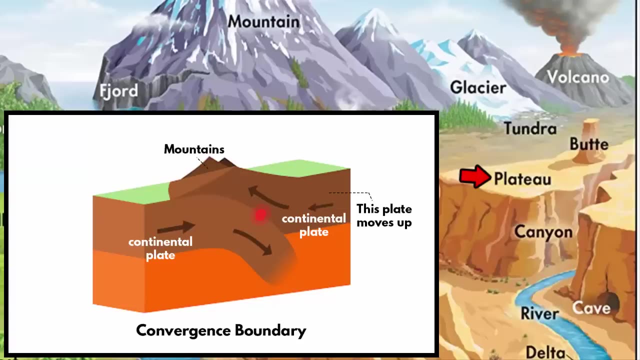 There are two kinds of plateau: dissected plateaus and volcanic plateaus. Dissected plateaus looks like this. These are formed due to upward movement in the earth's crust. One side of this plateau will have a slope, Basically when two continental plates collide. that is how mountains are formed, right. 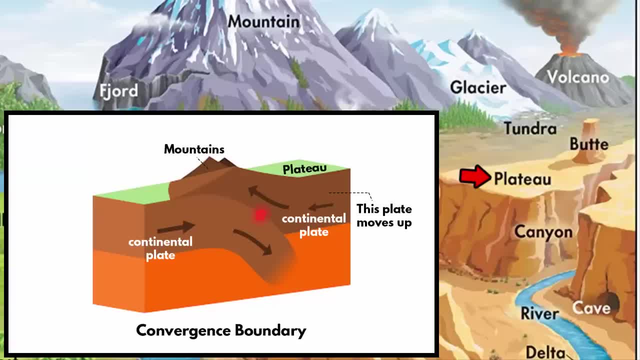 Even plateaus are like mountains, except it has a flat top. So even dissected plateaus are like mountains, except it has a flat top. So even dissected plateaus are like mountains, except it has a flat top. And so these two types of plateau are formed due to slow collision of tectonic plates. 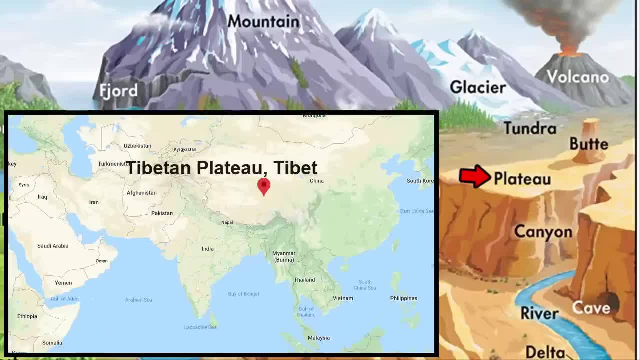 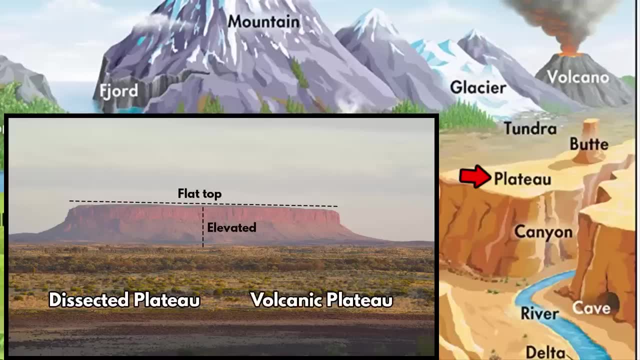 A good example is the Colorado plateau in US, then Tibetan plateau, then Mexican plateau in Mexico and Patagonia plateau in Argentina. And the second one is volcanic plateaus. They are formed by numerous small volcanic eruptions that slowly build up over time, forming 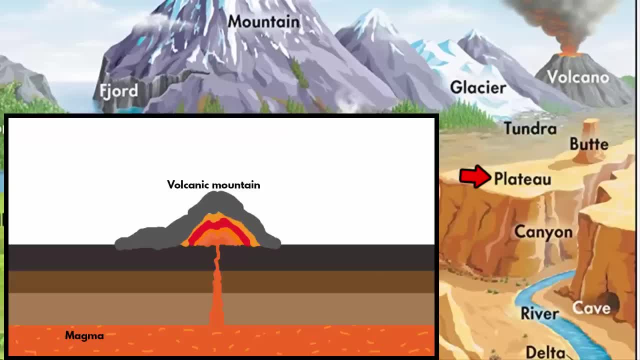 a plateau. Anyhow, a plateau is an elevated piece of land. When lava continuously comes out of a volcano, over time it accumulates in the form of layers, And that is also another way how plateaus are formed. Some examples of volcanic plateaus are: 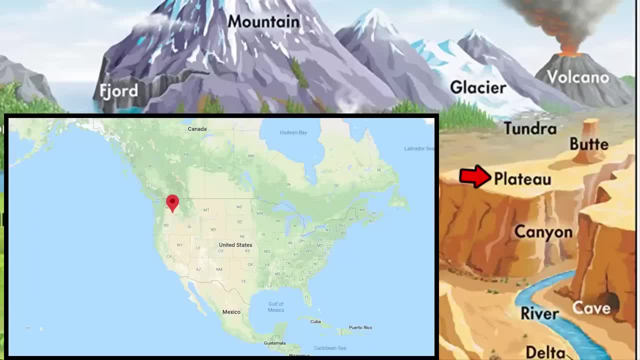 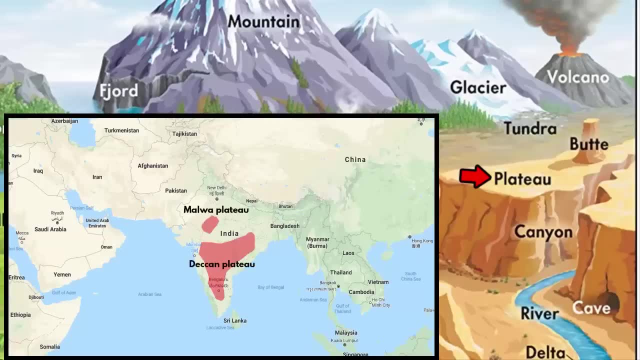 the Columbia Plateau in the northwestern United States of America, the Northern Islands of New Zealand. In India, Malwa Plateau and Deccan Plateau is of volcanic origin. Now, erosion and rivers can influence the shape of a plateau. Even in the oceans you will find plateaus. 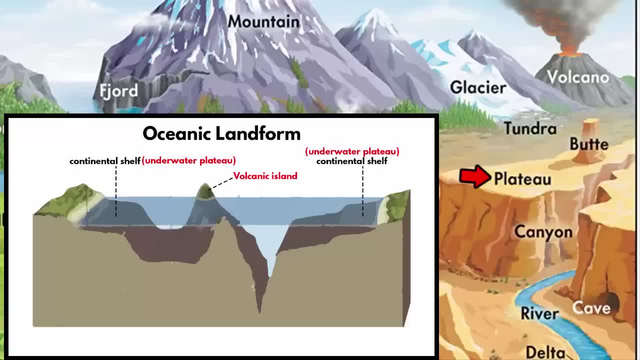 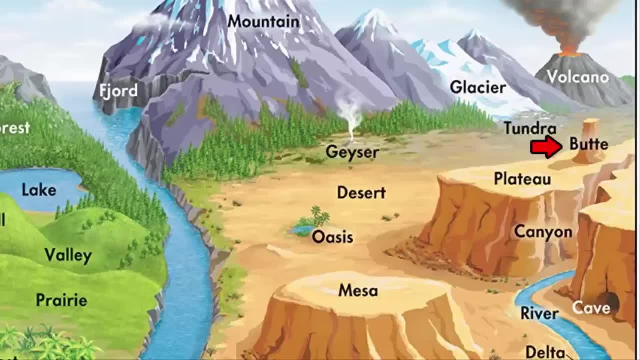 Ocean plateaus are of two types. One is made of continental crust and the other is made up of igneous rock due to solidification of lava. The next one is Butte. It is an isolated hill with sharp vertical sides and flat tops. 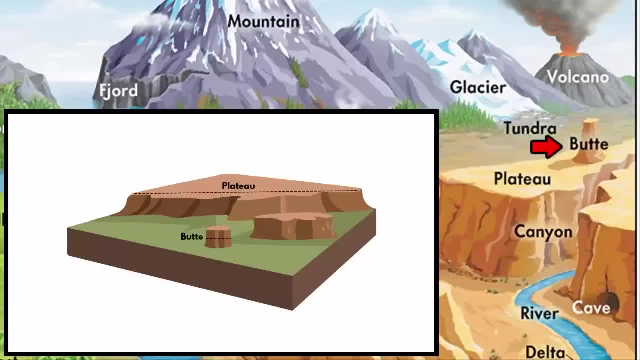 Buttes are smaller in size compared to a plateau. If you see, buttes are also plateaus But due to continuous erosion by water, rain and wind, they have turned into tall, flat-topped landform. Continuous flow of streams and wind activity. 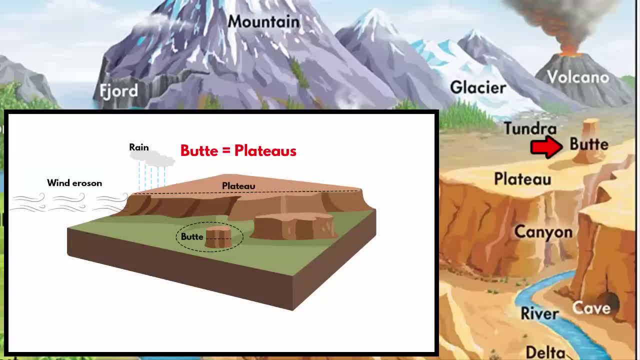 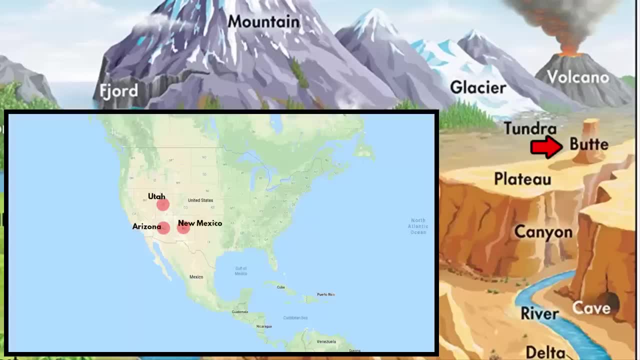 cuts a plateau in such a way that from a plateau it turns into a butte. They basically look like a tower And they are created by the flow of water. They are created by erosion and weathering. Buttes are found in Mexico and the southwestern side of the United States. 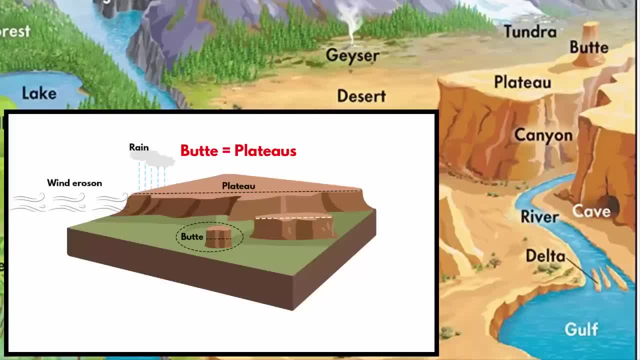 The next one is Mesa. Now, Mesa is also a plateau, basically an isolated, flat-top elevated landform, But the only difference between a Mesa and a plateau is that Mesa is formed after weathering and erosion of a plateau. If I have to put it in an order, 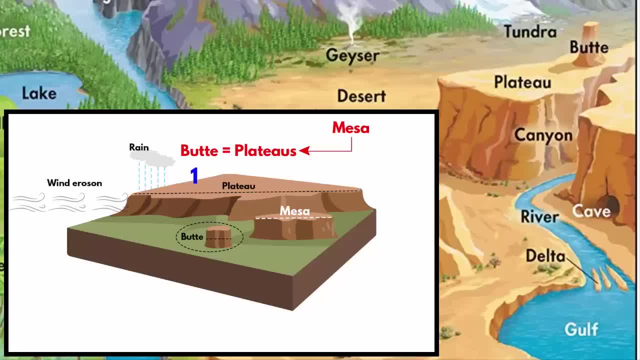 first comes a plateau. after weathering and erosion, a plateau gets converted into a Mesa and after that, more and more weathering and erosion, a Mesa gets converted into a butte. Weathering and erosion basically cuts the rock in a plateau and turns them into Mesa and Butte. 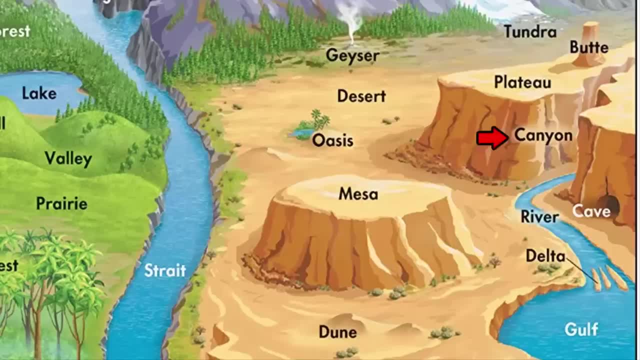 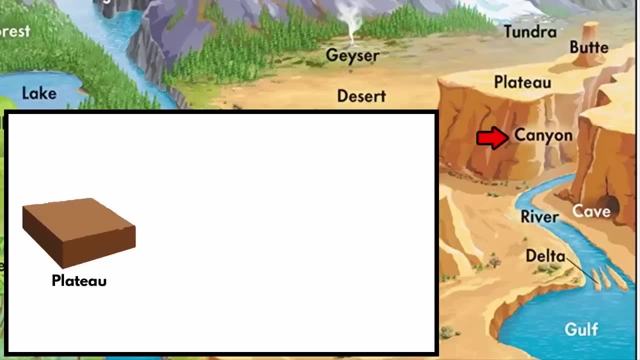 Now let's see what is a canyon. First I want you to imagine a large plateau. I have already explained how plateaus are formed, So imagine a large plateau. Now try to carve this plateau with the help of rivers and glaciers. So, basically, with time. 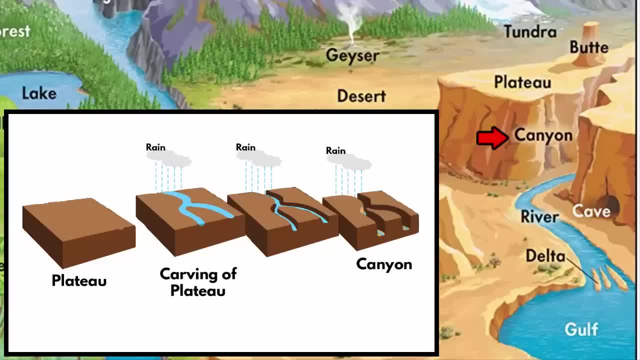 the river erodes the bedrock of a plateau By cutting deep channels in the bedrock. Continuous flow of rivers and wind activity carves out a steep valley walls to form a canyon, And this kind of process takes many, many years. So that's how canyons are formed. 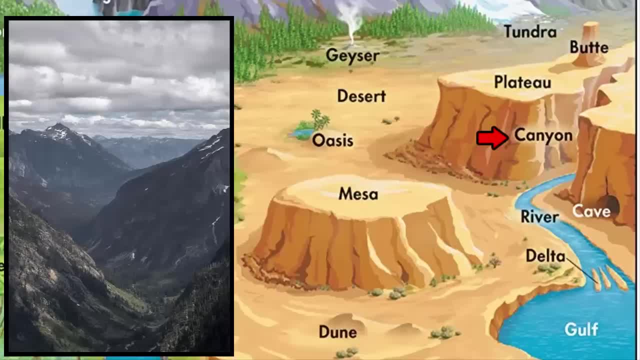 By the way, canyons are formed not only by cutting a plateau. It also happens with mountains. That is how valleys are created. In a way, valleys are also like canyons. Both of them are formed through erosion, that is, continuous wearing down of the land. 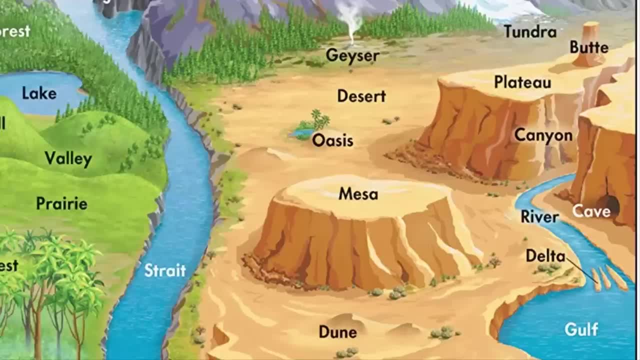 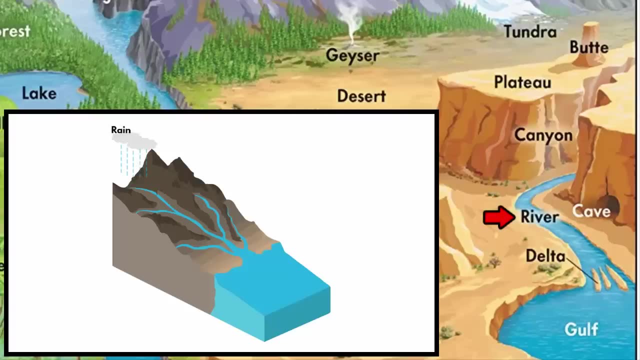 by wind and wind. Now we will see how rivers are formed. Rivers are basically water that moves from high elevation land to lower elevation land with the help of gravity. The water on the higher elevation land can come both from rain as well as melting of snow. 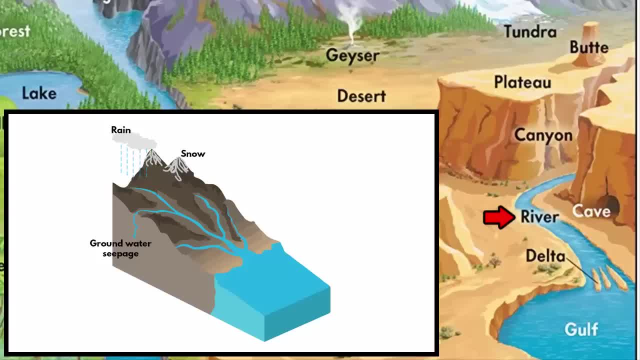 After that, the water either gets absorbed into the ground or starts to flow where there is land depression. This kind of a downhill flow turns the water into a river and lake. Rivers eventually end up flowing into a sea or in the ocean. Along the way, it causes massive erosion. 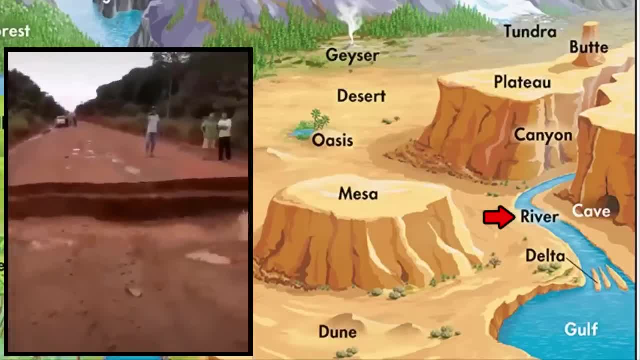 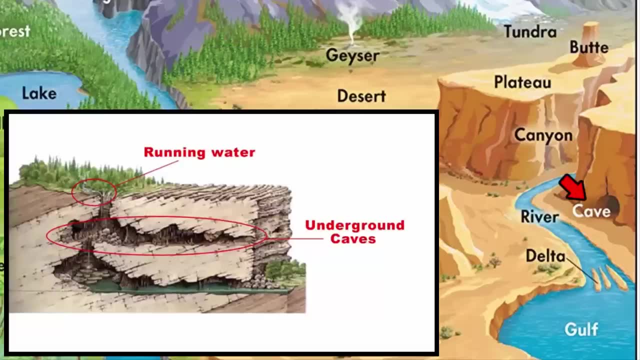 and weathering of the soil, rock and sediment, Which in turn changes and alters the face of a landscape. The next one is cave. Caves are formed by the dissolution of bedrock. Rainwater reacts with carbon dioxide from the air and, as it penetrates through the soil, 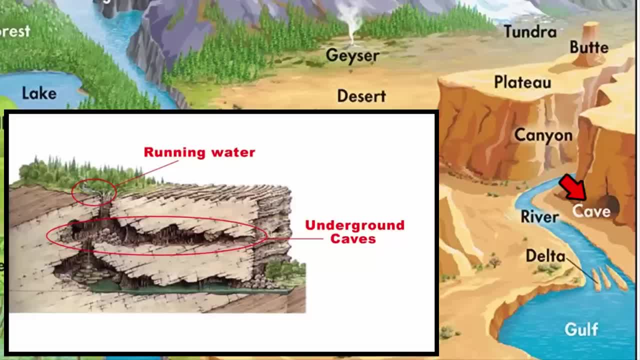 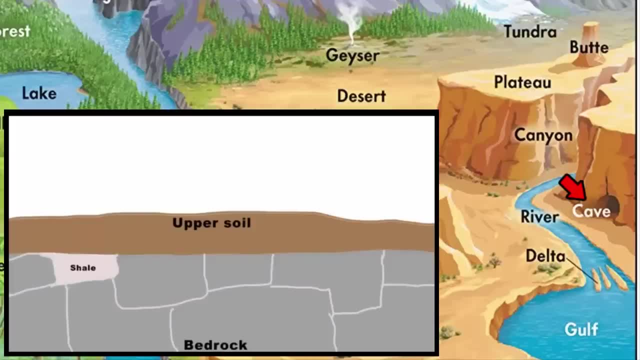 the rainwater turns into a weak acid. Now this slowly dissolves the bedrock. A bedrock consists of alternative rocks. Somewhere you will find shale rock and then somewhere you will find sandstone. Then, in between these two, you will find limestone or dolomite. 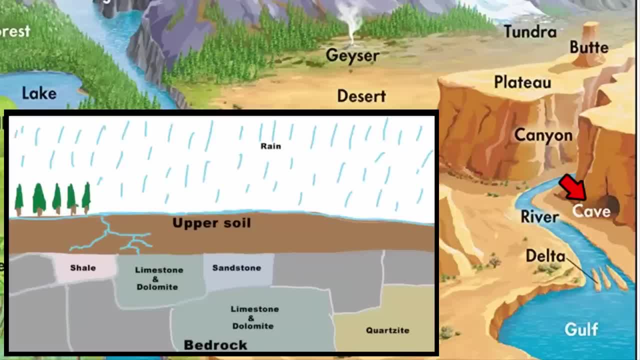 When rainwater penetrates to the soil, it turns into a weak acid and it starts dissolving the bedrock by reacting with rocks like dolomite and limestone. As a result, long, hollow underground caves are formed. The height of these underground caves depends on how thick the bedrock is. 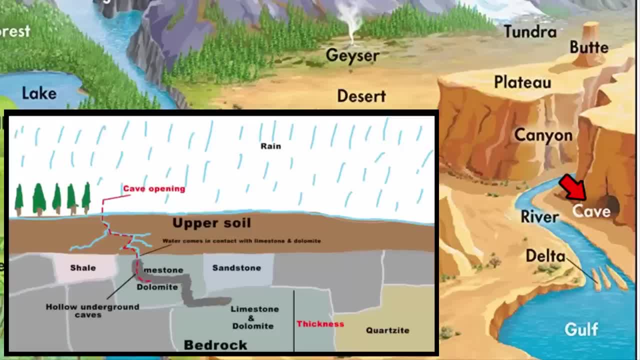 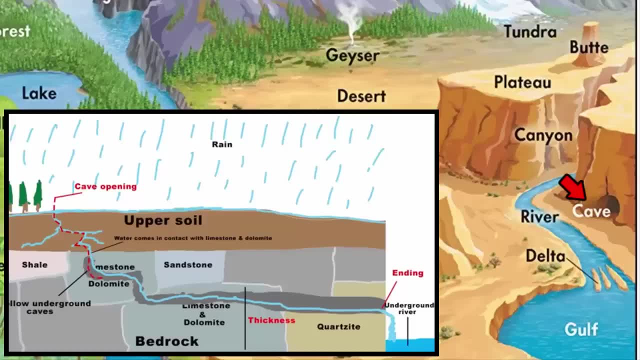 So every cave has an opening through which water enters. Similarly, there is also an end from where the water goes out, But there are many caves that do not have an end, Because they may be still in their middle age, where the water has not eroded the rock enough. 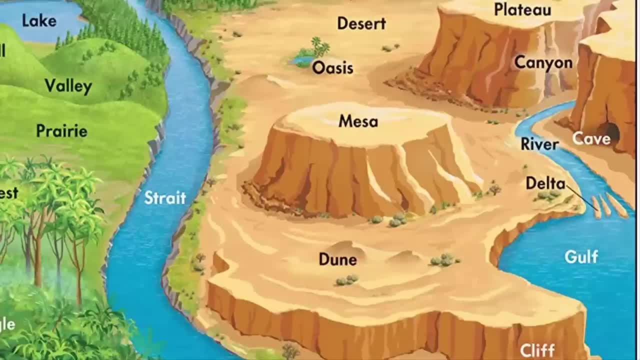 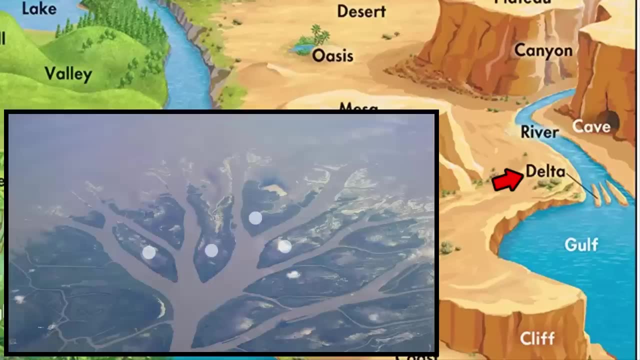 to create a complete tunnel. The next one is delta. Now this is called river delta. These are landforms created by deposition of sediment that is carried by a river. We know that when rivers flow, it carries a lot of sediments and rocks. 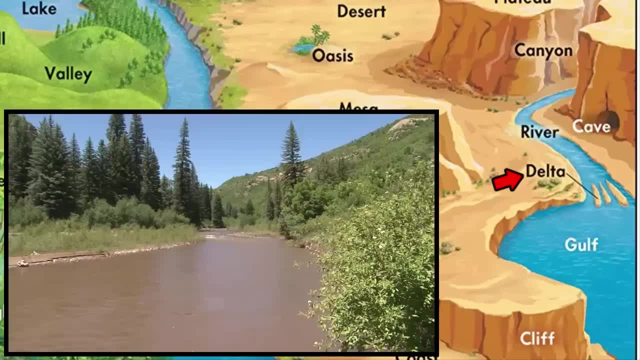 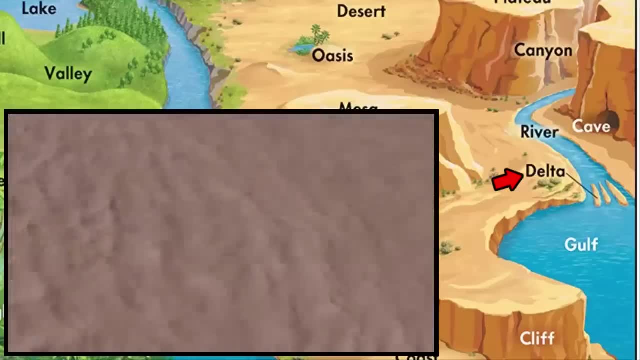 The greater the flow, the more sediment it will carry. As soon as the flow of the river slows down, sediments in rivers get deposited. You will notice that large, heavier particles like pebbles, rocks and sand are deposited first. After that, lighter material like 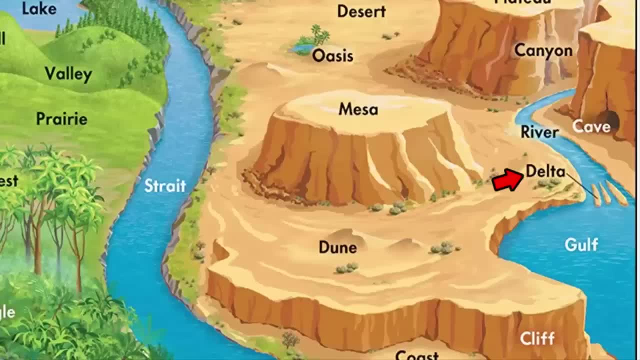 silt and clay gets deposited. So what I am trying to say is that you will find these deltas where the speed of the river is slow. When river starts to move slowly, that is when the sediment gets accumulated. Deltas usually occur where rivers enter an ocean. 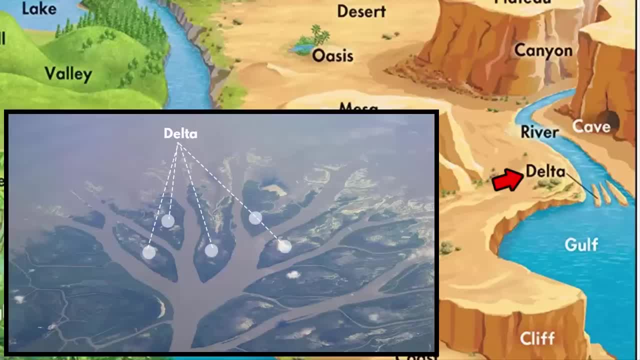 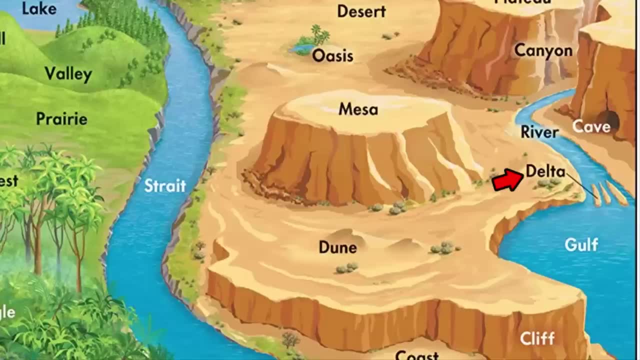 sea, estuary, lake reservoir, etc. Apart from these places, you will find deltas at places where the river moves slowly. That's all you have to remember. In India, you will find deltas at all those places where major rivers meets the Bay of Bengal. 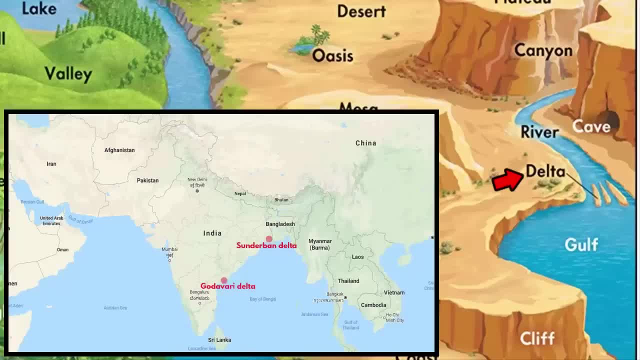 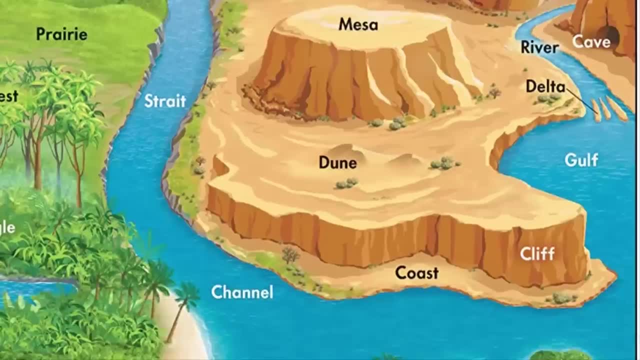 For example, the Sundarban Delta, Godavari River Delta, Kaveri River Delta, Mahanadi River Delta, Krishna River Delta and Bhitarnika Delta. The next one is Gulf. A gulf is a large inlet from the ocean into the landmass. 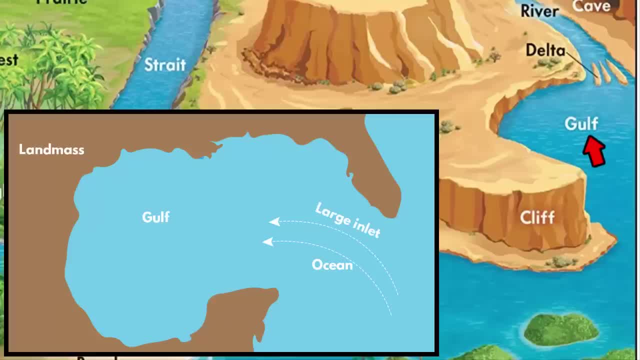 Basically, the shape of the landmass is such that some part of the ocean water forms an inlet. Now, this kind of landforms are purely natural and they are formed by the movement in Earth's crust. Whenever we talk about movement in the Earth's crust, 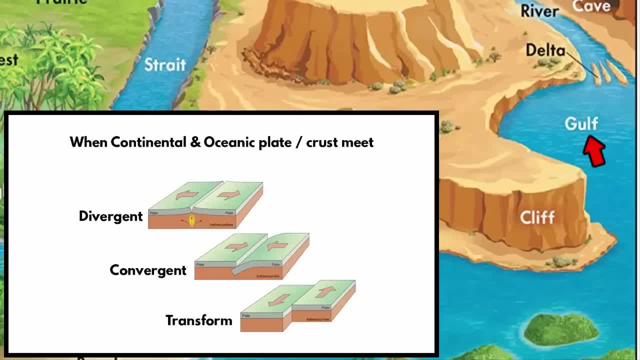 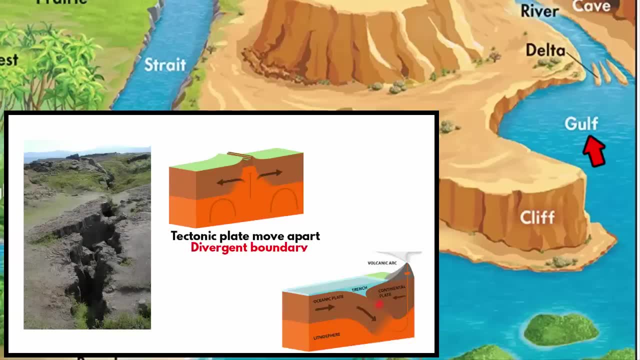 automatically remember those three types of plate boundaries: Convergence, Divergence and Transform. When Earth's tectonic plates crack or break apart, or when one plate goes under another, these are the ways how a gulf is formed. You must have heard many times that. 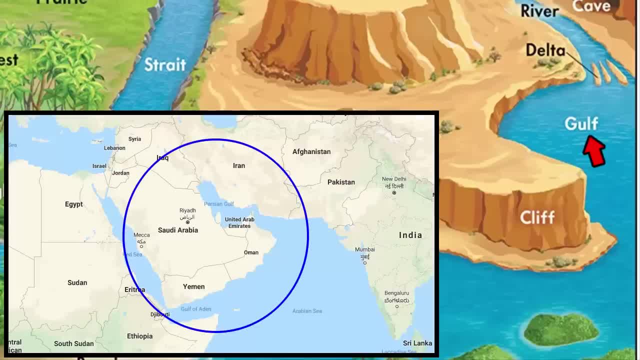 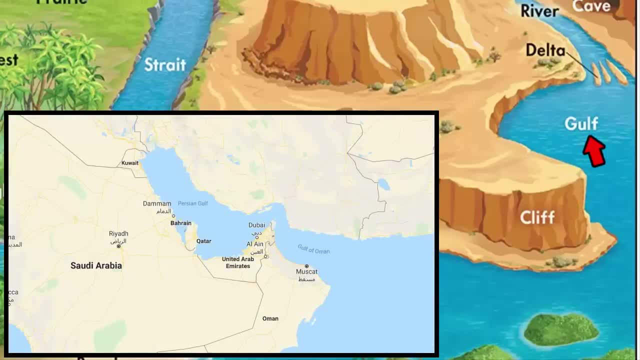 when people go to countries like Saudi Arabia, UAE, Qatar, they call these countries as gulf countries, And the reason these countries are called gulf countries is because they are located around the Persian Gulf, So Persian Gulf is a water inlet. Here the water is. 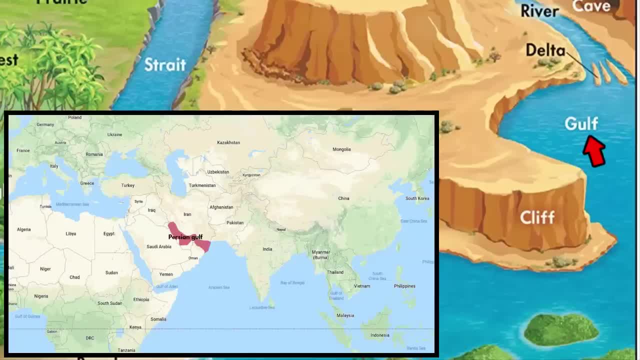 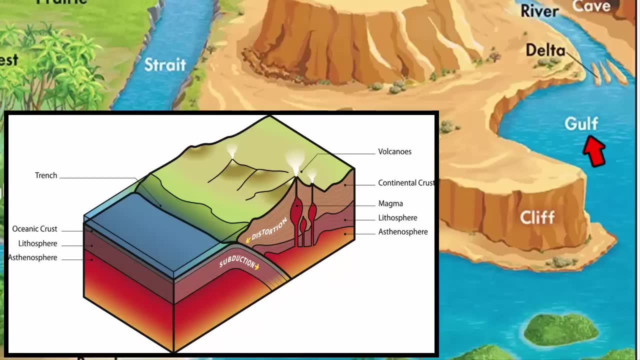 part of the Indian Ocean. The Persian Gulf was formed due to the subduction of the Arabian plate under the Eurasian plate, And subduction means the downward movement of the plate into the mantle beneath another plate. In India, the Gulf of Kutch. 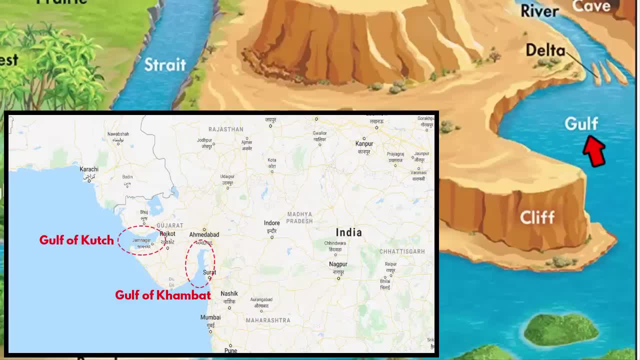 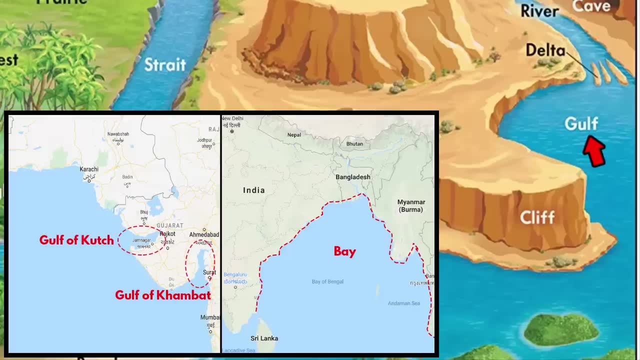 and Gulf of Khambhat are the two famous inlet of the Arabian Sea along the west coast of India, in the state of Gujarat. Another important point to remember is that both a gulf and a bay are the same things. The only difference is in the size A gulf is. 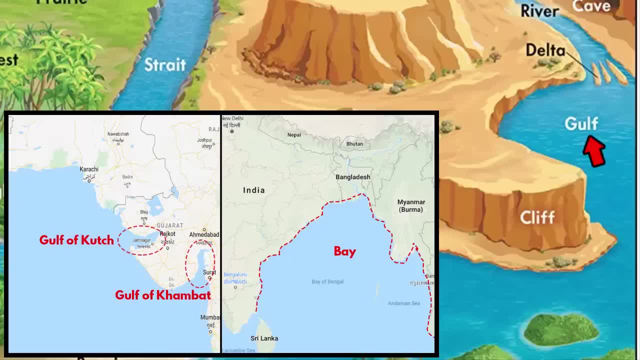 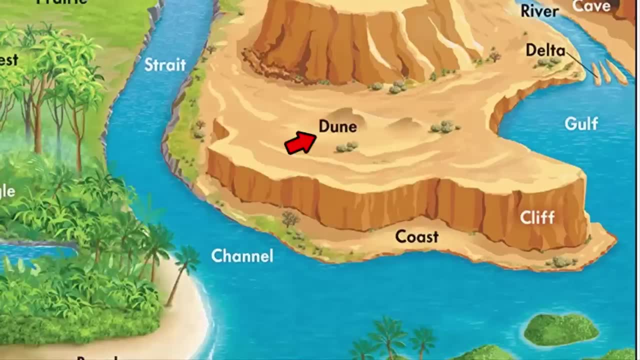 much larger than a bay, And their way of formation is also different. I'll tell you how a bay is formed when we reach that topic. The next one is sand dune. You will find them in deserts and beach By looking at the. 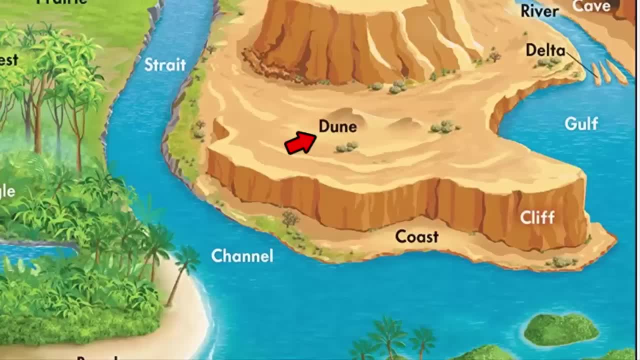 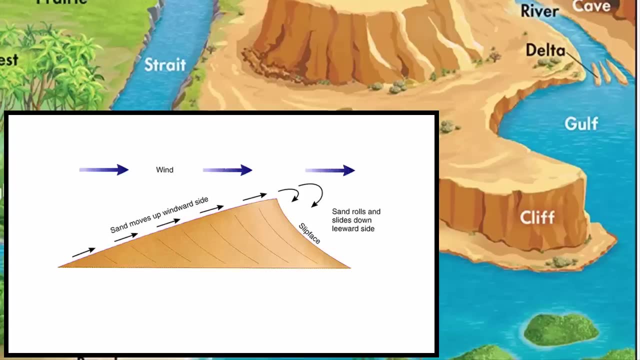 shape. you can easily figure out that they are formed by the wind. When wind blows sand, it gets accumulated at one place and forms a pile or stack of sand. This is what is called as dunes. Every dune has a windward side and a slip face. 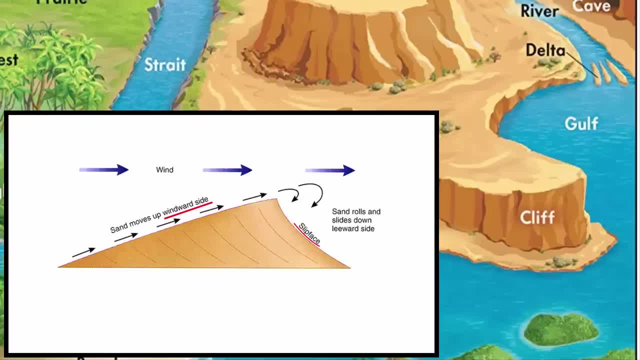 Windward side is the side where the wind is blowing and pushing material up. A dunes slip face is simply the side without wind. A slip face is usually smoother than a dunes windward side. The next one is cliff. If you look at a cliff, 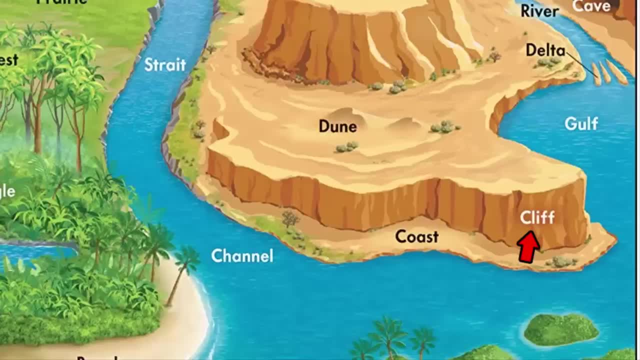 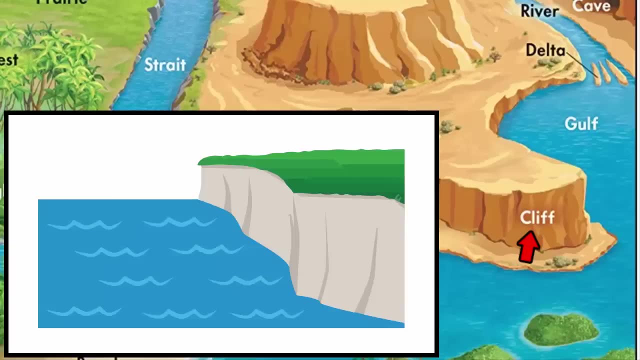 they are vertical and exposed rock, Basically an elevated piece of land form, And they are found near coastal region and river bed. The major sedimentary rocks that form a cliff are dolomite, sandstone and limestone. Even they are formed how mountains and plateaus are formed, That is. 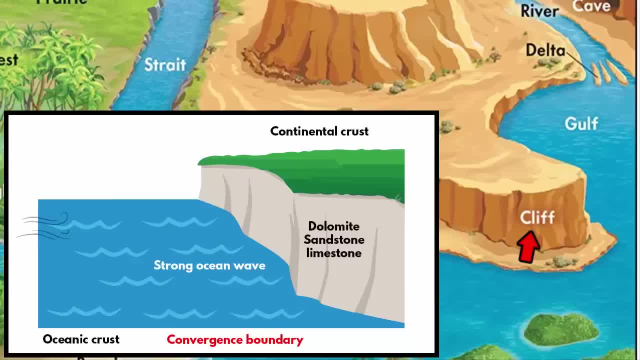 through tectonic activity. Now these rocks get hit by constant wind and water. As a result, they get eroded and weathered. The force of the water wave continuously hits the cliff On top of it. the water is salt water. 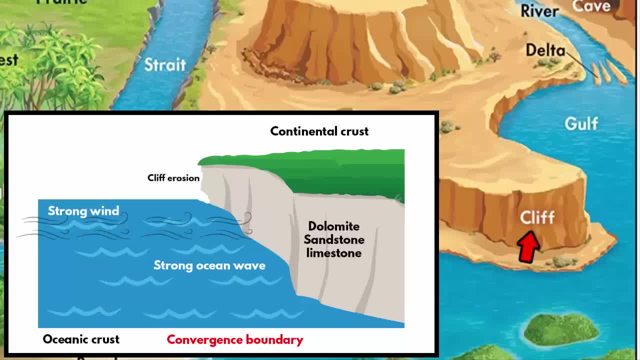 It dissolves the rocks easily. Then strong wind hits the cliff and erodes the rock particles slowly. The bottom portion of the cliff faces maximum erosion due to continuous hit by the sea and ocean waves. This creates a dent in the lower portion of the cliff, which is called a wave. 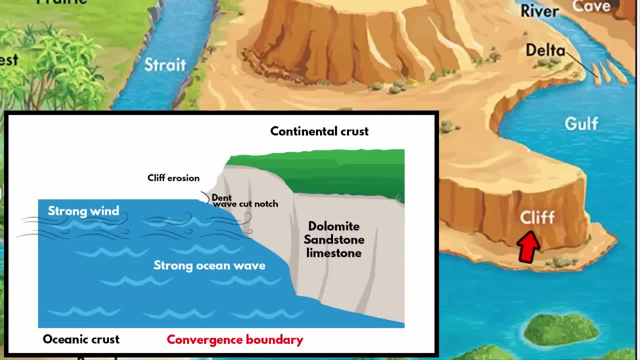 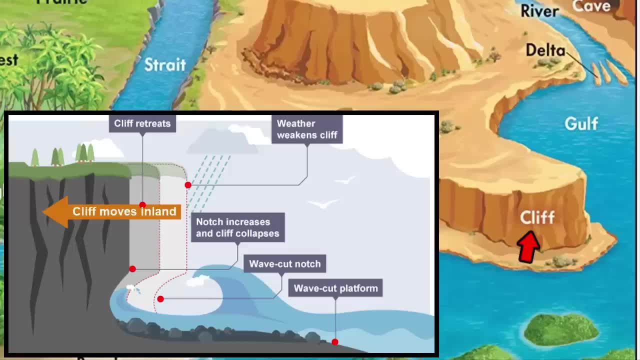 cut notch. As the notch increases in size, the cliff becomes unstable and collapses and gets washed into the sea. This continuous process will make the cliff collapse and move the entire cliff further and further inland, leaving behind a wave cut platform. When there is low tide, you will be able to. 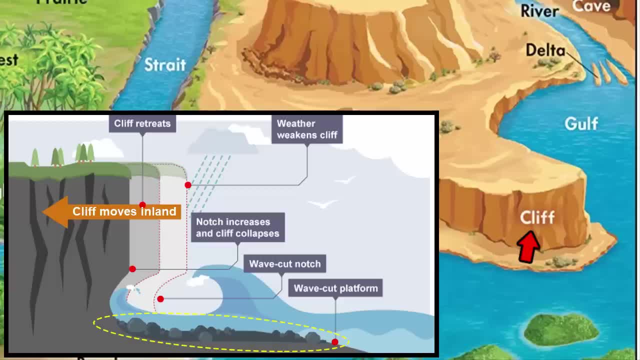 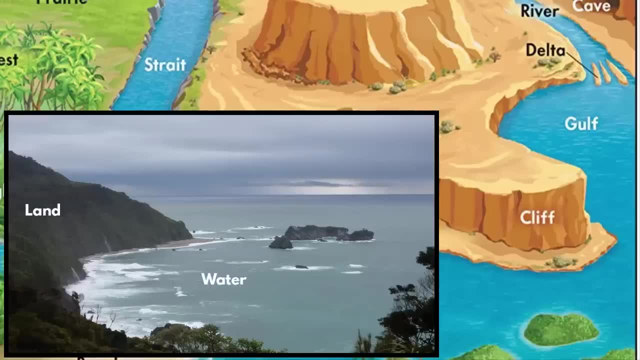 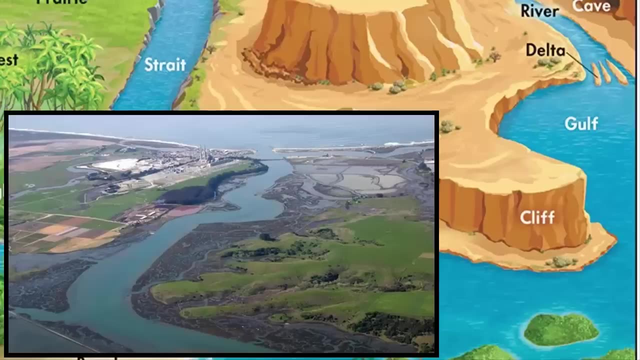 see the wave cut platform, And during high tide this area is submerged. The next one is coast. It is a boundary where land meets water. It is also called coastline. Waves, tides and currents help create coastlines, Even rivers, when. 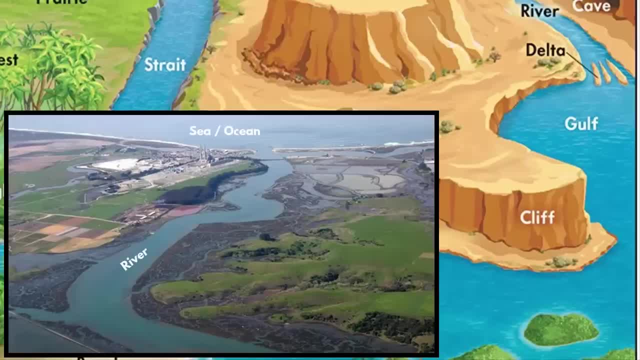 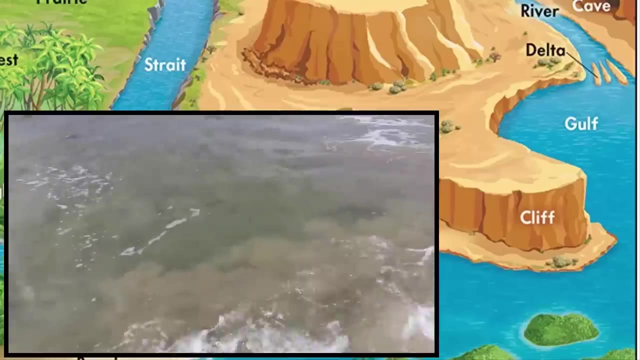 they meet. the sea or ocean. rivers bring large amount of sediment that gets deposited near the mouth of a sea or ocean, where it naturally forms deltas, beaches, dunes and barrier islands. When waves crash onto shore, they erode the land and take away large amount of sediment back. 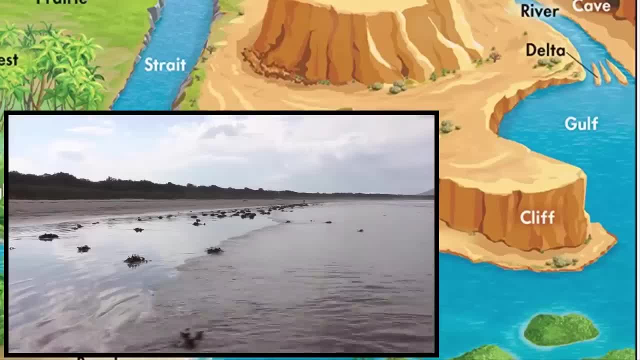 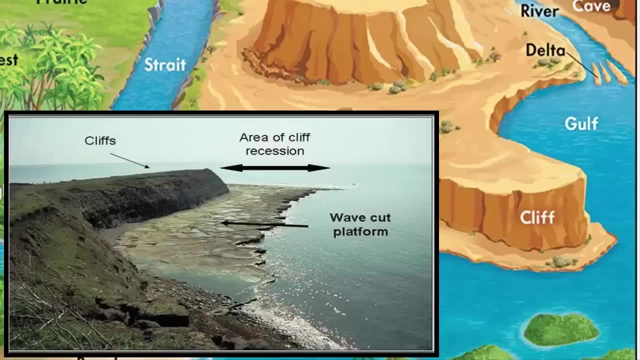 into the sea or ocean, leaving behind shells, seaweeds, etc. Now, depending on what kind of land it is- for example, if it is a hard granite land, then it is harder to erode. Just now we saw that at the bottom of. 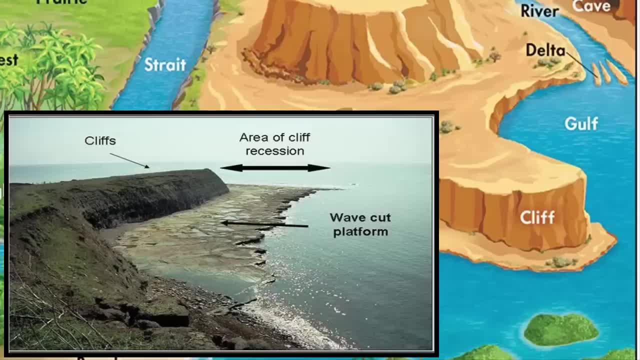 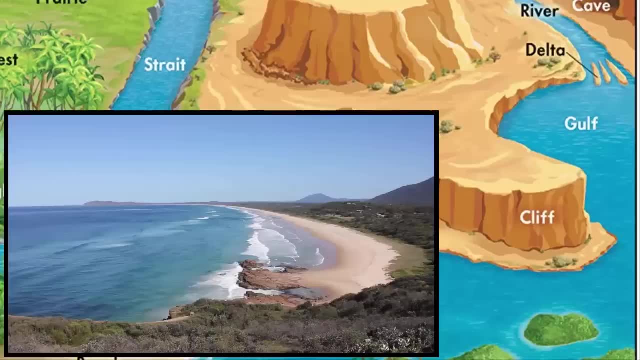 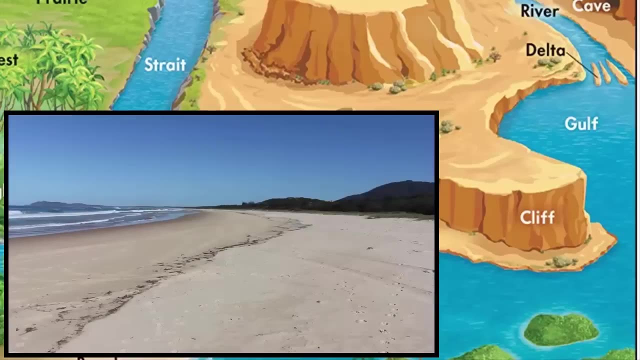 cliffs you will find rock hard surface, which is also called wave cut platform. A granite coastline takes hundreds of years to erode, But the sandy coastlines, on the other hand, change almost daily. The water slowly rises up over the shore and then slowly falls back again. 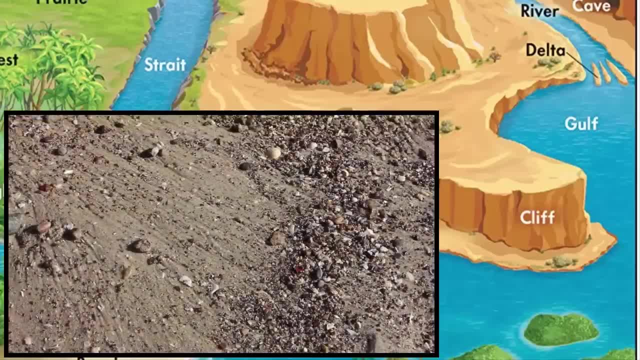 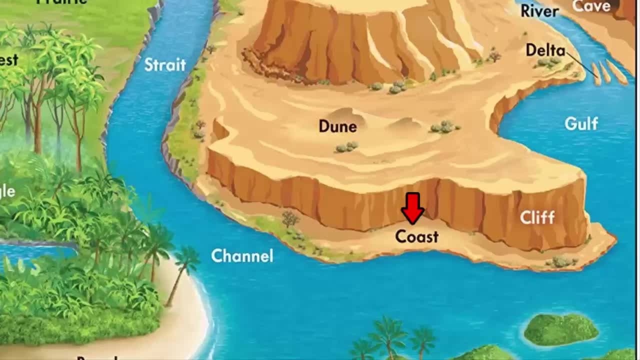 leaving material behind and taking away large volume of sand Again. big waves have lot of energy and small waves have less energy. So based on the size of the wave and the land material, the coastal landform varies. The next one is Strait. 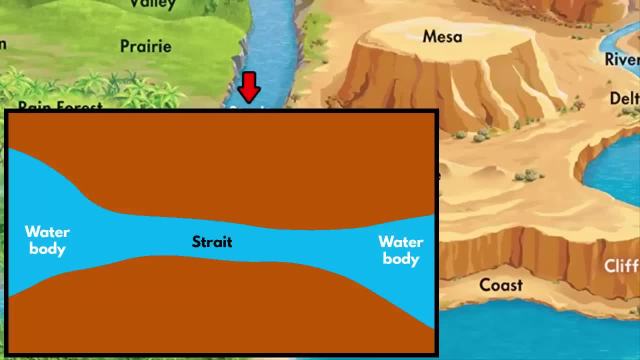 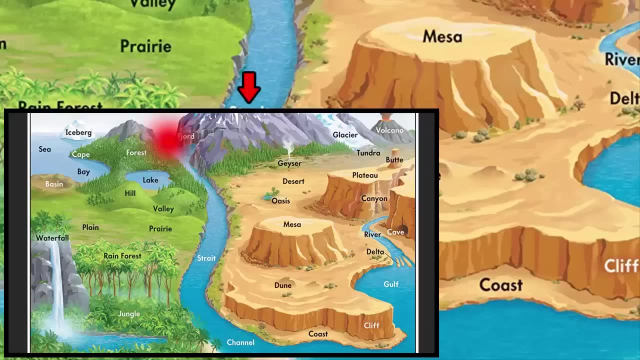 A strait is a narrow body of water that connects two larger bodies of water. In this picture you can see that a strait is connecting two large bodies of water. One is here and the other one is here. There are three ways by which a 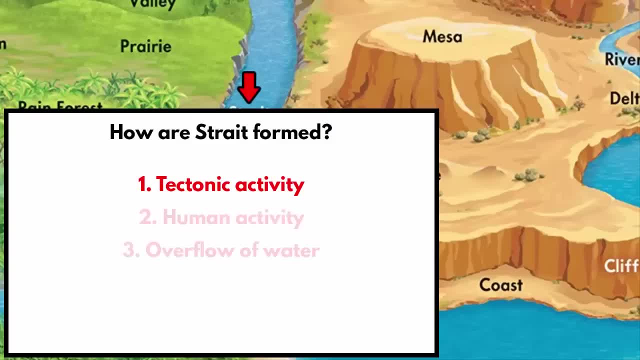 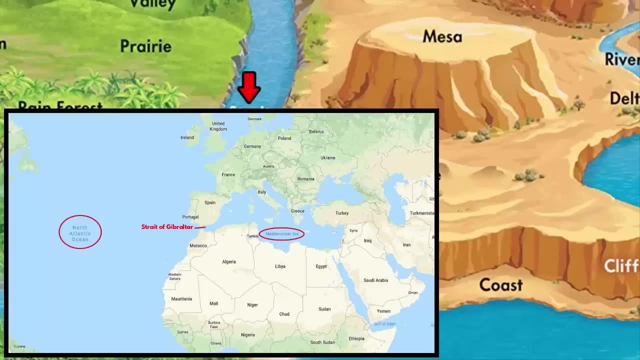 strait can be formed. Tectonic activity can be one reason. If you look at the strait of Gibraltar, it is the only link between the Mediterranean Sea and the Atlantic Ocean. It was formed by tectonic activity between the Eurasian and African plate. 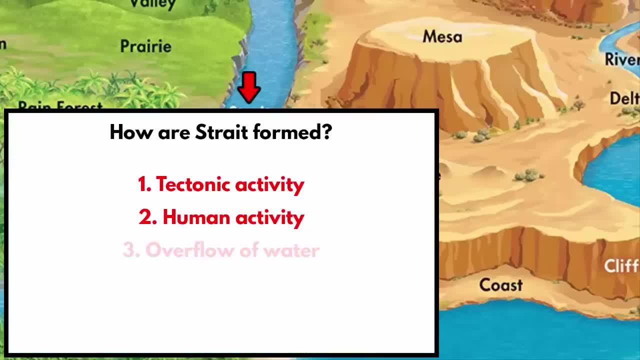 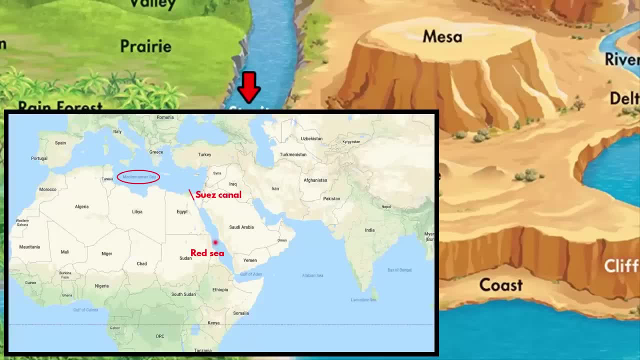 when they drifted apart. Another way a strait can be formed is by human activity. If it is done by humans, then we also call them canals. The Swiss canal is a good example. It connects the Mediterranean Sea and the Red Sea. 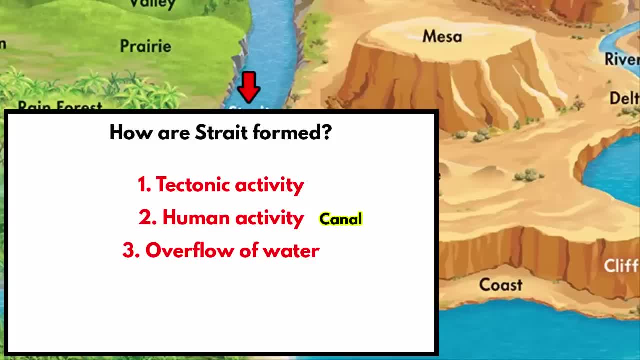 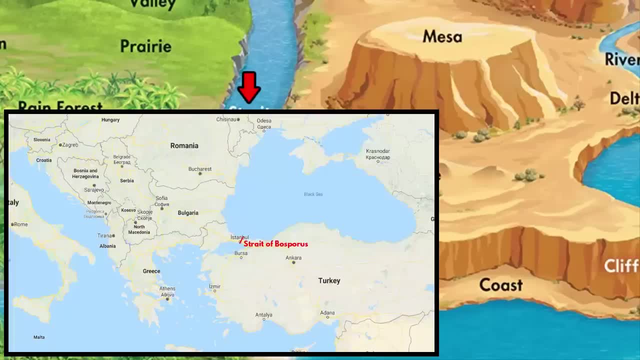 And the third way by which a strait can be formed is when a body of water overflows on the land and completely erodes the land and drowns it. If you look at the strait of Bosporus, it links the Black Sea and the Aegean Sea. 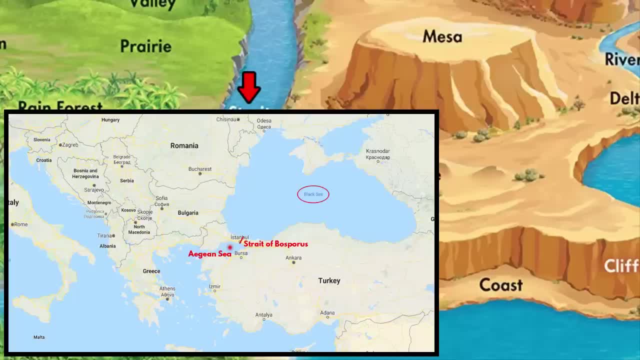 The strait of Bosporus is an extremely important strait separating the continents of Europe and Asia. So this strait was formed when the land at the southwestern edge of the Black Sea eroded and crumbled, creating a strait. In India we have the Park Strait. 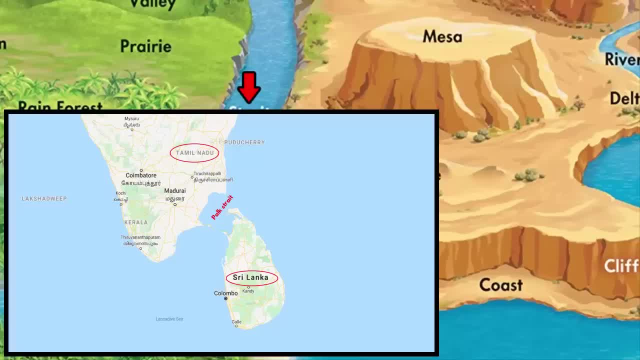 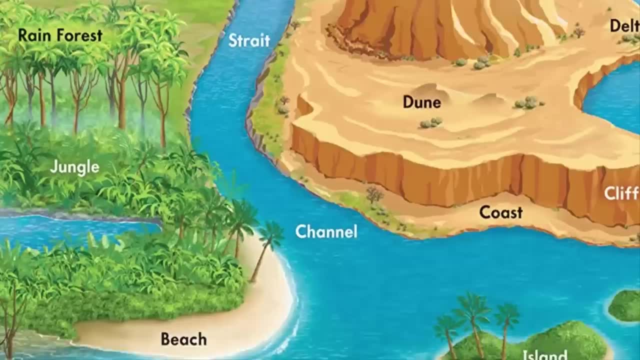 which is between the Indian state of Tamil Nadu and the island nation of Sri Lanka. It connects the Bay of Bengal in the northeast with Park Bay in the southwest. The next one is channel. A channel is a wider waterway that passes between two neighboring. 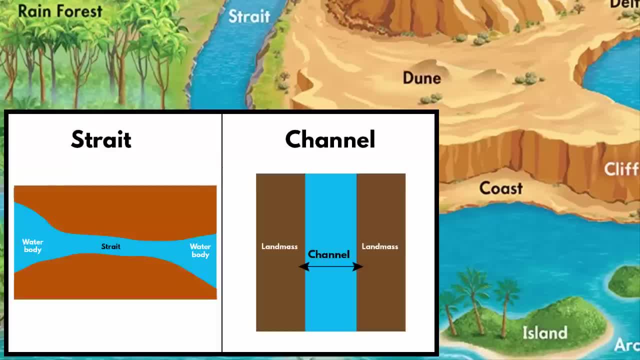 landmasses. Now, if you look at the difference between a strait and a channel, a strait is a narrow waterway that connects two larger bodies of water, While a channel is a wide waterway that passes between two neighboring landmasses. 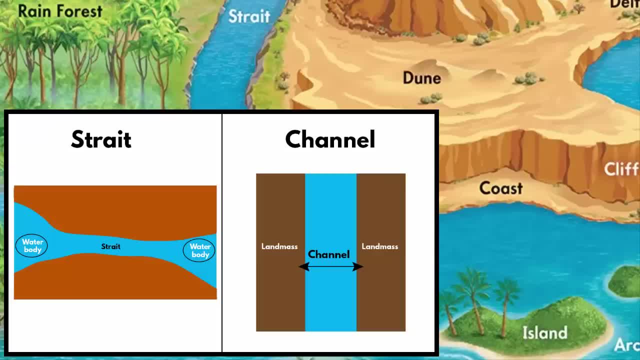 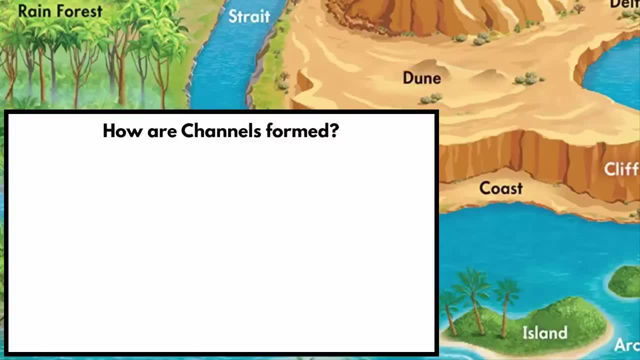 One connects two waterbodies and the other creates a gap between two landmasses. Around the world, you will find both small as well as big channels. That means channels are created both naturally as well as by humans. Natural processes include tectonic. 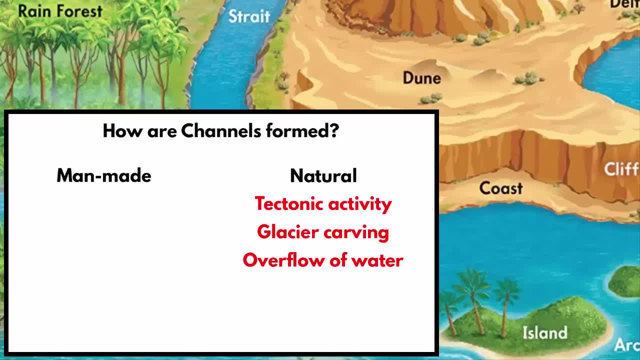 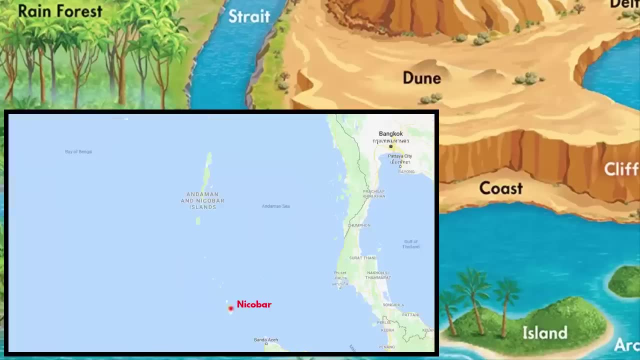 activity: carving of landmass due to glaciers and overflowing of water bodies. Manmade processes include digging up the land so that large ships can pass through them. A good example is the English Channel. It separates southern England from northern France. In India we have the 10 degree channel. that 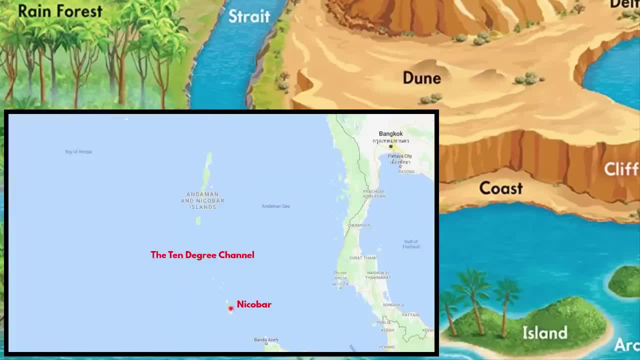 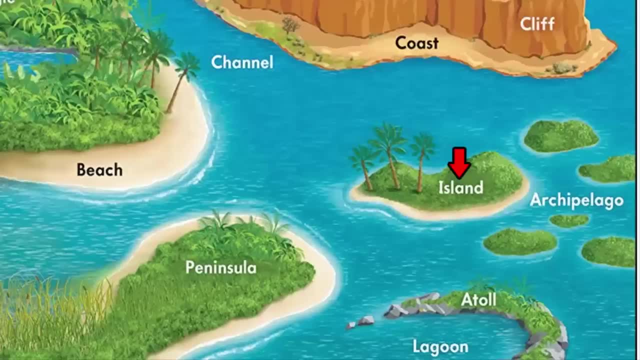 separates the Andaman Islands and the Nicobar Islands from each other in the Bay of Bengal. Let's go to the next land form: Islands. An island is a piece of land that is completely surrounded by water. When we say water, it can be a sea, ocean, river. 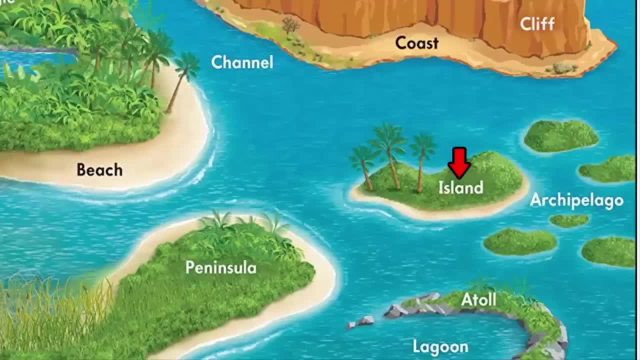 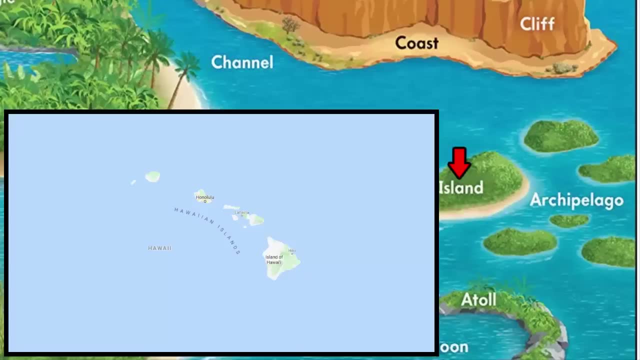 and lake. When we try to look at its formation overall, there are four general ways that can explain the formation of an island. When you take a look at the islands of Hawaii, they were formed by underwater volcanoes. Volcanoes would keep. 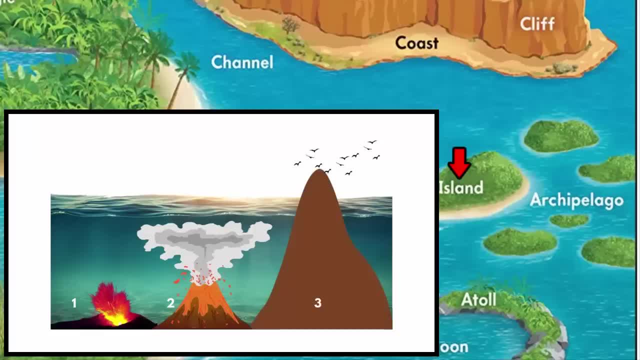 erupting. as a result, land starts to form underwater. This land would keep on rising up as the volcano erupted Over thousands of years. the land would go above the water, forming a sea mount, And that is how an island is formed. 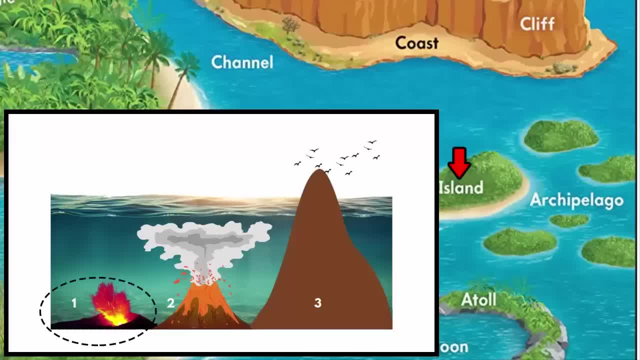 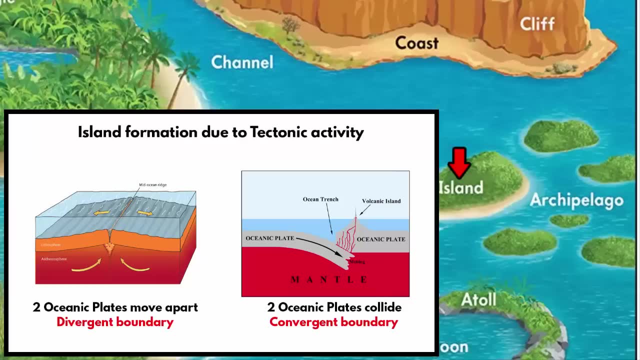 But if you go back a little and try to understand how volcanoes occur under sea, then you will realize that when two oceanic plates collide or move apart, it leads to the formation of volcanic islands. So even tectonic activity plays a role in island formation. 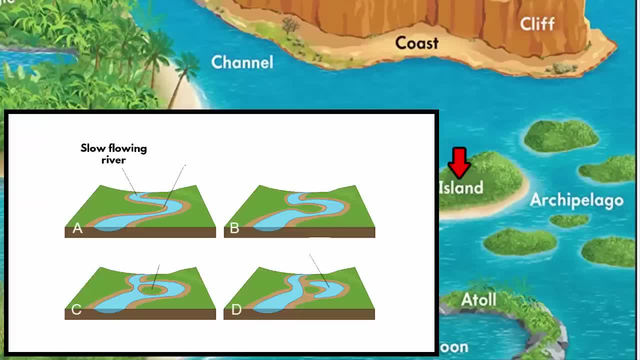 The third way by which an island is formed is through deposits of sand that came from erosion. When rivers flow, sand and other debris are picked up by the river current, which is called erosion. These sediments get deposited in certain areas Over time. 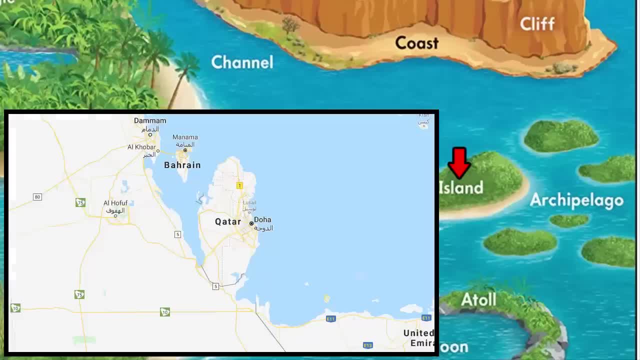 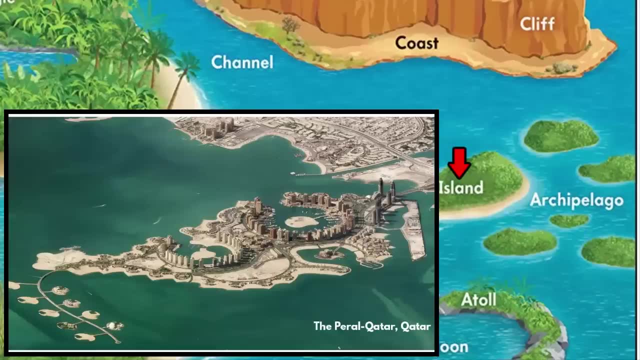 it creates a landmass which is nothing but an island. And then, finally, islands can also be man-made. The country of Qatar, which is an island itself, has made islands in many shapes to build communities on. Another one is the famous Palm Jumeirah: It is an artificial. 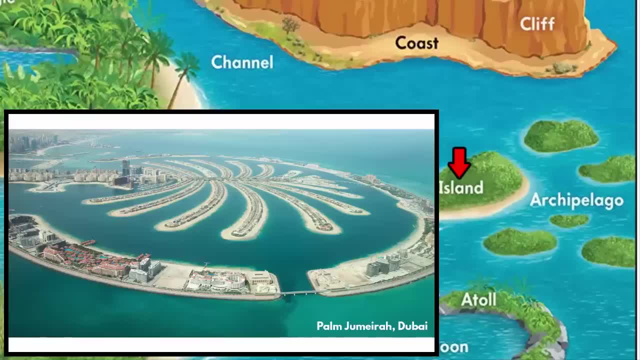 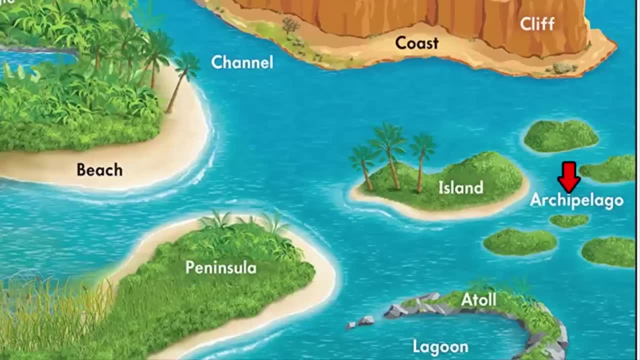 island in Dubai, UAE, which is made in the shape of a palm tree. In India, the Andaman and Nicoba islands are of volcanic origin. The next one is archipelago. They are also islands, But the only difference between an island 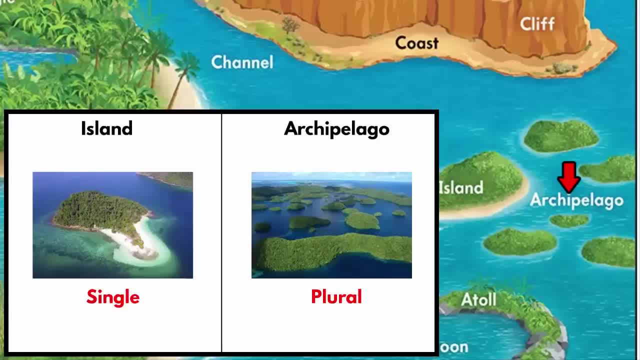 and an archipelago is that archipelago is the plural form of an island. In other words, archipelago is the name given to a group of islands. So an island is singular, whereas archipelago is plural, which means group of islands. 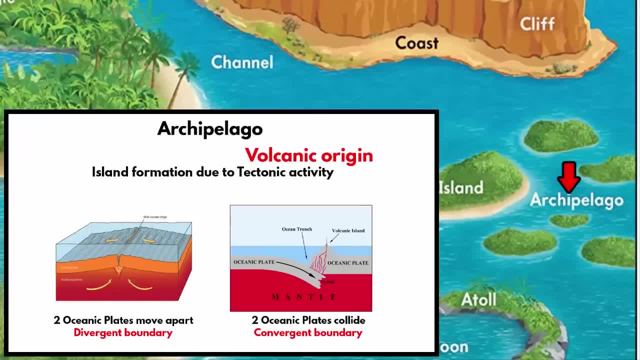 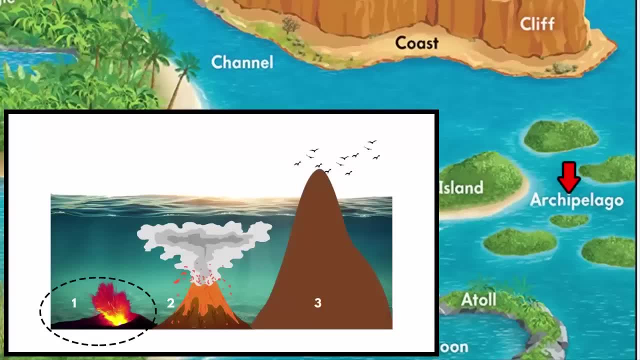 Most archipelagos are of volcanic origin. That means the islands were formed by volcanoes erupting from the ocean floor. In the previous term I have explained how underwater volcanoes are formed. These are basically sea mountains and the existing group, The Hawaiian islands. 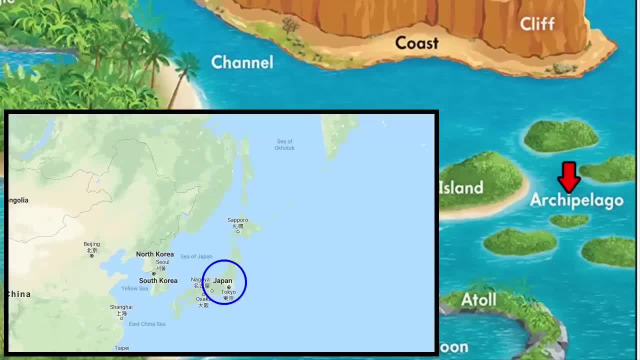 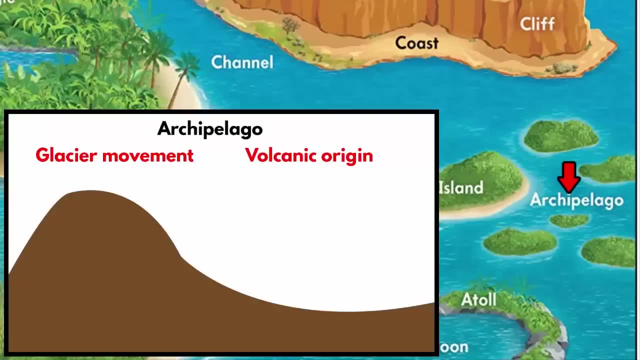 are a good example of volcanic archipelago, Then islands of Japan is a good example. There is another way archipelagos are formed. That is through glacial activity. We know that a glacier is a large piece of ice that moves very slowly. When glaciers 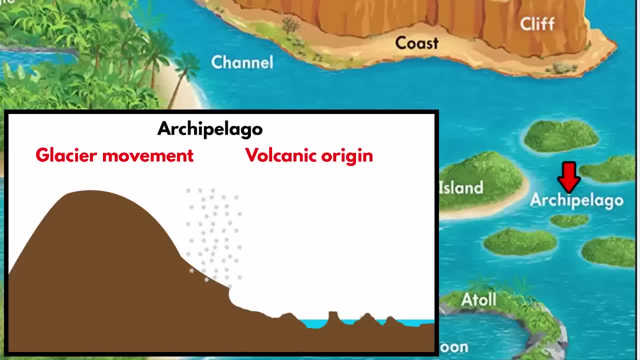 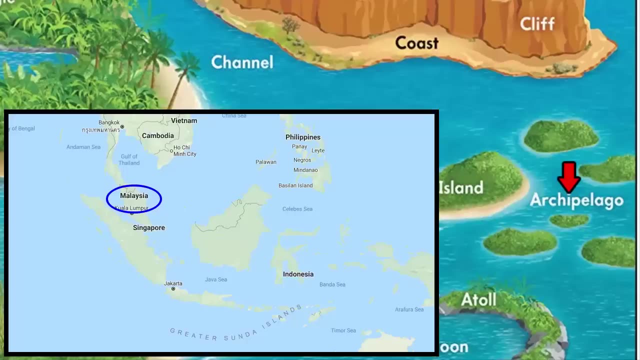 move, they cut out the land, creating a depression, and then it fills in with water and this creates islands that weren't there before. Many archipelagos that are found in lakes and rivers were created by glacial activity. Thousands of islands of Indonesia and Malaysia are a part of 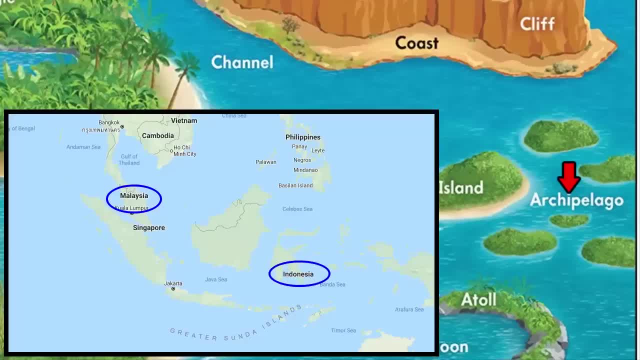 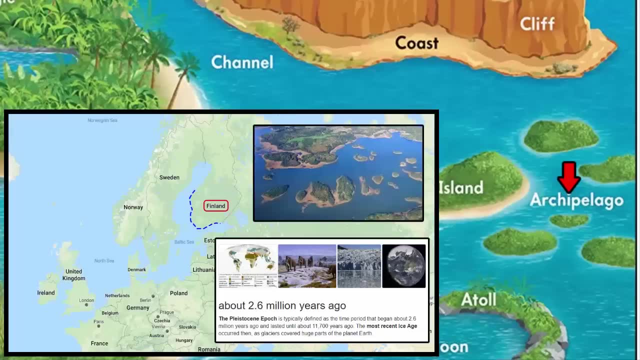 the Malaya archipelago. At least some of these islands and the straits that separate them were part of mainland Asia during the last ice age. Then Finland's coast has world's largest archipelago, which are part of the Baltic Sea. They also emerged. 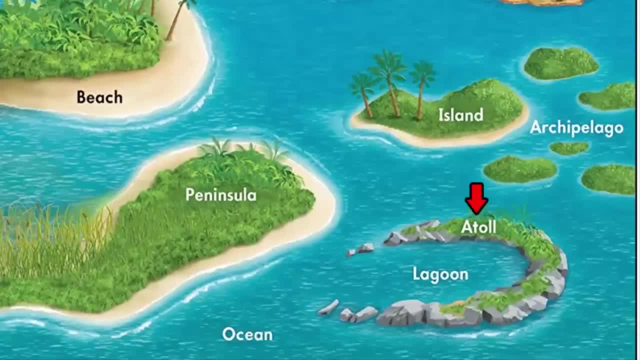 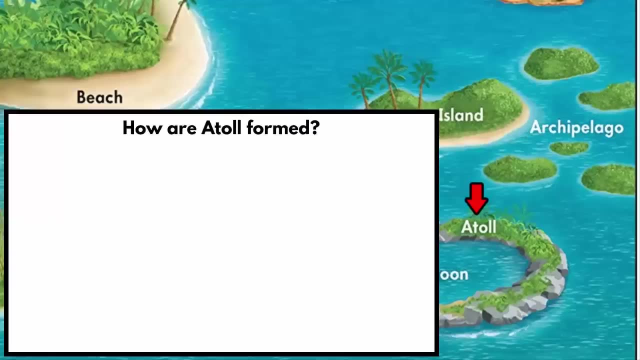 after the last ice age. The next one is Atoll, And Atoll is a ring shaped coral reef island. How is it formed? At first, there is an underwater volcano that creates a sea mountain. We have already seen how a sea mountain is formed. 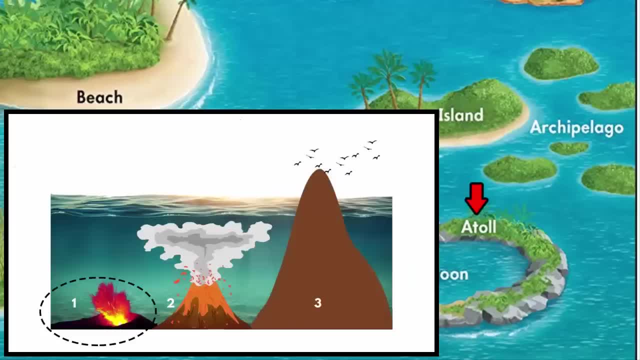 We know that a volcano erupts underwater and piles up the sea flow with lava. As the volcano continues to erupt, the sea mount's elevation grows higher, eventually breaking the surface of the water. The top of the volcano becomes an oceanic island. So this is how. 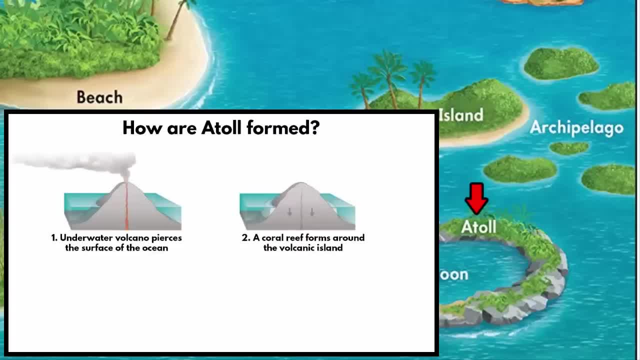 a volcanic island or a sea mount is formed. Now, in the next stage, tiny sea animals called corals begin to build a reef around this island. These corals are very hard in nature. It surrounds the island just below the ocean surface Over millions of years. the volcanic 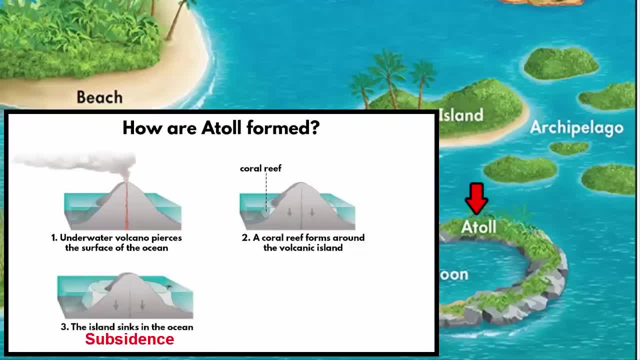 island erodes and sinks to the sea floor. This process is called subsidence. The sea mount erodes into the sea and its top portion is made flat by the constant pounding of powerful ocean waves. Ultimately, the island sinks below the sea and all you can see is a ring shaped. 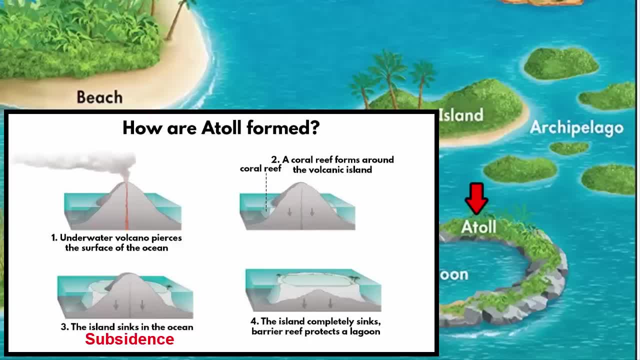 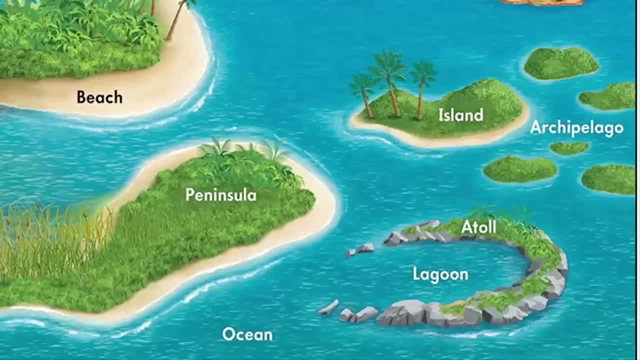 island formed with coral reef. This is what is known as an atoll, And in between you will have a pool of water which is called a lagoon. The next one is Lagoon. The simple definition of a lagoon is when a shallow body of water. 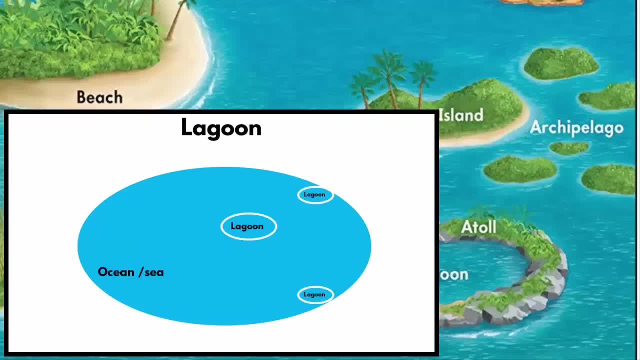 is separated from a larger body of water like a sea or an ocean. That is what is called a lagoon. Now, the key point to remember is that this shallow body of water should be nearer to a sea or an ocean, Because the water of a lagoon has to come from a 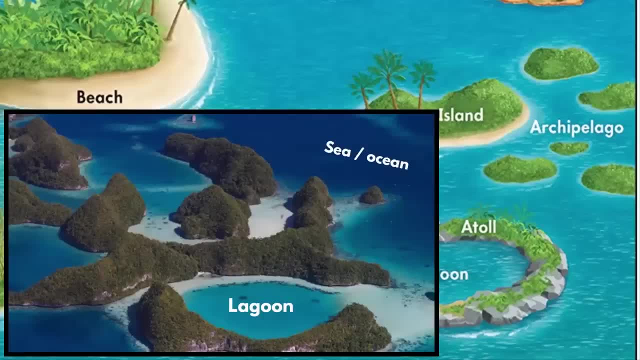 sea or an ocean. Otherwise a simple lake can also be called as a lagoon. But then if a lake is near to a sea or ocean and somehow the lake gets water from the nearby sea or an ocean, then we call it a lagoon. 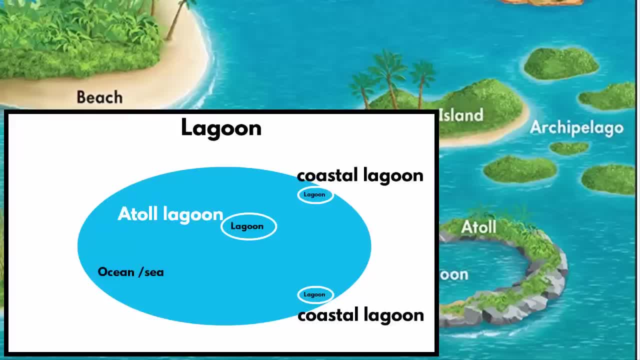 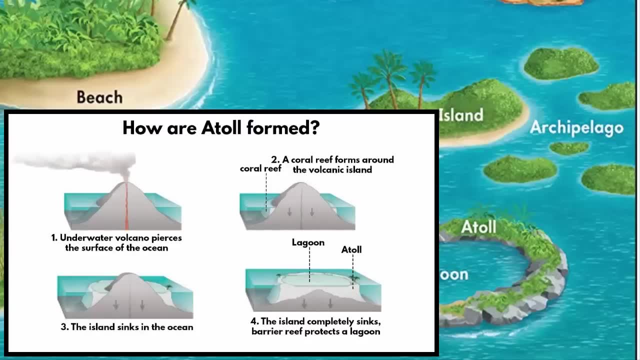 Lagoons are of two types. In the previous point we learned about atoll. At the center of an atoll you will find a lagoon, And this type of lagoons are called atoll lagoons. However, lagoons can also. 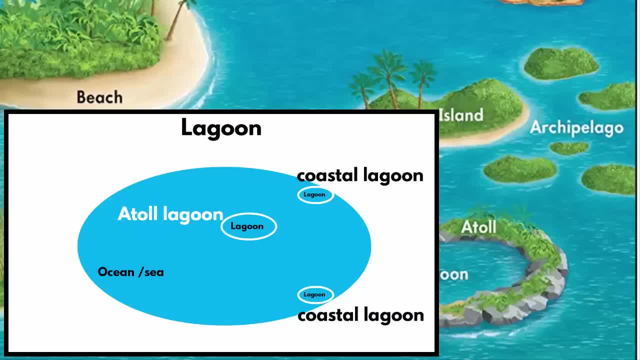 occur near coastlines. Suppose you are near to a coast. Usually you will find a coastal lagoon where the coastline has a gentle slope Because the sediment gets continuously washed away by the sea or ocean, And then the sediment churns and turns into a sand ridge or 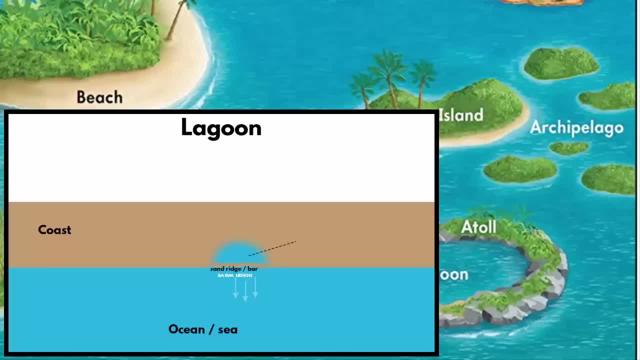 a sand bar. As a result, a small pool of water gets separated from the ocean. This is how a coastal lagoon is formed. Now, this coastal lagoon is connected to the ocean by a small stream. That's how the lagoon gets its. 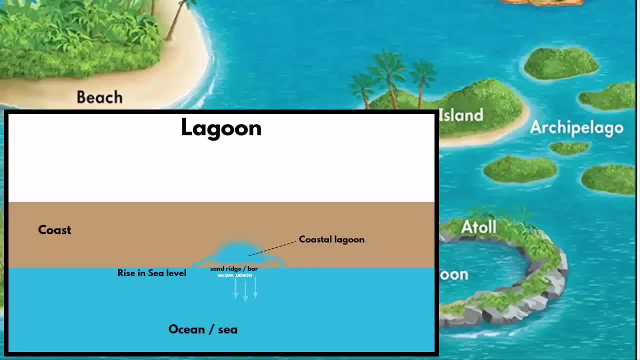 water supply. Apart from this, there is another way the coastal lagoon gets its water, And that is when the sea level rise. But when the sea level rises, it impacts the coastal lagoon's landscape to a great extent. The most famous lagoons in India include the: 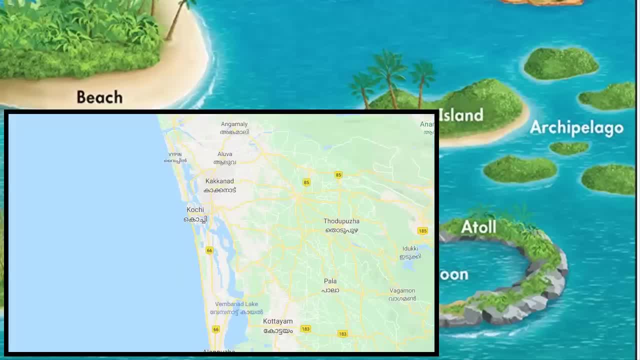 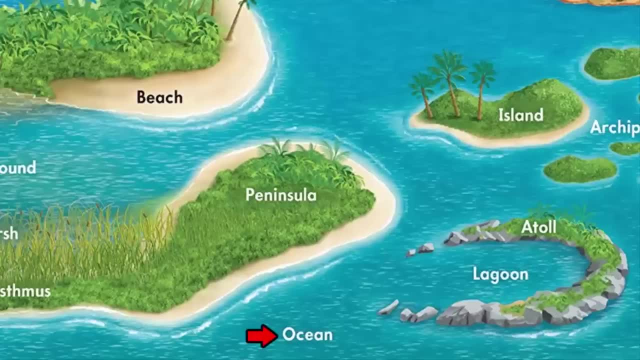 Chilika lake, the Kaliveli lake, the Kerala backwaters, Pulikat lake and Vembanad lake. The next one is ocean. When we think about the planet earth, we cannot forget oceans, Because the reason earth looks blue is due to. 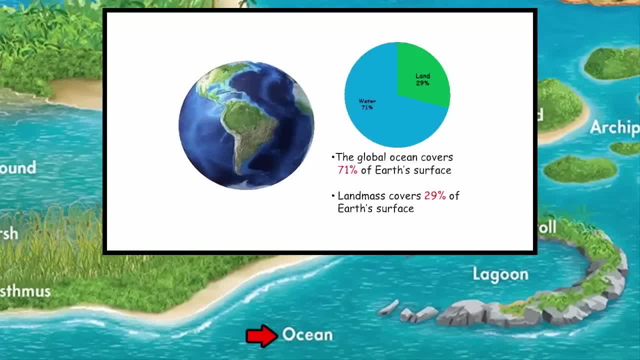 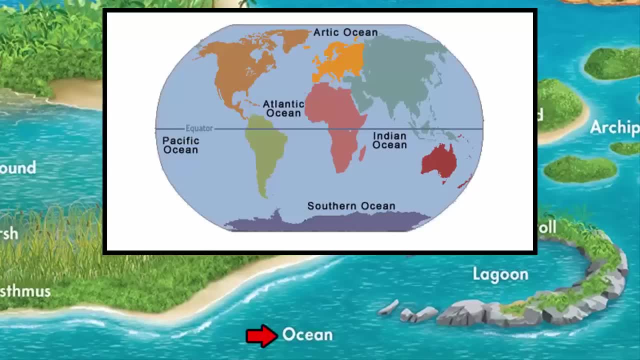 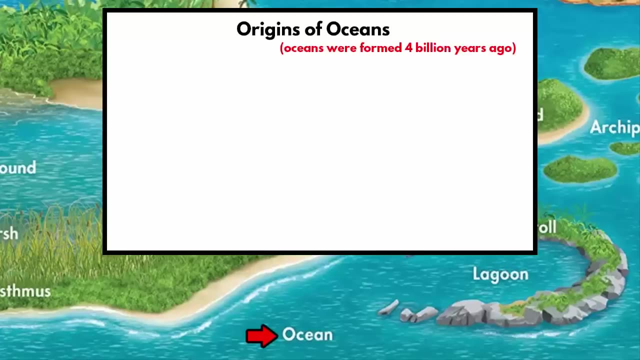 the oceans. The surface of the earth is approximately 71% water and contains 5 oceans, including the arctic, atlantic, indian, pacific and southern. The most popular theory behind how earth got its ocean is that the ocean was formed 4 billion years ago. 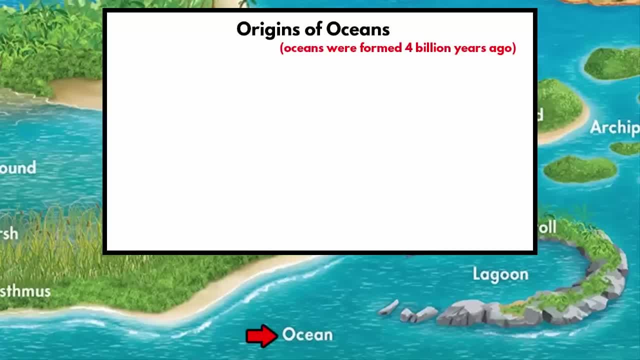 with the continual degassing of the earth's interior. We all know that the earth was formed over 4.5 billion years ago. When the earth was formed, it was a hot molten rock. There was no liquid water anywhere on earth. 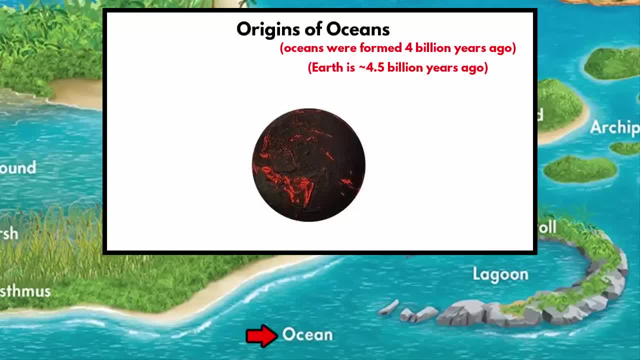 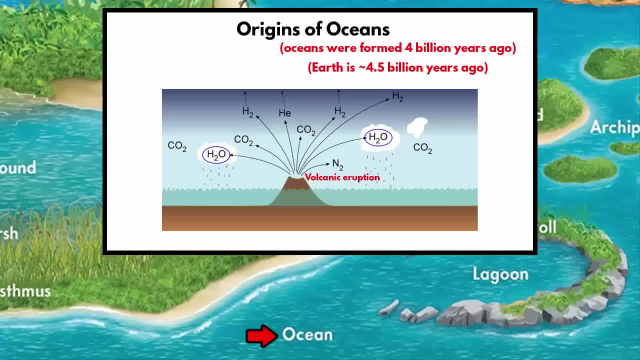 But the ingredients that were required for water were there. When volcanic eruptions took place, one of the gases that came out of the earth's core was steam, which is basically water vapor, And when the planet slowly cooled this steam or water vapor, 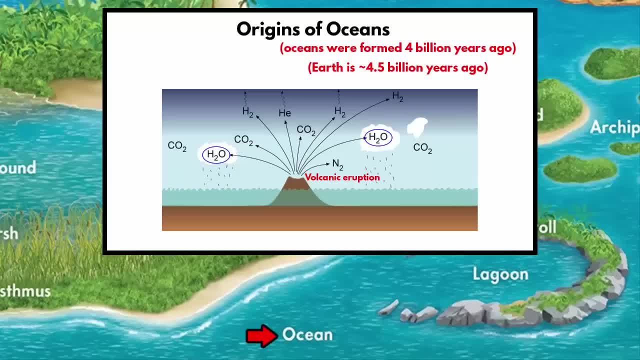 turned into clouds, Then rain began to fall and continued to fall for thousands of years. Then the water started accumulating at the lower areas of the earth's ground, possibly creating the ocean. And then it is also believed that some of the water also came from the. 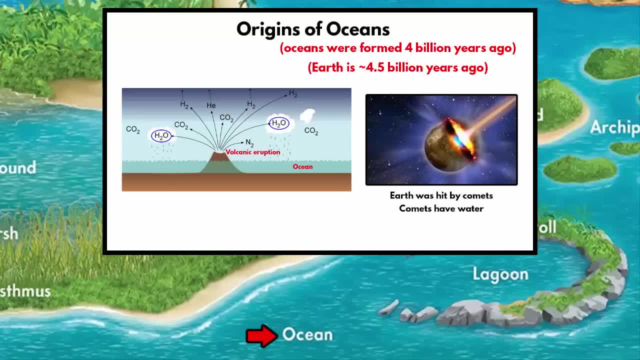 outer space There are comets which are filled with water. It is said that in the beginning years the earth was hit with thousands of comets And this kind of bombardment delivered half of the ocean water that we see today. The next one is peninsula. 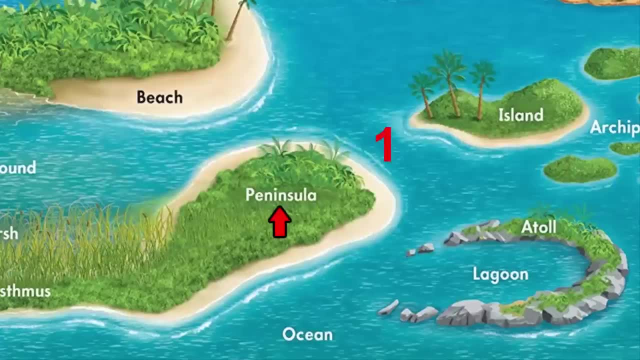 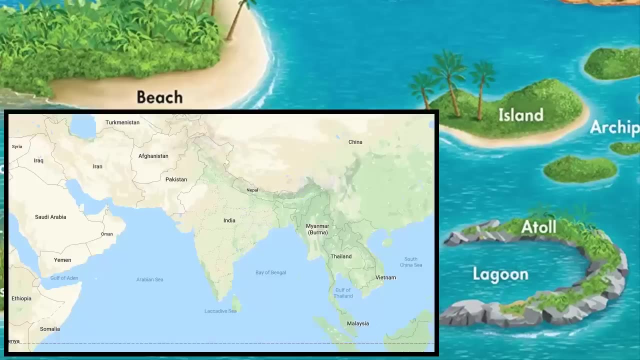 Now, what is a peninsula? It is a piece of land that is surrounded by water on three sides, But the fourth side is connected to the mainland. For example, India is a peninsula country Because it is surrounded by the Bay of Bengal in the east. 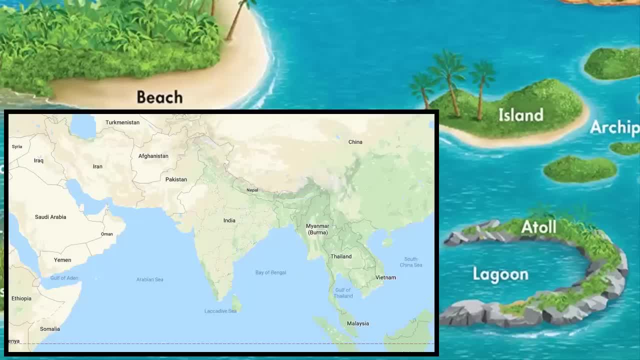 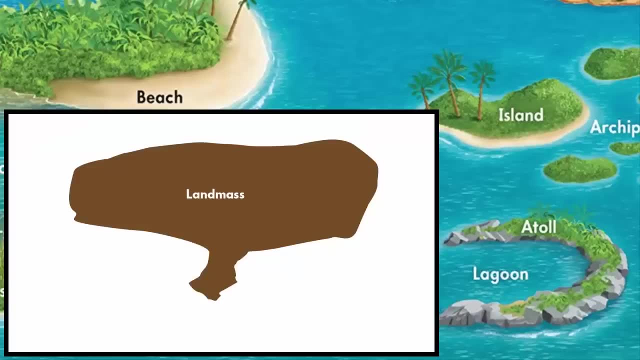 Arabian Sea in the west and the Indian Ocean in the south. It is connected to a larger body of land. How are peninsulas formed? A peninsula can be formed by rising or falling of the sea level that may expose or cover portions of land. 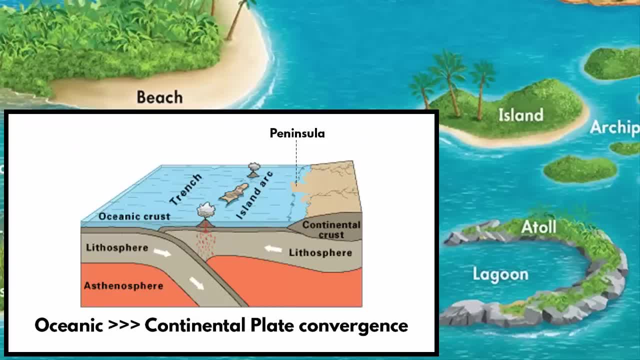 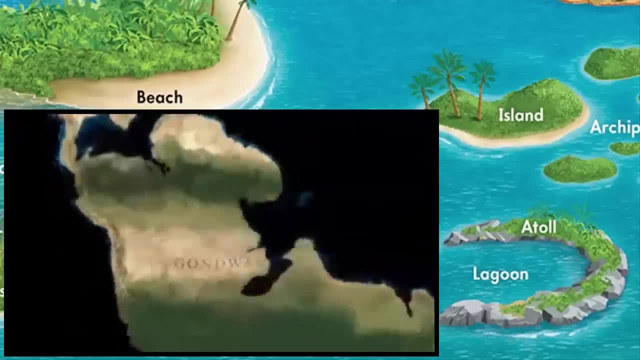 to form a peninsula. Even due to tectonic activity, upliftment or falling of land mass may also help to form a peninsula. A separation of land masses over millions of years can create a peninsula Again. a good example is the Indian subcontinent. 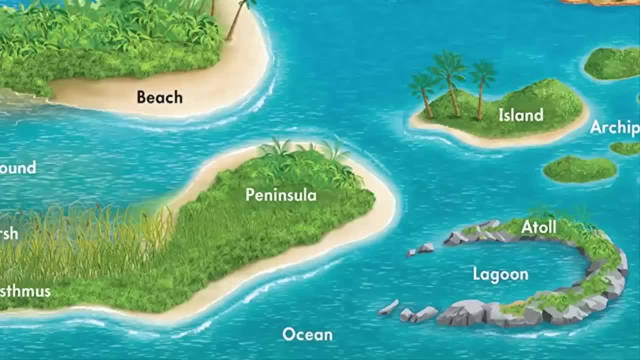 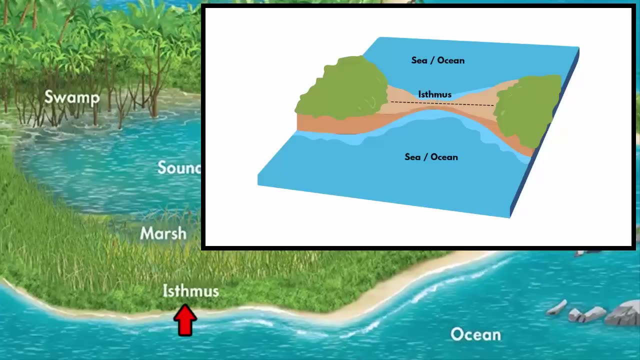 which broke away from the ancient continent of Gondwana. The next one is Isthmus. It is a narrow strip of land with sea on either side, forming a link between two larger areas of land. One of the most famous example of the Isthmus landform. 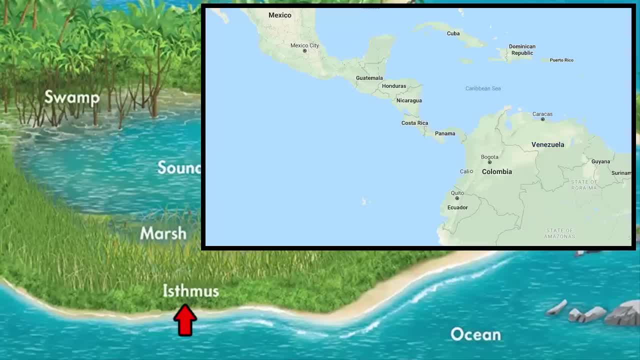 is the Isthmus of Panama. The Panama Isthmus is a narrow strip of land that connects Costa Rica and Colombia. Essentially, the Isthmus of Panama connects North and South America. It is in between the Caribbean Sea and the Pacific Ocean. 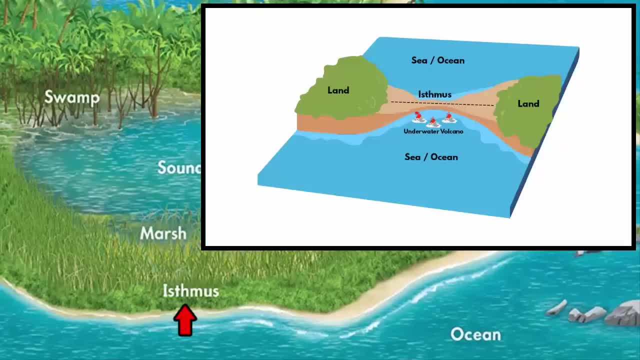 In addition, an Isthmus can be formed by volcanic activity, which then creates sea mount, which then forms a chain of islands and block water on either side, forming an Isthmus. This is how the Isthmus of Panama was formed. Another way an Isthmus is formed. 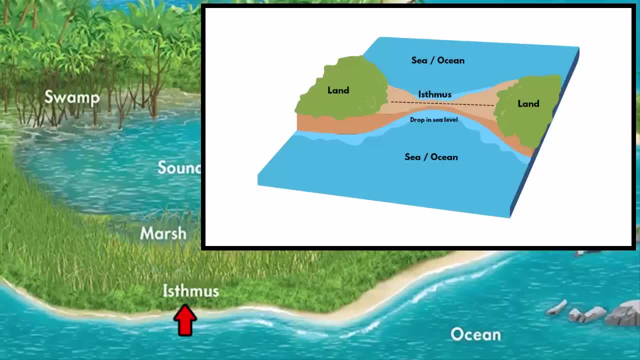 when there is a drop in the sea level, which will then expose more land, and this is also an Isthmus. The next term is Marsh. It is basically a wetland. If you look at the area, it is a low lying land which gets filled with water. 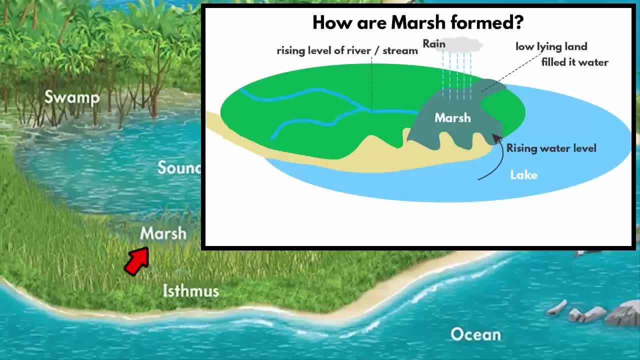 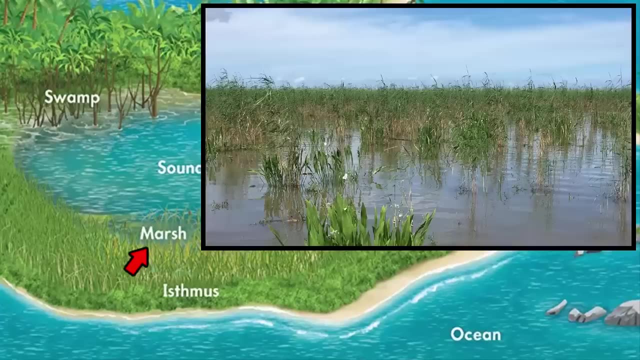 during rainy season or from rising water levels of a river, lake or stream? And how does a land become a low lying land? Through continuous erosion processes or through deposition of sediment on nearby lands during floods? A marsh is always covered with water throughout the year. You will mostly find marshes at the edges of rivers, lakes and streams. Talking about the vegetation, these places are dominated by grass and other herbaceous plants. You will not find trees. These plant roots holds the muddy soil tightly and slows down the flow of water. 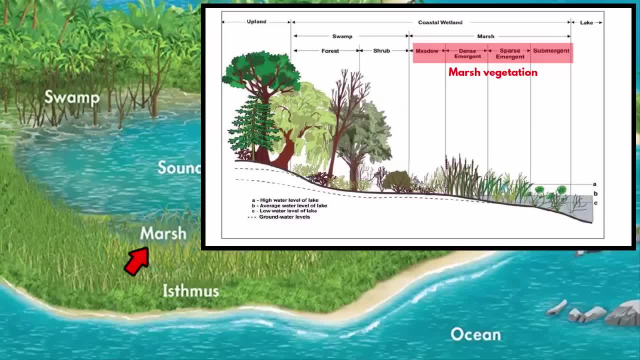 This is how marshes are flooded with water all the time. Marshy area of land is also rich in biodiversity. That is why these landforms are conserved and protected throughout the world. The famous Ramse convention on wetlands is a good example of what I am saying. 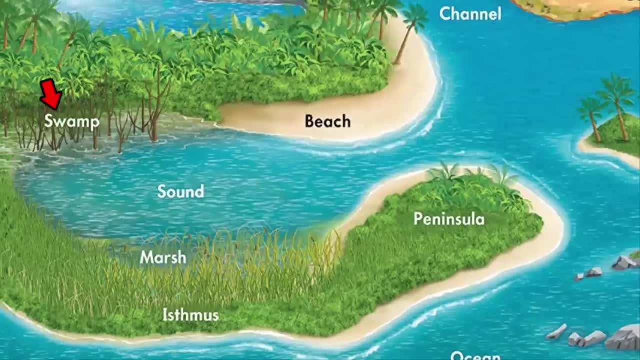 The next term is swamp. If you look at their locations, both are almost at a similar place, Closer to a water body. So both a swamp and a marsh is a wetland. Both of them has similar characteristics in their landform. However, the only difference between a marsh and a swamp is that in a marsh area you will not find trees, You will only find grass and herbaceous plants, Whereas in a swamp you will find trees and other woody plants. Otherwise, both of them are. 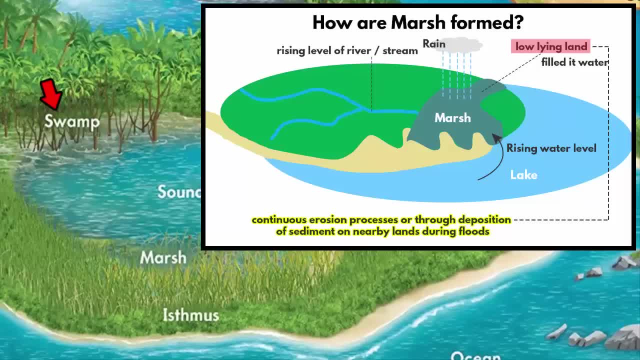 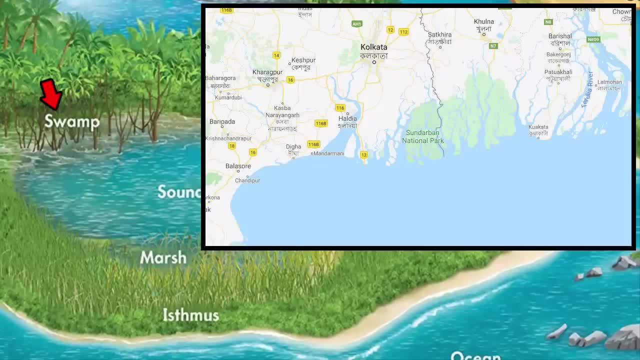 a low lying land which gets filled with water during rainy season or from rising water levels of a river, lake or stream. In India, we know that Sundarban is a mangrove area. The moment you think about mangrove, you will find woody trees and plants. 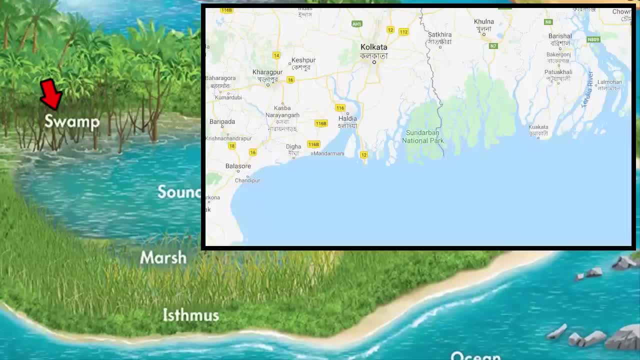 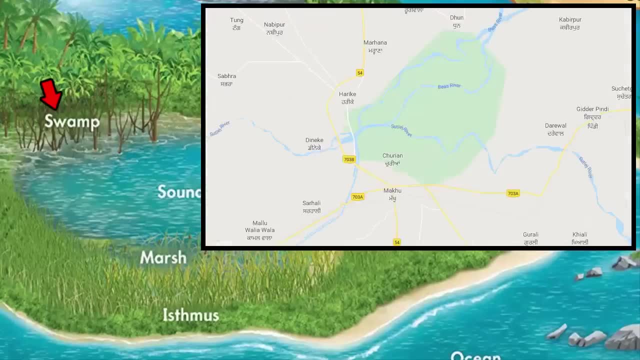 That means the Sundarban wetland is a swamp and not a marsh. Plus, it is next to the Bay of Bengal. that means it is a salt water swamp. Similarly, if you look at the Harikay wetland in Punjab, you will find grass and herbaceous plants. 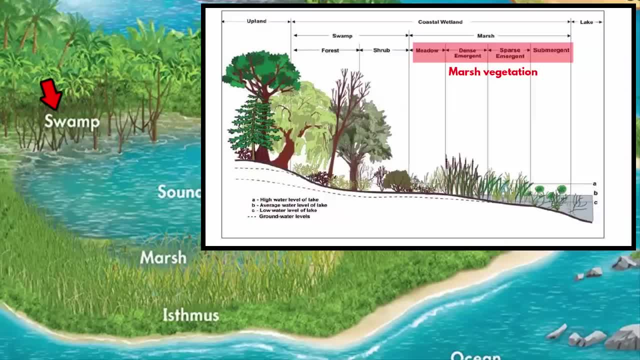 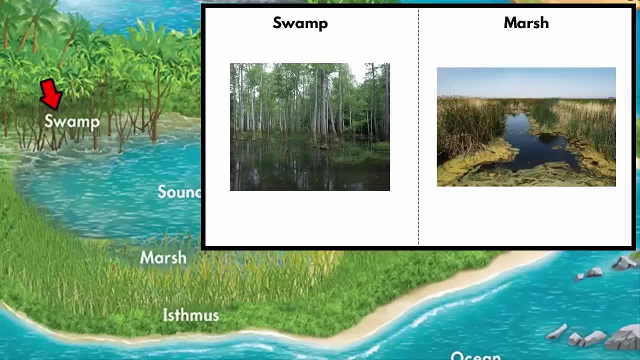 That means it is a marsh. So the only difference between a marsh and a swamp is the existence of trees. If there are trees and woody plants, then it has to be a swamp. Please remember this point. The next one is sound. It is a geographical term. 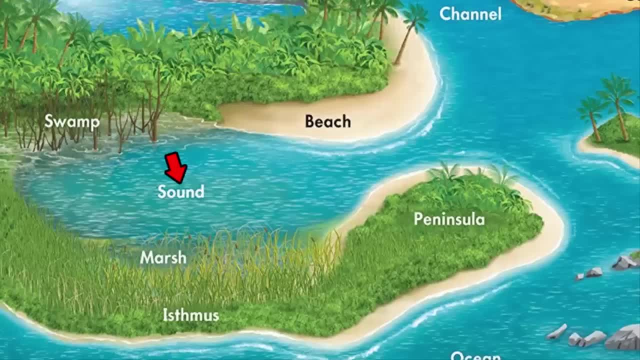 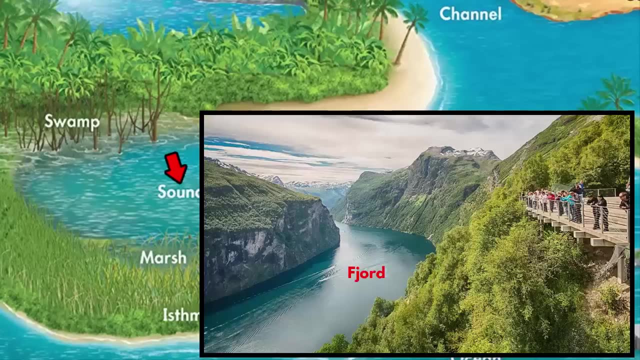 Please don't think of it as a sound wave. A sound is a large sea or an ocean inlet that separates two land masses. Now, if you remember, in the beginning we read about a term called jod. These are long, narrow, deep inlet of the sea between high cliffs. 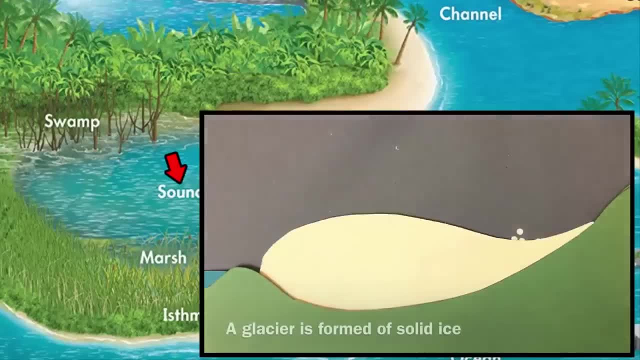 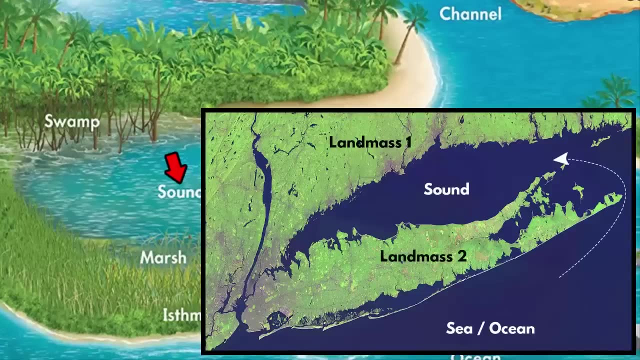 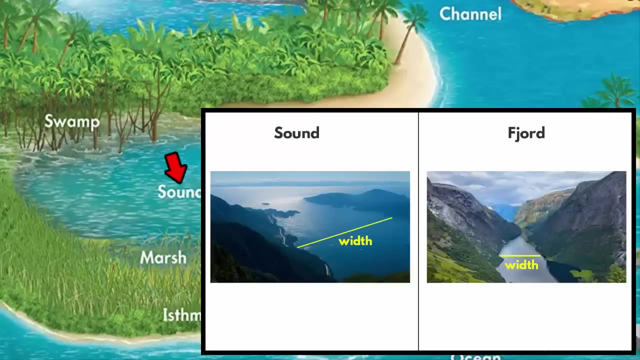 And they are created by glacier, by carving a whole valley, and then water fills in that land depression. Similarly, a sound is a large depression of land which gets filled in with sea or ocean water. Plus, it is much wider in size, Much wider than a jod. 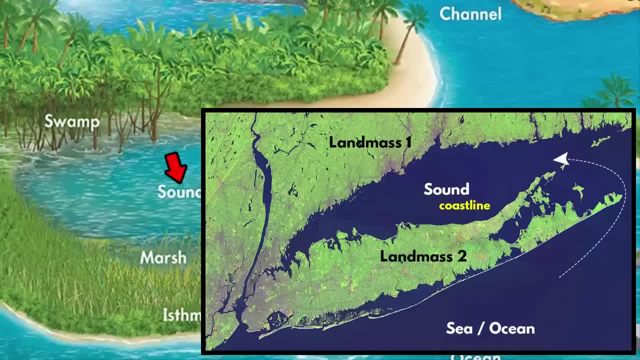 You will find a sound only near the coastlines of the world And the water is from sea or ocean. that means it is a salt water land form. If you look at this land form, you will find that this area has to be a low lying land. 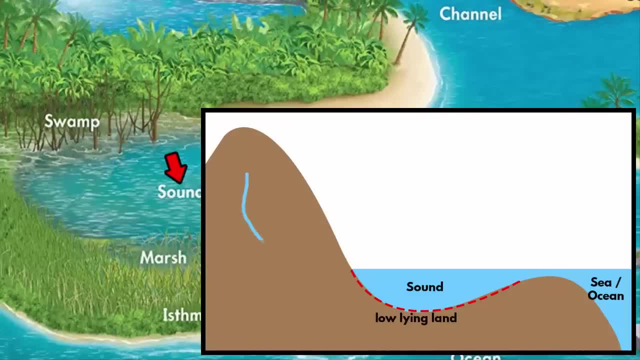 And that is how the water from the ocean or sea gets filled in. Now, this kind of a land depression usually occurs through erosion processes, Or let's say, a river that is coming from the land and joins the sea Due to a rise in the sea level. 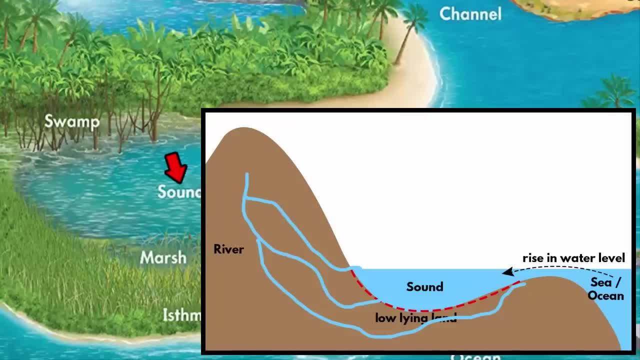 and since the flow of river has already created a depression in the land and now, due to a rise in the sea level, the river gets flooded with the sea water. Since it is a large sea or ocean inlet, it is much deeper in depth and wider in size. 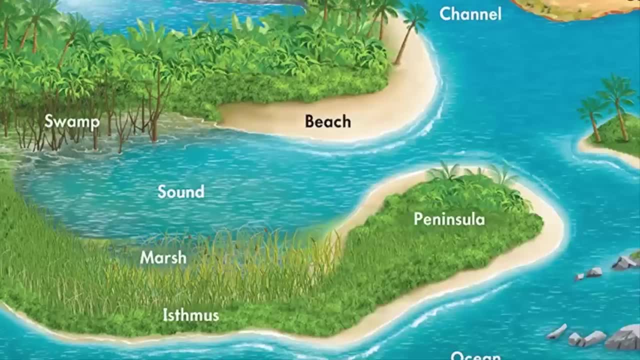 That means it can also be called as a bay or a harbour. The next one is beach. When you look at the beach, you will notice that this kind of a land form is always next to a water body. May be a sea or an ocean. 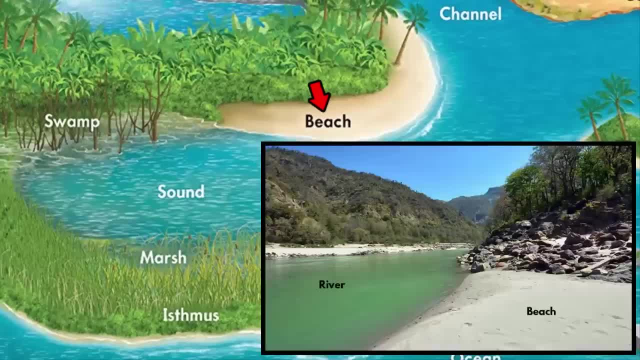 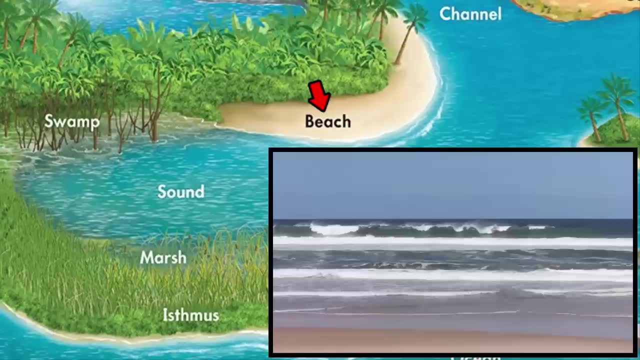 Even next to a large river, you will find a beach On a beach. if you look at the land, you will find that it is composed of sand, rocks, shells and pebbles. Moving water constantly erodes the land and turns them into loose sand. 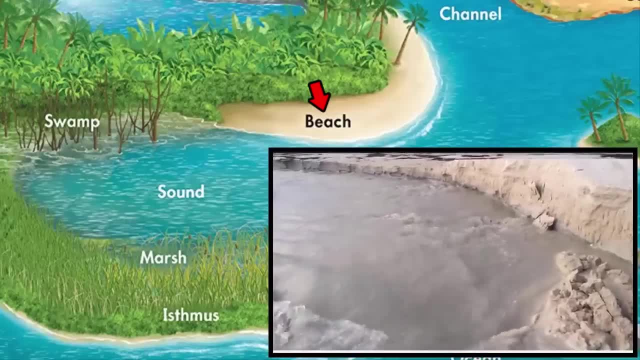 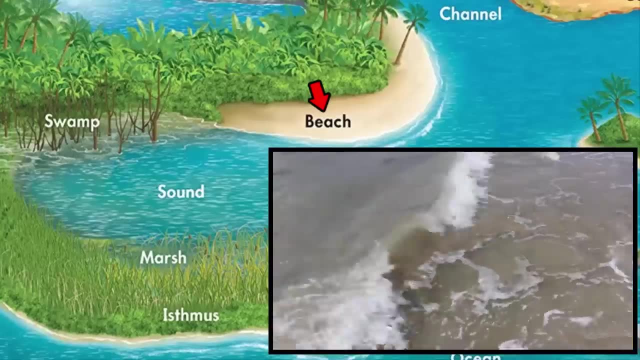 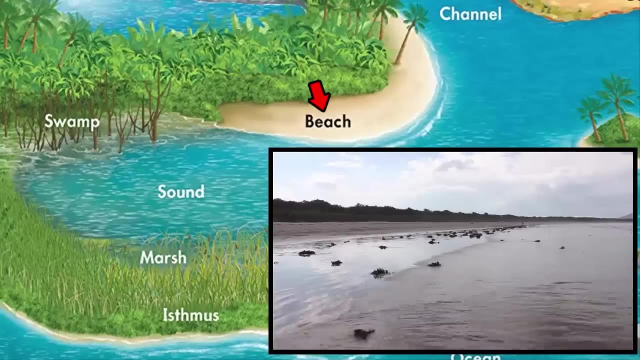 Additionally, rivers and rain water also erode rocks located further inland. These sediments flow through rivers and gets deposited along the coastline When the waves of the ocean or sea continuously hits the shore. every time the wave hits the shoreline, they erode the existing sediment. 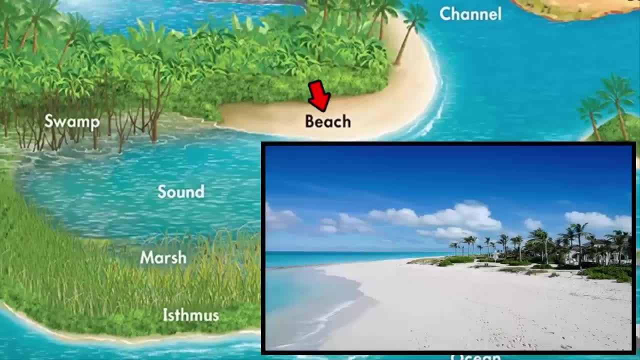 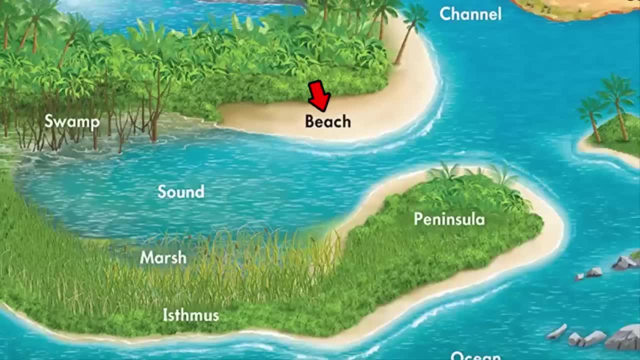 and rolls them over and over again. If the waves are strong, it will spread the sediment along the coastline to create a beach. By the way, the shape of the beaches keeps on changing. Tides and weather can alter beaches every day, bringing new shapes to the coastal. 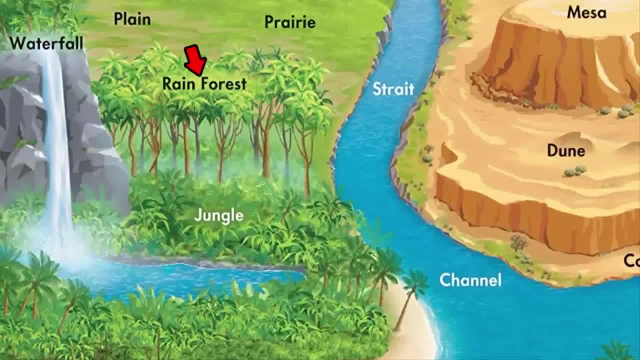 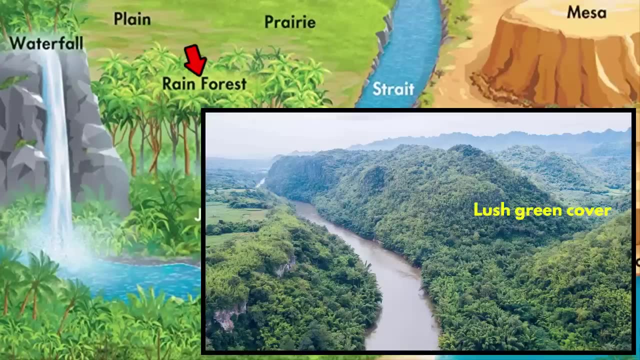 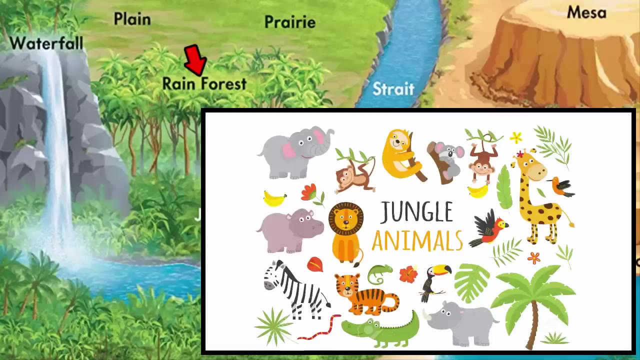 landscape. The next one is rainforest. It can also be called a jungle. The most common meaning of a jungle is a land filled with natural vegetation and has a vast lush green cover of trees, plants, grass, herbs, etc. Apart from natural vegetation, you will. 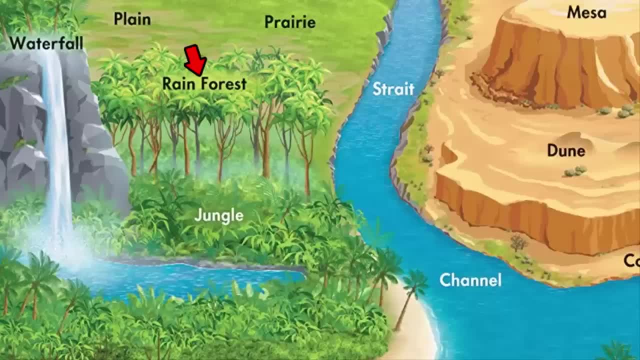 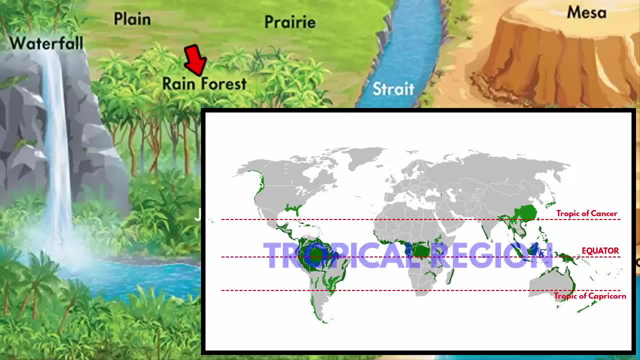 also find a variety of animal species. Most of the jungles in the world can be found in the equatorial region, In other words tropical region. When we say tropics, it lies between the latitude lines of the Tropic of Cancer and the Tropic of Capricorn. 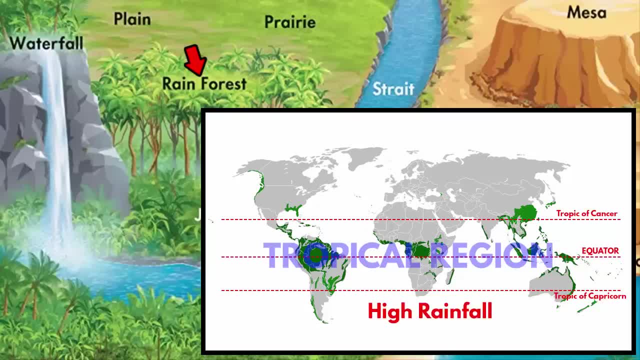 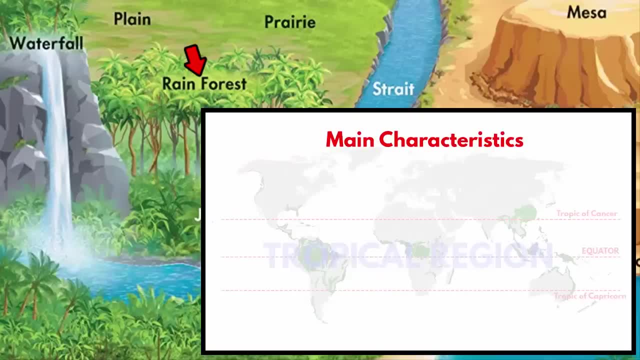 And we also know the tropical region receives very high amount of annual rainfall. This is how the name rainforest came into existence. If you look at the main characteristics of a tropical rainforest they are: The first one is: these regions receive very high annual rainfall because 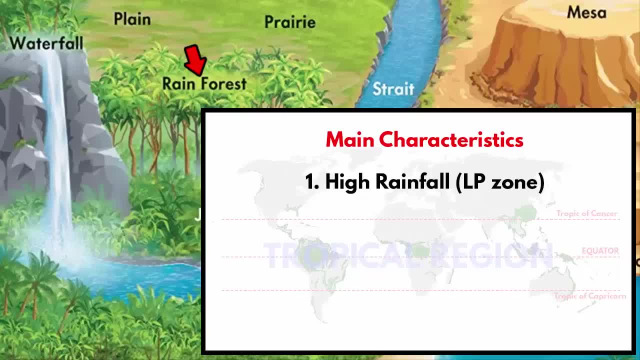 equatorial region is a low pressure zone and the average temperature is very high, which is ideal for rainfall. The second one is they have high average temperatures, which provides the necessary moisture and humidity, While the sun shines almost equally in all parts of the earth. the equator- 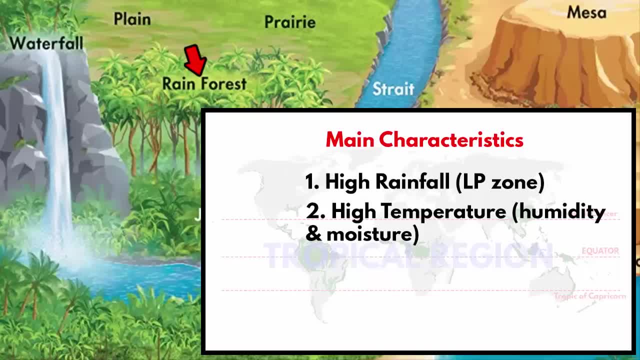 is exposed to a high amount of direct sunlight, which is the reason behind high average temperatures. And the third point is these places have very little nutrients in the soil because high volume of rain washes the nutrients out of the soil, Plus the existence of large volume. 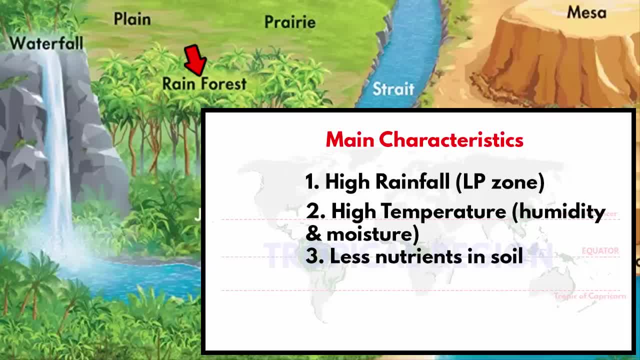 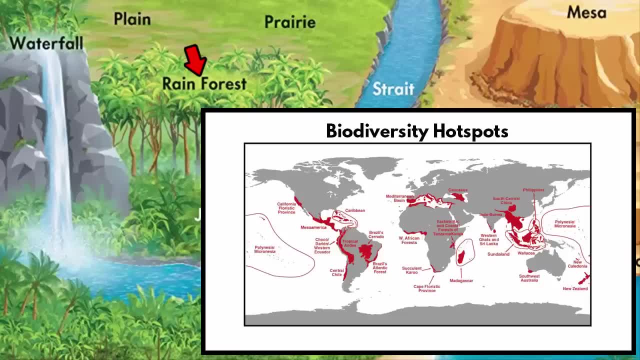 of trees sucks the nutrients out of the soil for their growth. And the last point is: equatorial region is rich in biodiversity. That is why most of the biodiversity hotspots are located in the tropical region. And the meaning of the word biodiversity is high level of existence. 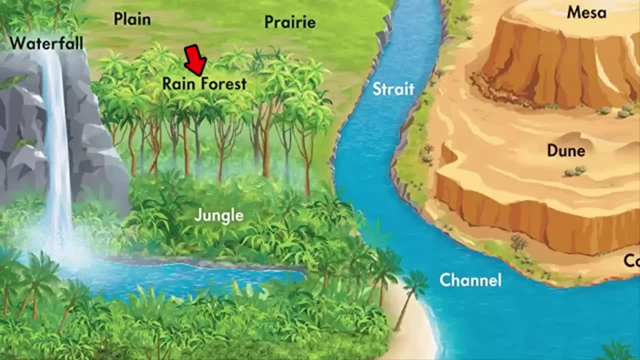 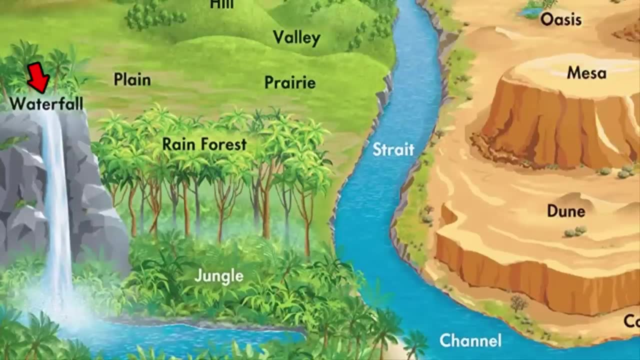 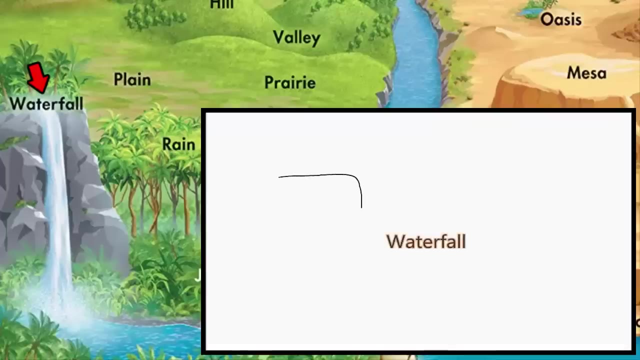 in the variety of plant and animal life at a particular place. The next one is waterfall. It is basically a stream of water or a river that flows over the edge of a cliff and then falls vertically downward. Waterfalls are formed when the river bed. 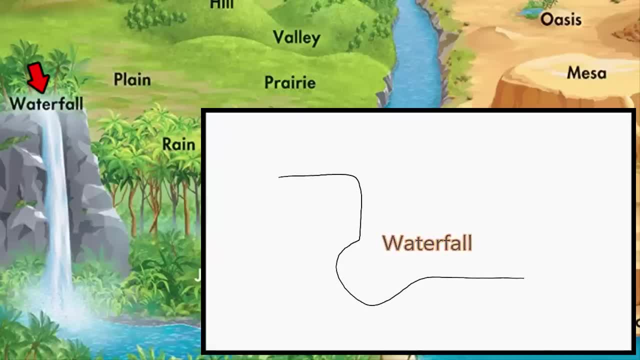 changes from hard rock to soft rock. So what happens is that the river flows on two different types of platform. One is a hard layer of rock and the other one is a soft layer. In other words, you have a river or stream flowing over a hard rock. 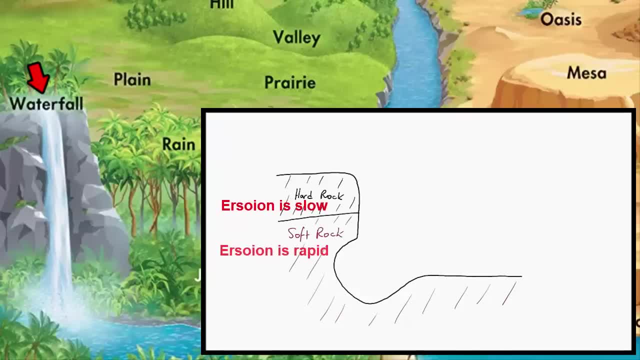 where erosion is slow, And also flowing over soft rock, where erosion is rapid. With time the soft rock layer gets eroded and becomes a low lying land. Now, when the water flows on top of the hard rock and falls on the soft rock layer, it tends to form a 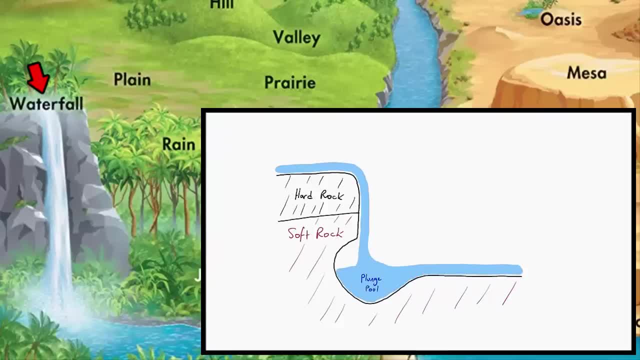 plunge pool because the speed of the water increases due to the influence of gravity. At the bottom, you will notice that a plunge pool is formed. Further it begins to undercut the soft rock layer As the undercutting continues, eventually the overhanging hard rock. 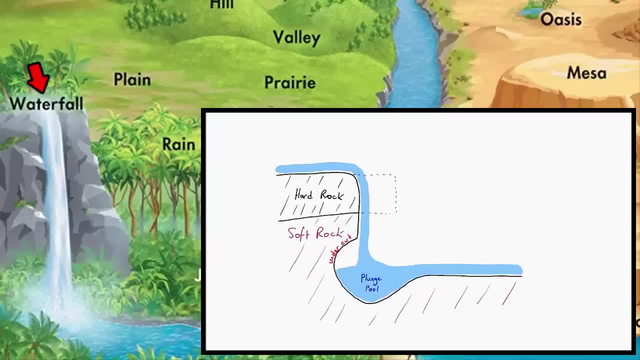 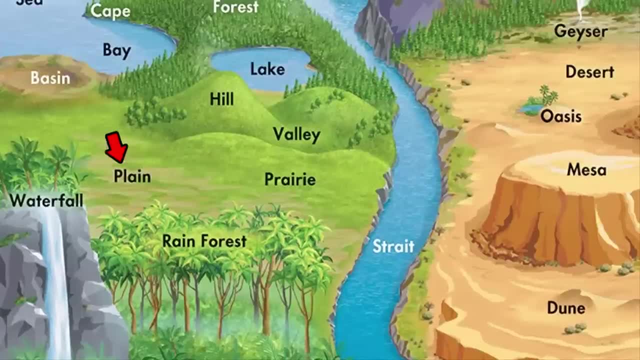 becomes unstable and collapses. As a result, the waterfall slowly retreats backwards to the remaining lip of the hard rock layer. The next one is plane. A plane is a broad area of flat land. Planes are one of the major landforms on earth. 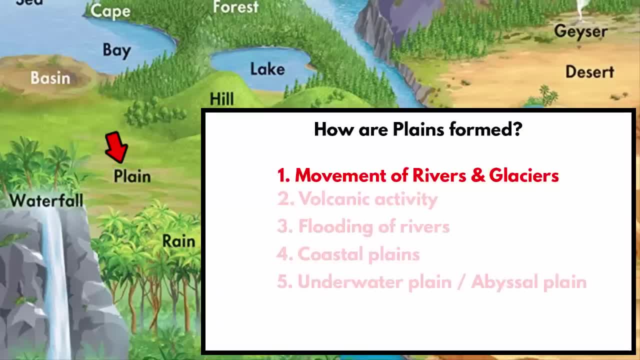 Planes form in many different ways. When ice and water flow over high elevation landform, they float the dirt and rock on higher land. Water and ice carry the bits of dirt, rock and other material called sediment Downhillside As layer upon. 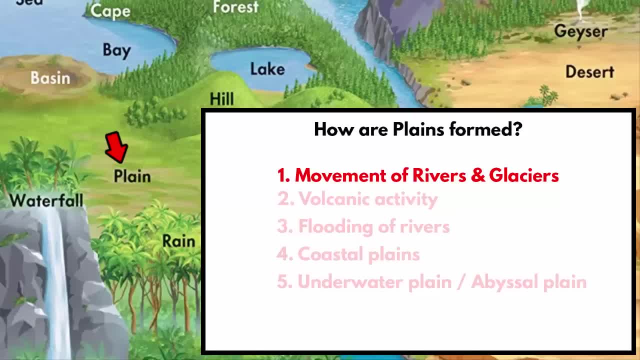 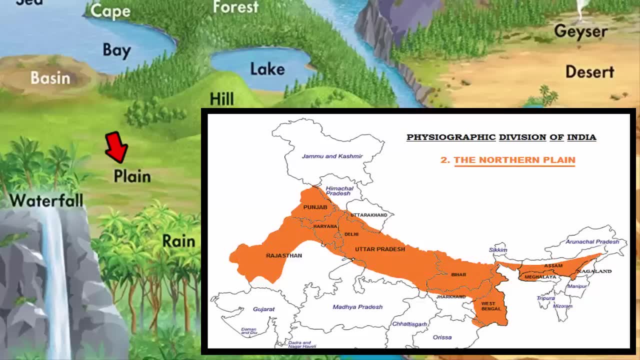 layer of this sediment is laid down, planes are formed. A good example is the North Indian plane River. like Indus, Ganga have been depositing this sediment in this plane over thousands of years. In northeast of India, the Brahmaputra plane. 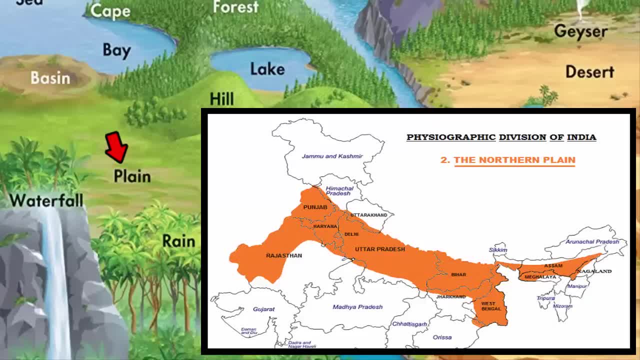 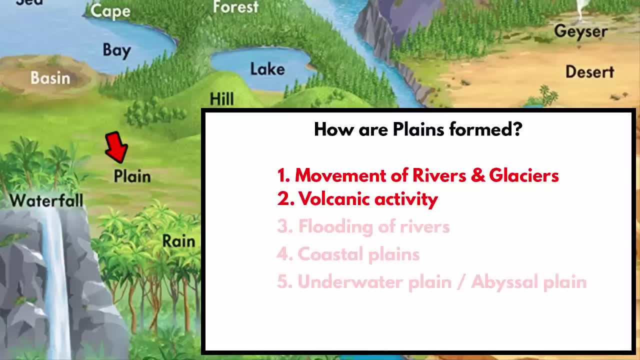 or the Brahmaputra valley in Assam, is another good example how the Brahmaputra have been depositing sediments for thousands of years. Even volcanic activity can also form planes. When lava flows out of a volcano, it spreads across the land. 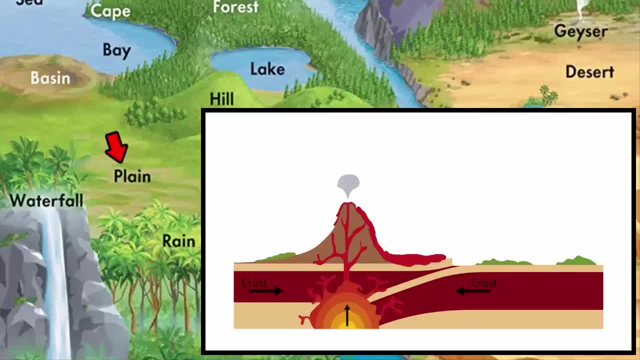 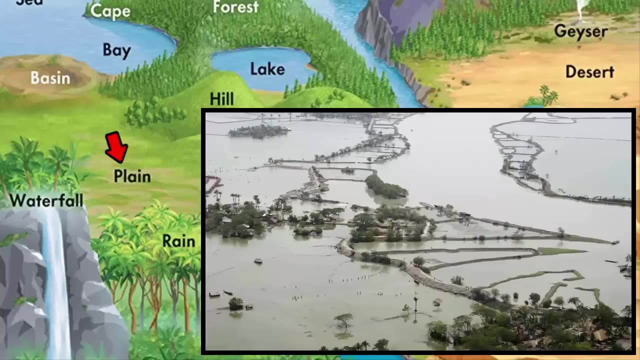 The colour of the soil is mostly dark coloured mineral called basalt. Even this soil gets broken down into tiny particles over millions of years And that is how, due to volcanic activity, planes are formed. Even flooding of rivers can form plane. As a river floods, it overflows its 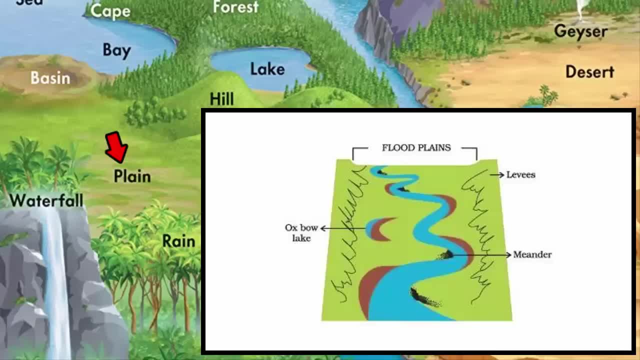 bank. The flood carries mud, sand and other sediment out over the land. After the water withdraws, the sediment remains. If a river floods repeatedly over time, this sediment will build up into a flood plane. Flood planes are often rich in nutrients and create 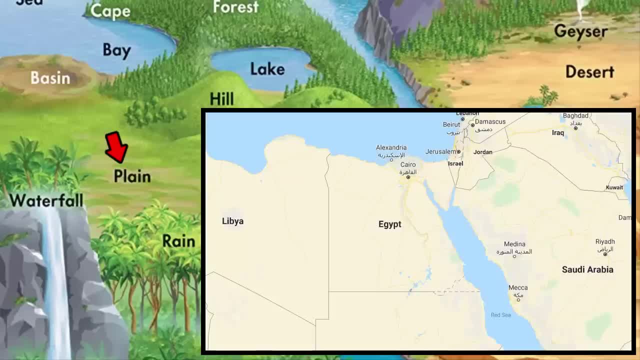 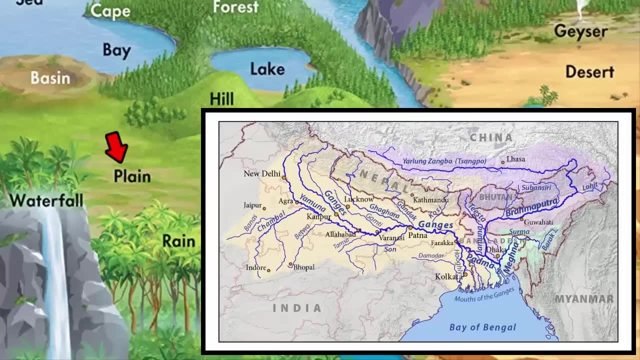 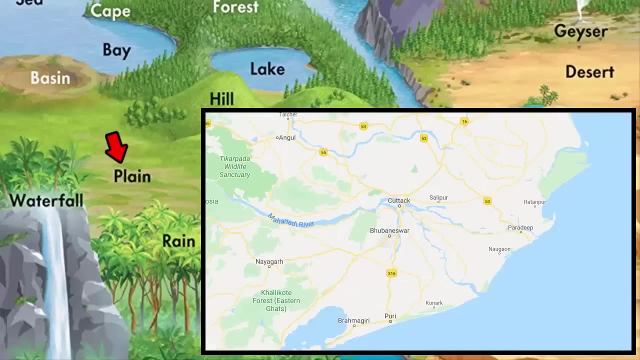 fertile farmland. The flood plane surrounding Africa's Nile river has helped Egyptian civilization thrive for thousands of years. In India, the regions near the Ganga river and Malaputra river are most prone to floods. The state of Odisha also suffers from the flooding. 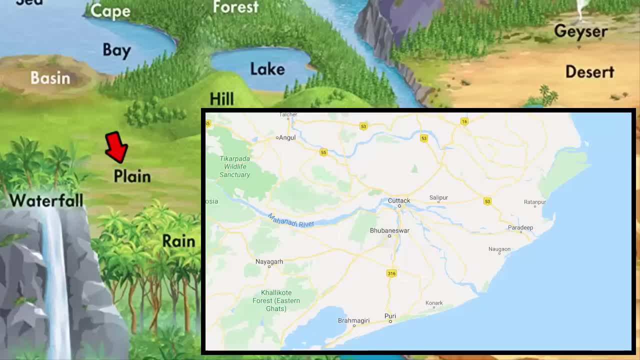 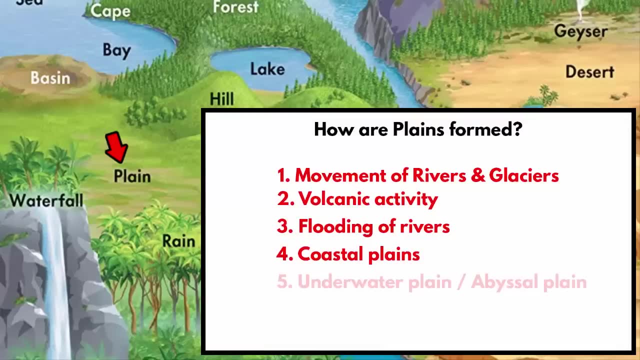 of the river Mahanadi. The Mahanadi delta region, just near to the eastern coast of India, is the most prone area of flooding. Another kind of plane is the coastal planes. Many rivers deposit its sediment in the ocean As the sediment. 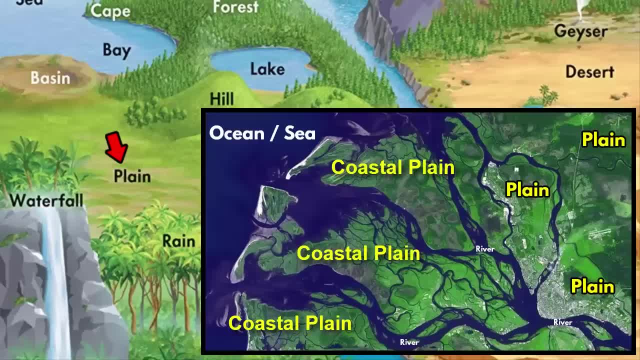 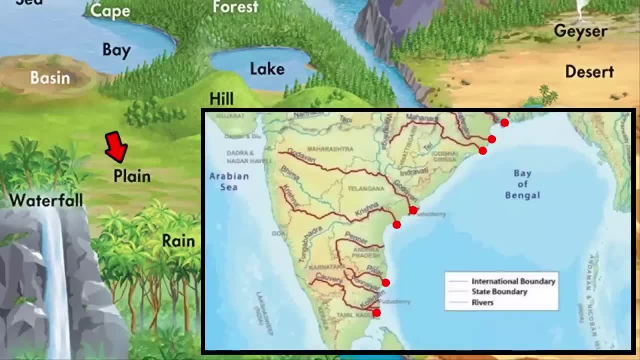 builds up. it slowly rises above the sea level, forming a coastal plane. A good example is the eastern coastal plane of India along the Bay of Bengal. Large rivers such as Mahanadi, the Godavari, the Krishna and the Kaveri have deposited large volume. 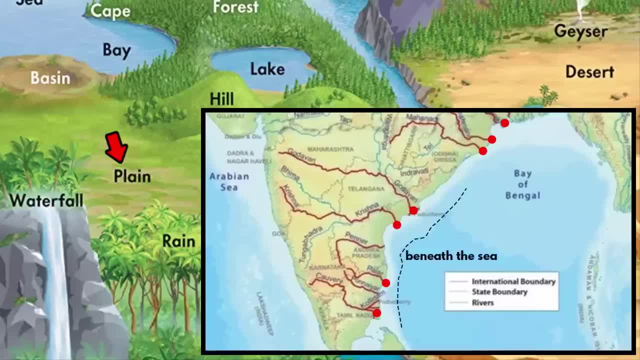 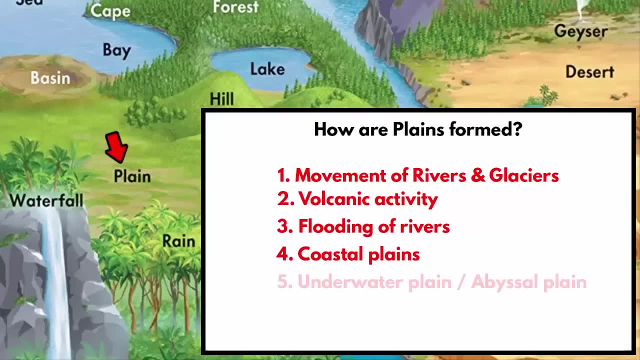 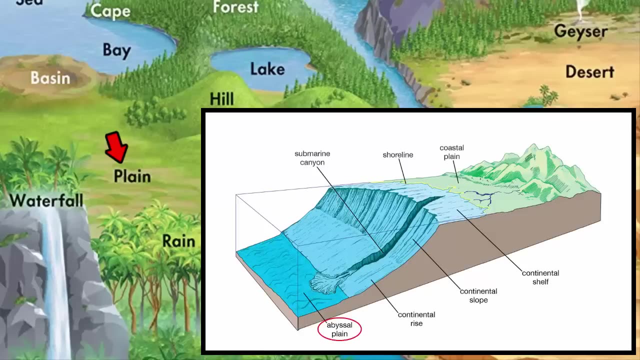 of sediments near coastal area. These coastal planes extend beneath the sea water And, by the way, these coastal planes are also referred to as beach. And then there are something called underwater plane, which are also called abyssal plane. You will find them at the bottom of the ocean. 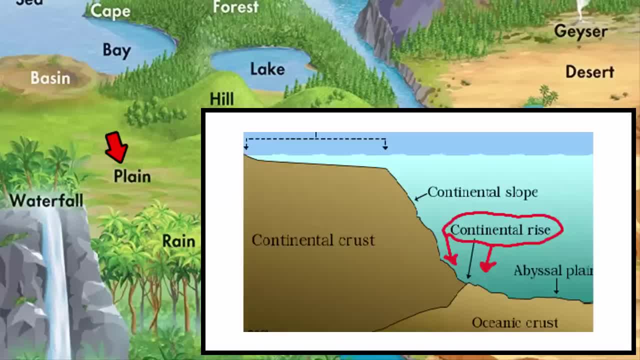 These planes are 5000 to 7000 meters below the sea level, And that is why these planes have not been thoroughly studied. But scientists say that these underwater planes are among the flattest, smoothest places on earth. The next one is: 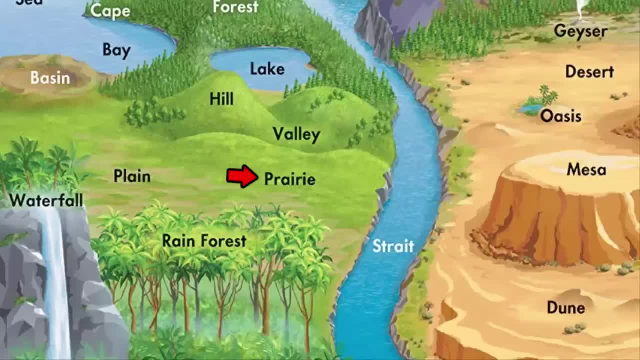 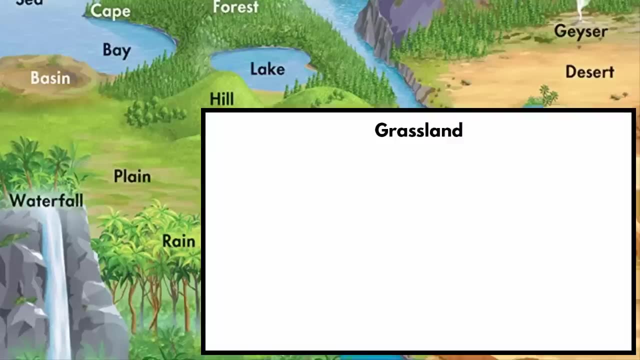 prairie. Prairies are basically flat fertile lands dominated by grasses. You can also call them grasslands. You will find very few trees Now. grasslands are known by different names in different parts of the world, In Asia and Europe. 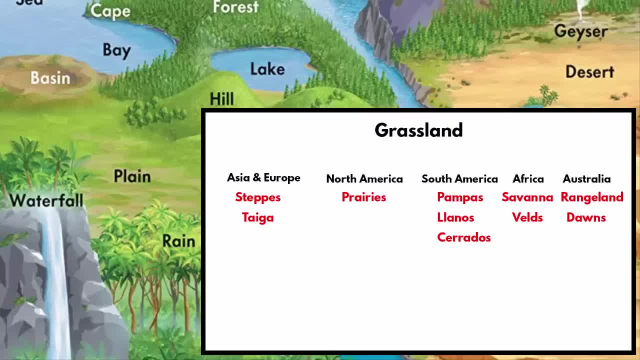 it is called steppes or taiga, In North America it is called prairies. In South America it is called pampas, lanos and cerrados. In Africa they are called savannas and wells, And in 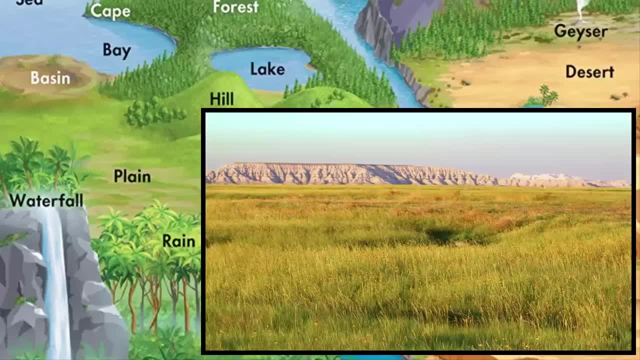 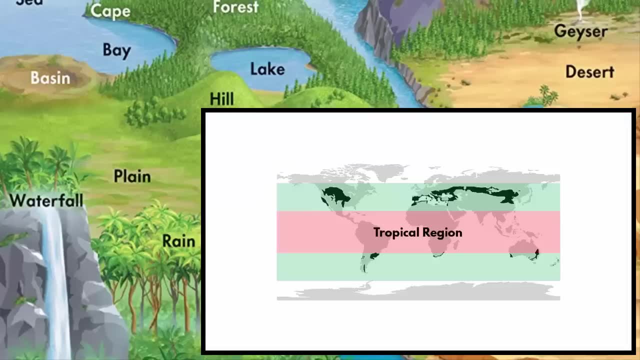 Australia they are called rangelands or downs. The grasses of these grasslands hold the soil firmly in its place. That is why erosion is very minimal. Majority of the grasslands around the world are found between 40 degree and 60 degree north and south. 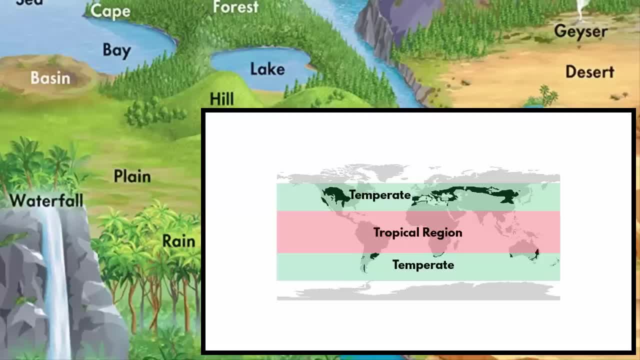 of the equator. That means you will find the grassland in temperate zone. That is why they are called temperate grasslands. If you look at the temperature in this region, it is somewhere between minus 3 to 18 degree Celsius. 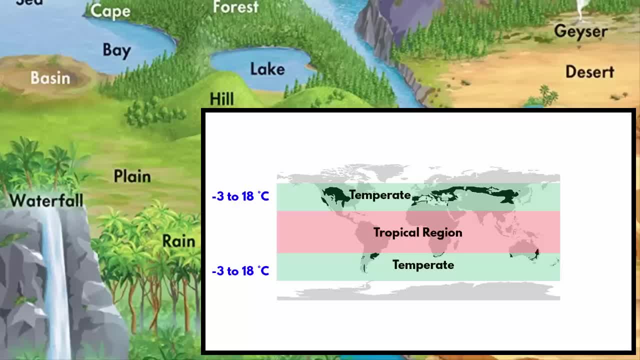 That means the average yearly temperature in this region are not extreme, because the meaning of the word temperate is moderate. Even the precipitation is moderate here. That is why these temperate grasslands are a difficult place for tall plants and trees. In tropical region these grasslands are called 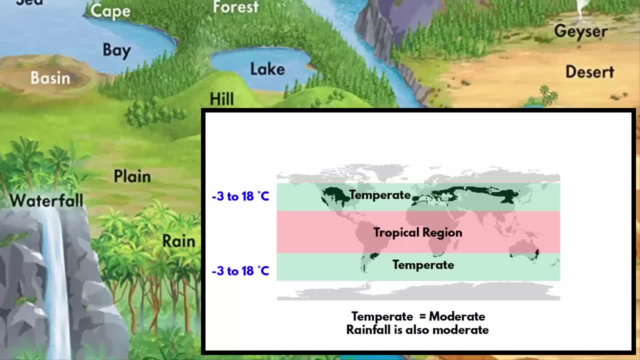 savanna. Here the grasses are a little bit tall because they lie in the tropical region And here the rainfall is a little higher than temperate region because of warm temperature. In India you will find grasslands near the lowland region of Himalayas, the Ganga and the. 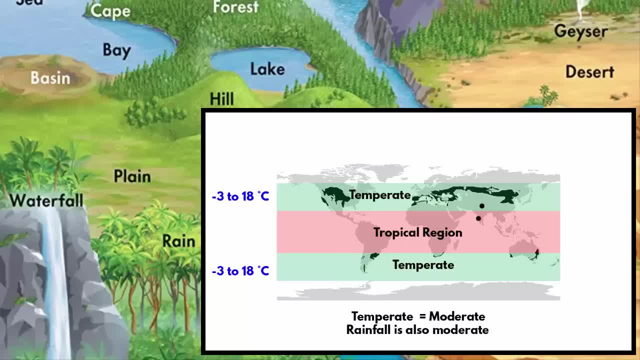 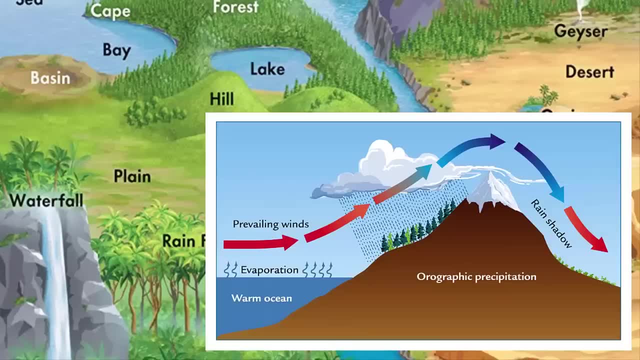 Brahmaputra river basin. You will also find grassland on the eastern side of the western ghats, Because the eastern side of the western ghats is a rain shadow region. Mostly you will find these grasslands very near to a hilly or mountainous region. 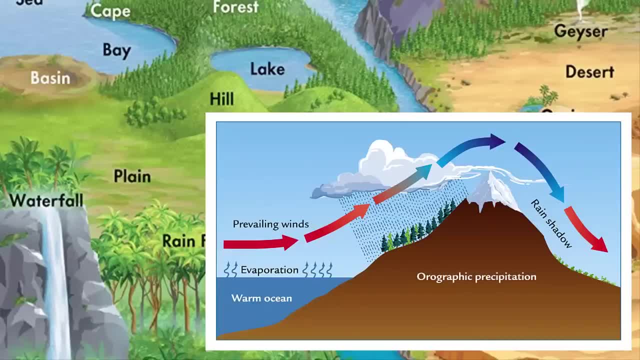 Because these areas are a perfect rain shadow region. That means the amount of rainfall is very low. As a result, here the vegetation is in the form of grass and not in the form of tall trees. The next one is valley. Valleys are one of the most common. 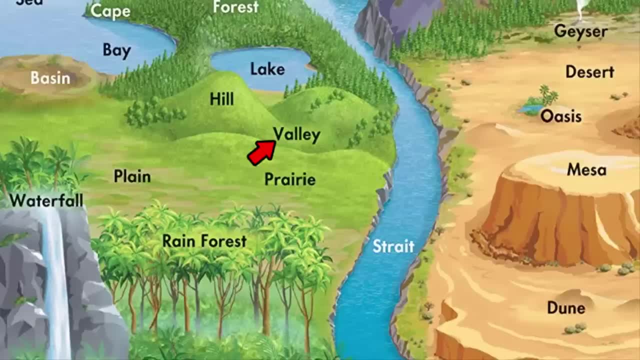 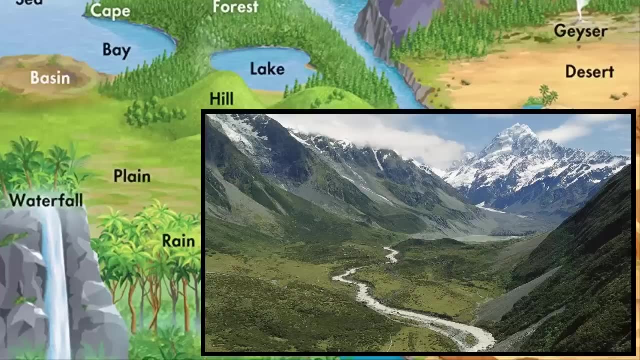 landforms on the earth, and they are formed through erosion or the gradual wearing down of the land by wind and water. In river valleys, for example, the river act as an erosional agent by grinding down the rock or soil and creating a valley in between the 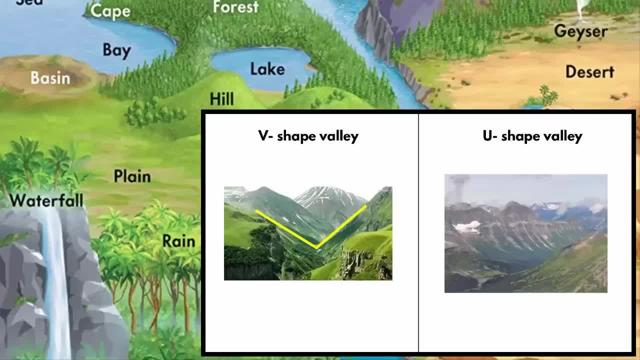 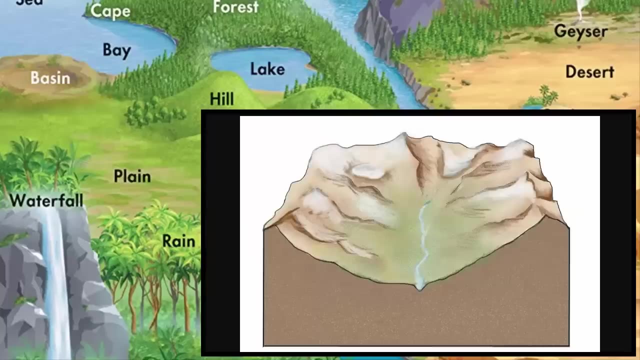 mountains and hills. Valleys are usually in the form of U and V shape. Rivers and streams do most of the work in carving hills and mountain slopes to form valley, Hence forming a landform that looks like the letter V. Even glaciers do the same work. what rivers and streams 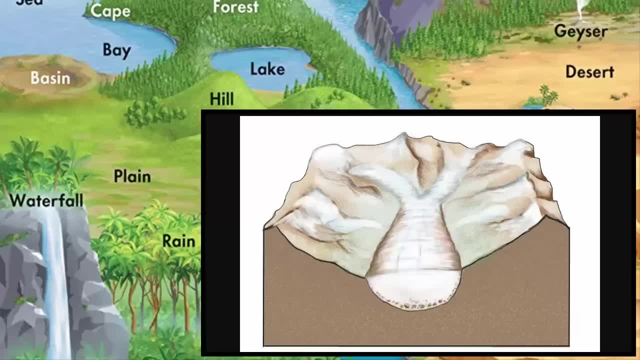 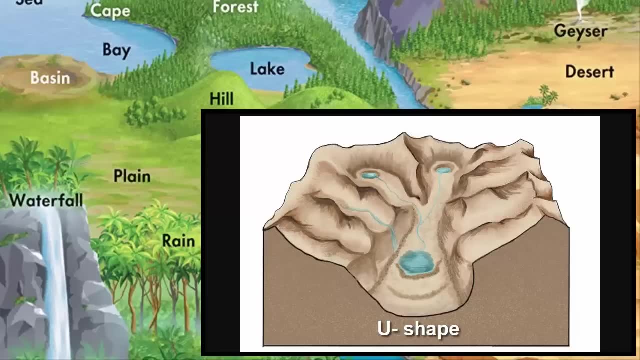 do. As the glaciers move, they grind the valley floor and carve it in the form of letter U. When the glacier melts, a U shaped valley marks the spot where the snow and ice once flowed. In India, you will find many V shaped valleys in the 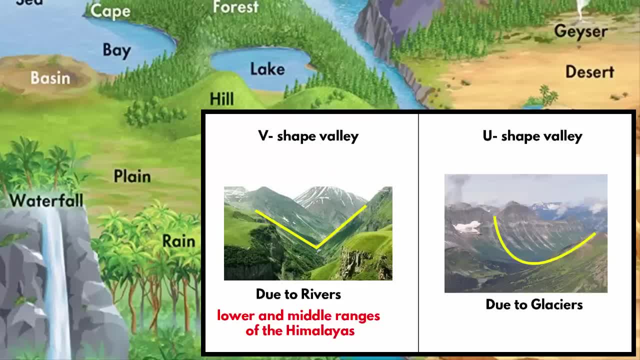 northern states and northeastern states. In these places, most of the V shaped valley are found in the lower and middle ranges of Himalayas, Because the upper Himalayas, or the greater Himalayan ranges, have glaciers, And I already told you that with glaciers, you will 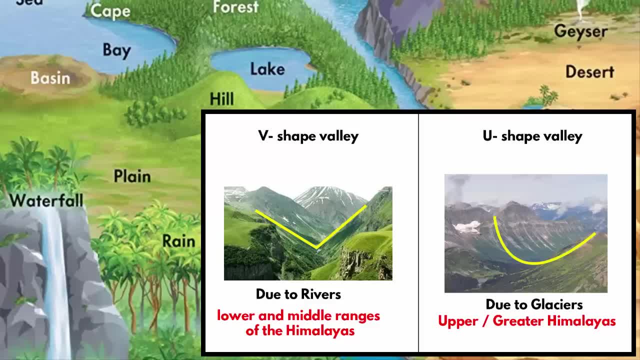 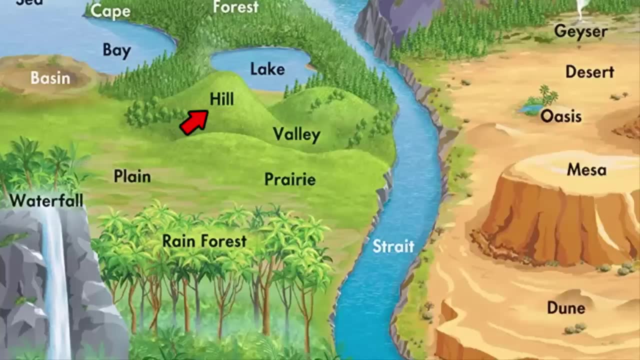 find U shaped valley. Apart from north and northeast India, you will also find mountains in central as well as southern part of India. Since there is no ice or glacier in lower latitudes of India, naturally you will find V shaped valleys. The next one is hill. 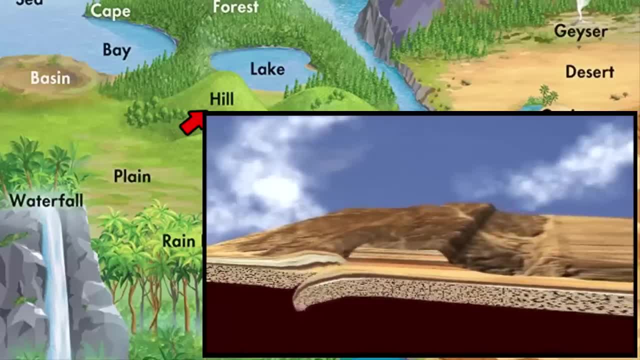 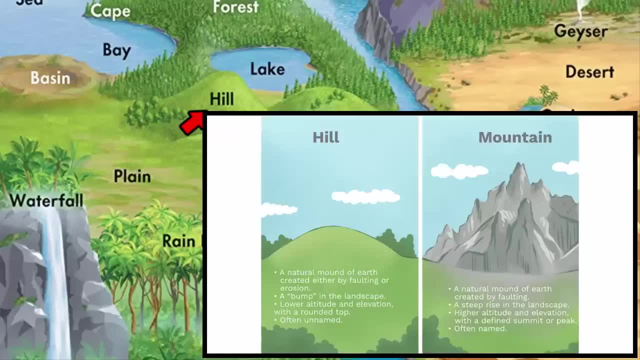 We have already covered how mountains are formed. Plus, there is no actual difference between hills and mountains. The only difference you can see is the height. Hills are not as high as mountains. Hills can be both natural as well as man made. Suppose if you dump piles. 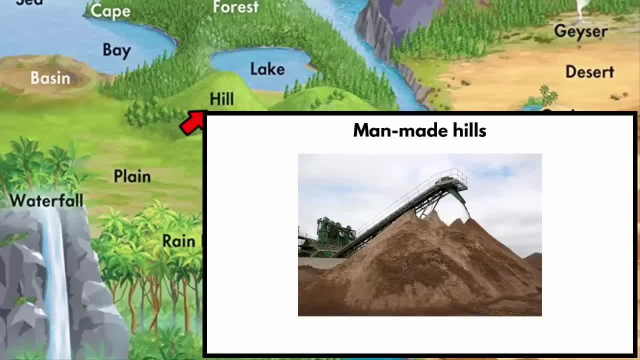 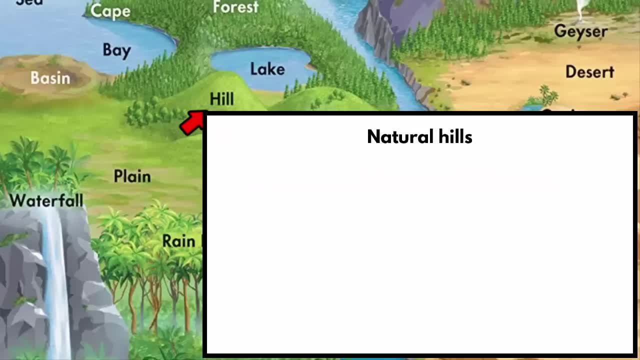 of sand, mud or earth material at one place. eventually it will turn into a huge stack, which is also a hill. It is actually called a mound, But when we talk about natural hills, they are formed by different types of geologic activity. One is faulting 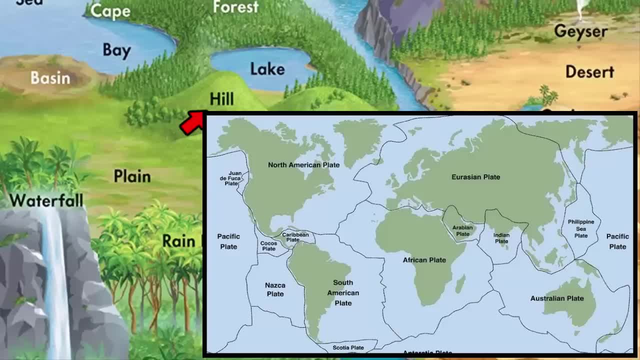 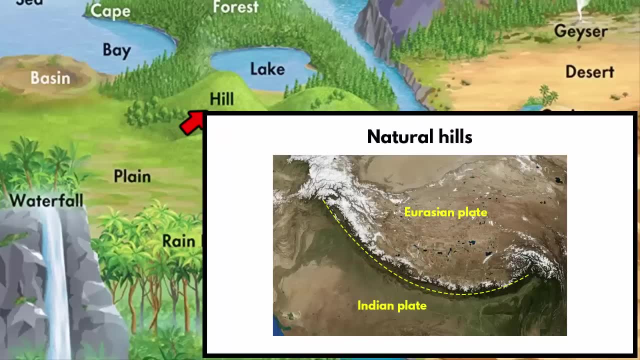 A fault lies at the major boundaries between earth's tectonic plates. These earth's tectonic plates are constantly moving and changing the landscape. The Himalayas are a good example. They were once tiny hills. The Himalayas continues to grow because 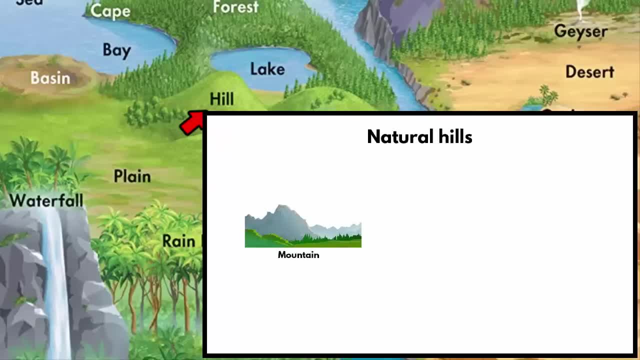 of faulting activity beneath the earth's surface. Hills can be created by erosion. A mountain which is bigger than a hill, it can be worn down by erosion. What I am trying to say is: hills may have once been mountains that were worn down by erosion over many. 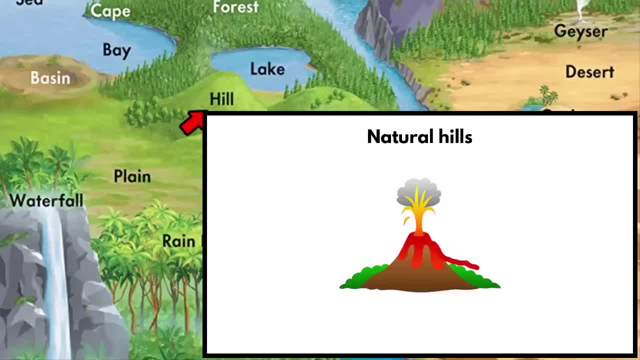 thousands of years. Hills can also be formed due to volcanic eruption. When a volcano erupts, it releases large amount of lava. When this lava gets accumulated at one place in multiple layers, it turns into plateau. If you see, all plateaus are. 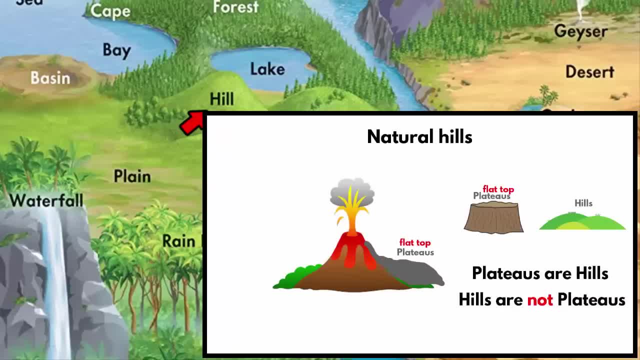 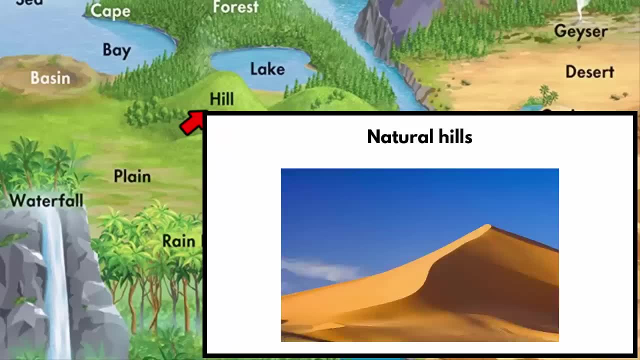 hills. but not all hills are plateaus, Because plateaus are hills with a flat top. That means these volcanic plateaus are also volcanic hills. Even a sand dune in a desert is a hill. It is called a hill of loose sand In Antarctica. 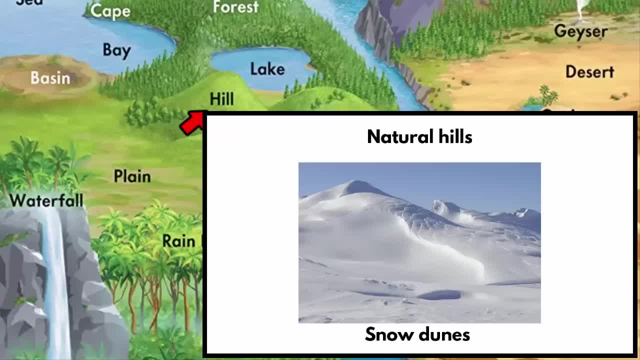 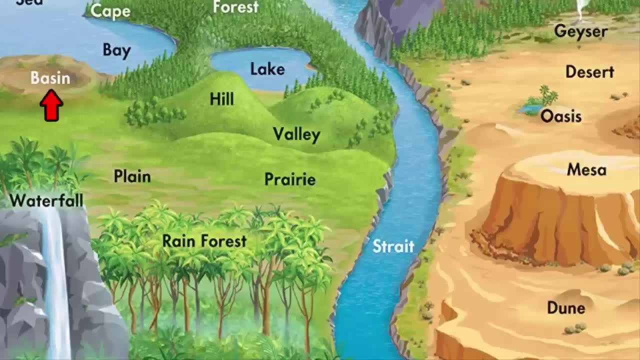 there are snow dunes that are formed by wind, blowing snow into large piles. As a result, they turn into ice hills. The next one is basin. When you look at a basin, basically it is a depression Or a dip in the earth's surface. 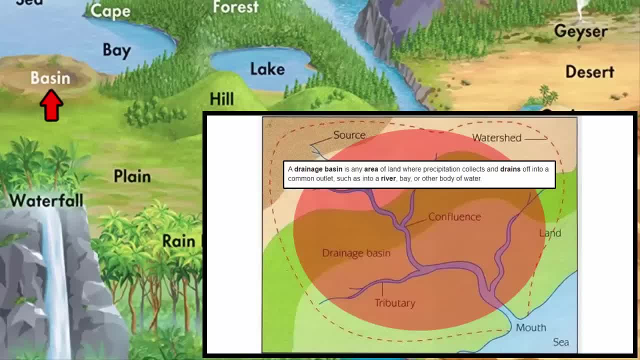 When you look at the shape, it looks like a ball and its sides are higher than the bottom. They are also in oval and circular in shape, Similar to a sink or a tub you might have seen in your bathroom. Some basins are filled. 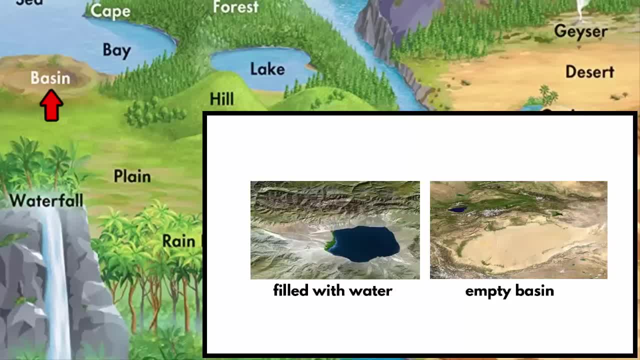 with water, and then there are ones that are empty. They are formed over thousands of years or almost overnight If it is through erosion. when a ground gets eroded, it takes thousands of years. A good example of overnight activity would be an earthquake. 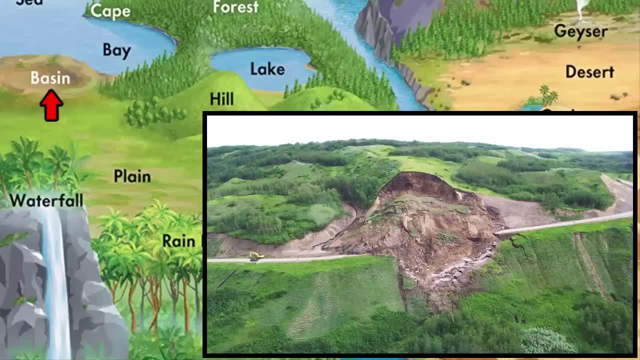 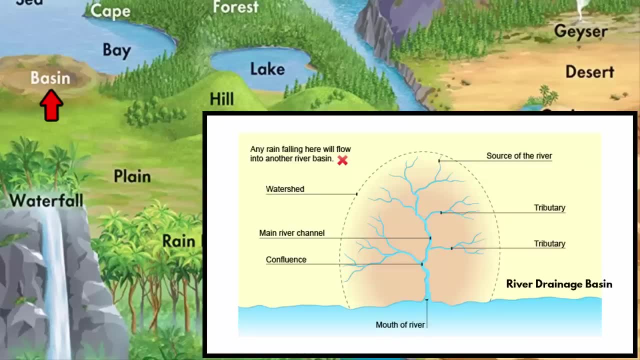 Earthquake makes the ground shake, due to which a landslide is triggered, and that's how a basin is created. A river drainage basin is an area drained by a river and all of its tributaries. Heavy and continuous flow of water sinks some land and accumulates in other places. 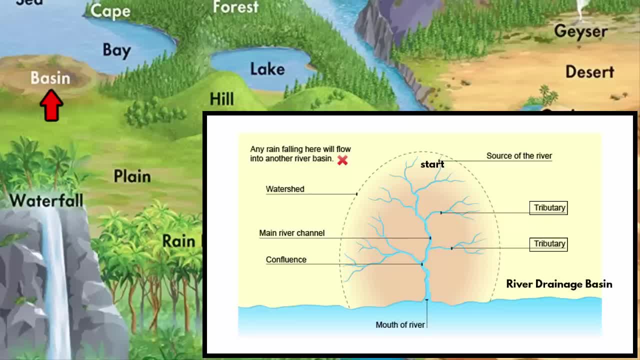 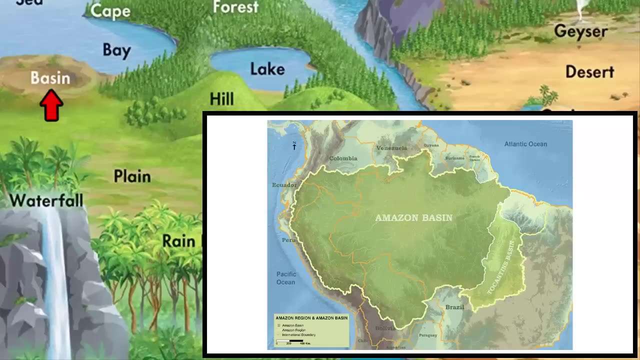 This process is called erosion. Heavy and continuous flow of water picks up sand particles along the way, causing land erosion. The land that is taken away is now lower than the other land. Basins usually take thousands of years to form The Amazon basin in. 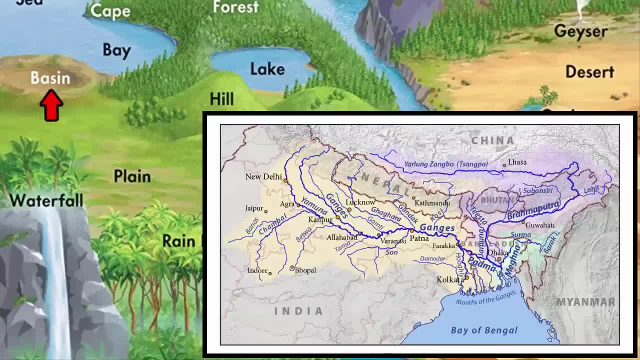 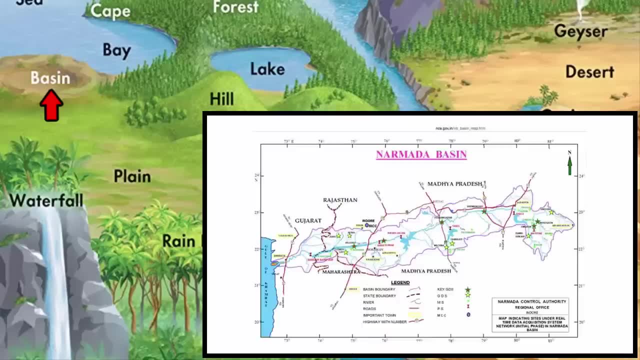 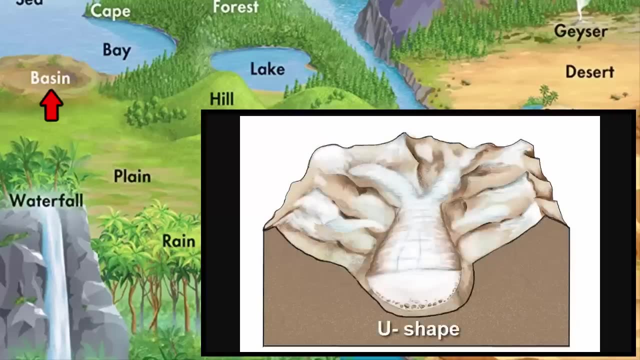 northern South America is the largest in the world. In India we have Ganga river basin, Brahmaputra river basin, Krishna river basin, Mahnadi river basin and Narmada river basin. Even slow movement of glaciers forms basin. Glacier movement carves the land creating. 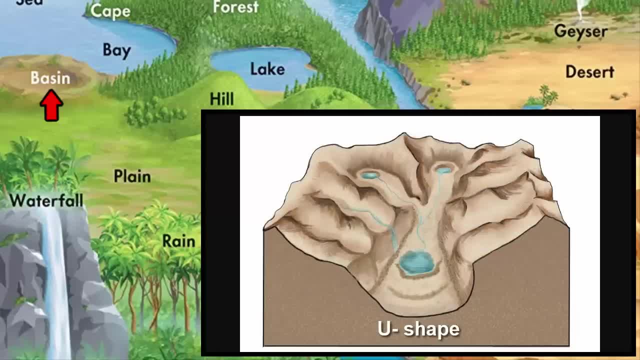 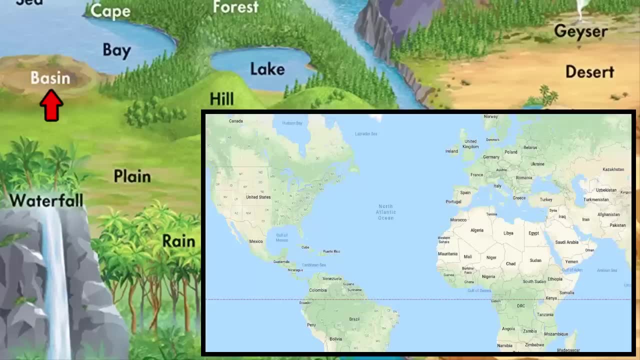 a low ground or depression. As a result, you have an area of land which is lower compared to its surrounding, And this is exactly called a basin. And finally, when you look at an ocean, it is a large portion of earth's crust that is filled with water. 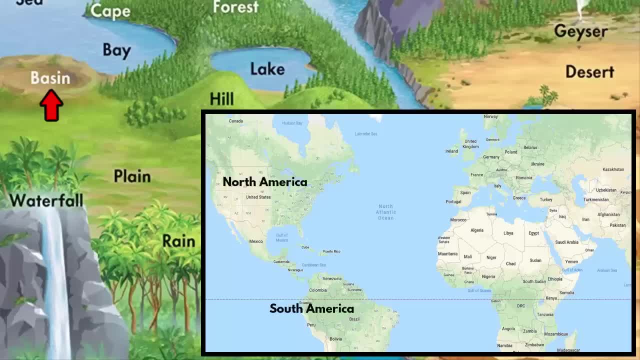 Let's take the example of Atlantic Ocean. We have North and South America on left and Europe and Africa on the right. In between them there is a low land that is filled with water, which we call the Atlantic Ocean. That means an ocean is a. 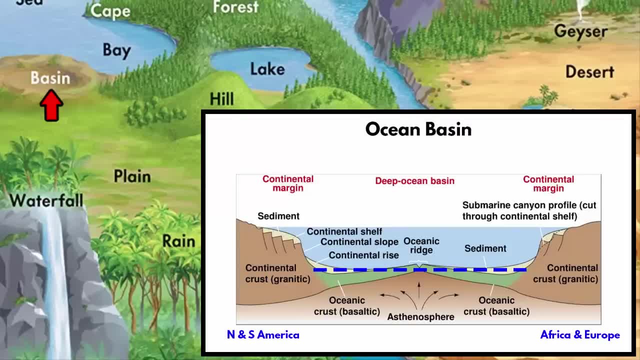 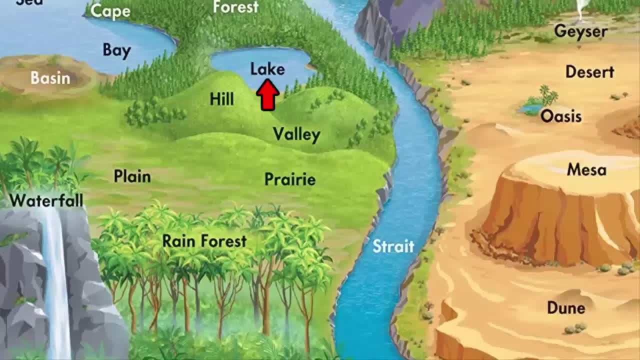 low land between two continental land mass that is filled with water, So in a way it is a huge basin. It is called as Ocean Basin. The next one is Lake. A lake is a body of water that is surrounded by land. Most of the lakes are. 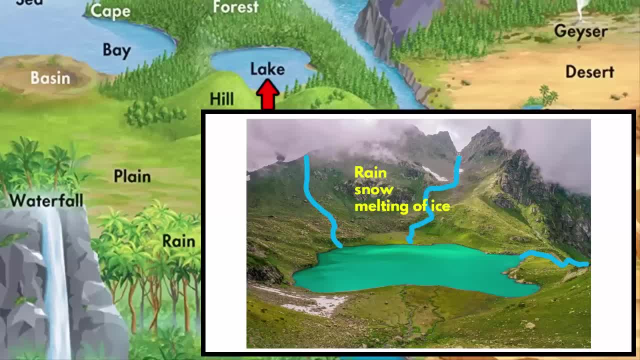 fed and drained by rivers and streams, which get water from rain, snow, melting, ice and groundwater seepage. That means a lake is a low lying land, which you can also call a basin. That's how a lake will have water. Lakes are found in every kind of 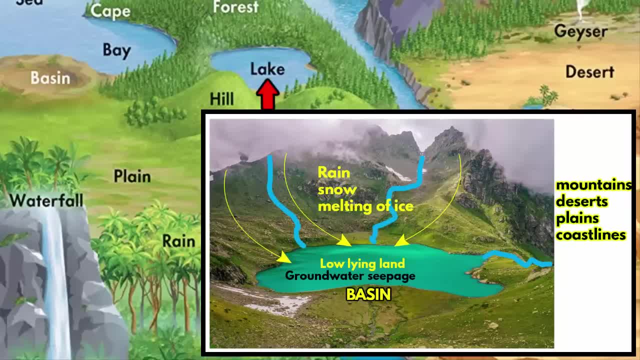 environment: Mountains, deserts, plains and near coastlines. Lakes are both small as well as big in size. Small lakes are often referred to as ponds, Whereas a big lake can also be called as sea. The Caspian Sea in Europe and Asia is the world's. 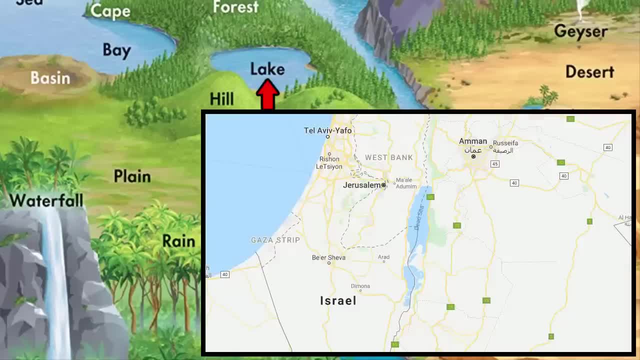 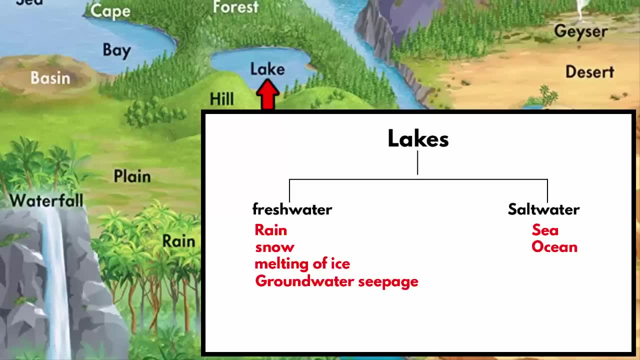 largest lake. Then there is Aral Sea. Dead Sea Lakes are both freshwater as well as saltwater, But most of them are freshwater. You can figure that out by looking at the water source. Saltwater lakes usually exist near coastal areas, And 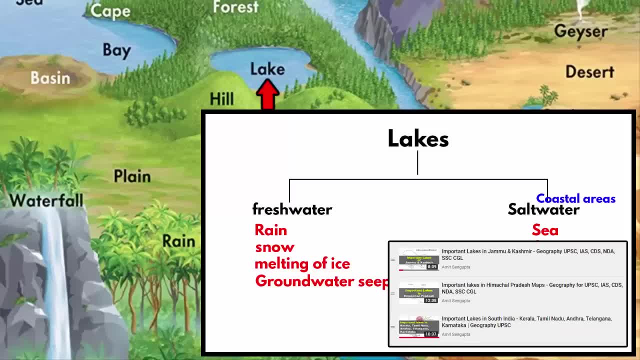 I have a playlist dedicated to lakes in India. In that you will find videos describing lakes that exist in different parts of India. Have a look at it. you will learn a lot about Indian lakes. Lakes also vary greatly in depth. The world's deepest lake is Lake Baikal. 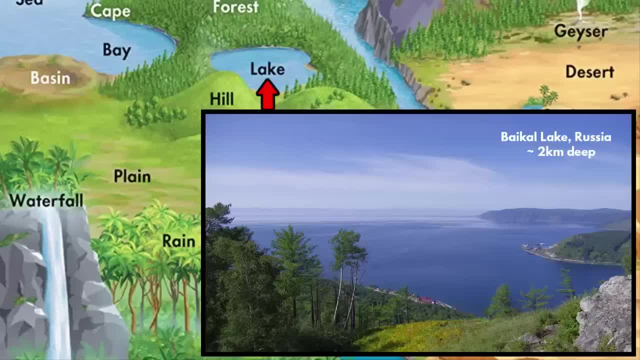 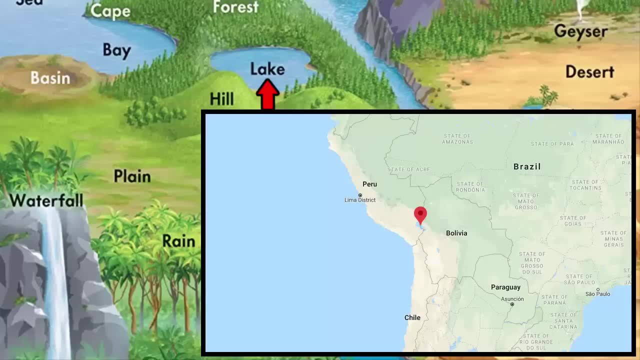 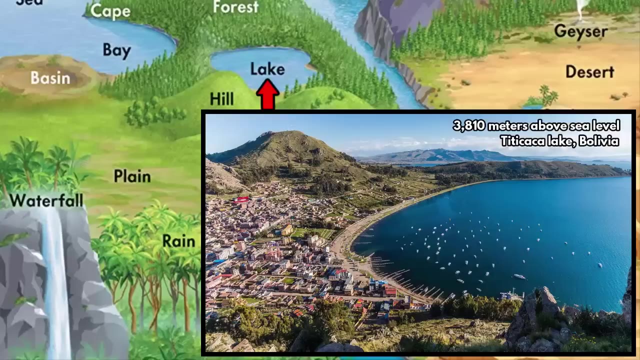 in Russia It is nearly 2 km below the surface. Lakes also exist at many different elevations. One of the highest lake is Lake Titicaca in the Andes Mountains between Bolivia and Peru. It is about 3810 m above sea level. 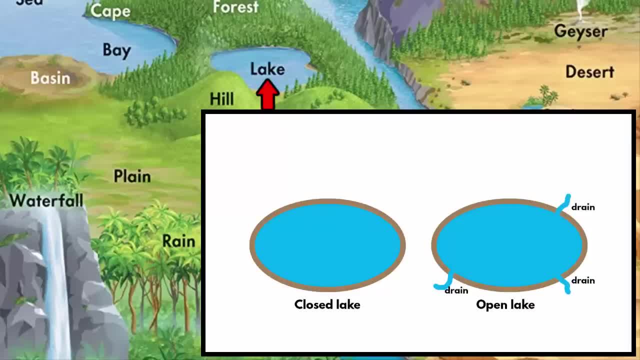 All lakes are either open or closed. If water leaves a lake by a river or other outlet, it is said to be open. All freshwater lakes are open. If water only leaves a lake by evaporation, the lake is closed. Closed lakes usually become 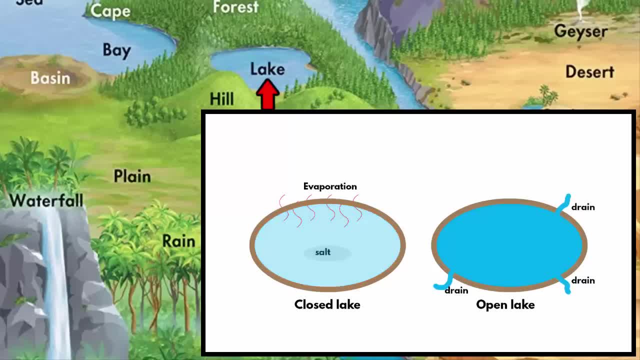 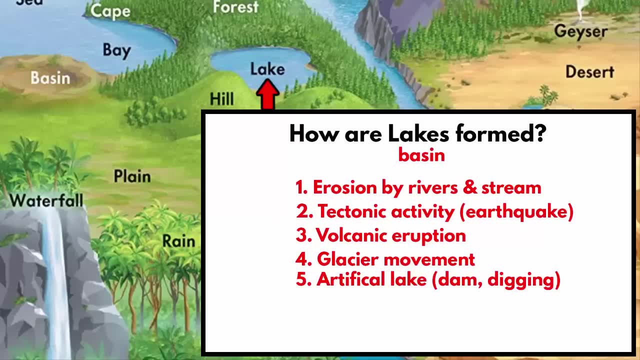 saline or salty. This is because, as the water evaporates, it leaves behind solids, mostly salts. As I have said, lakes are basically basins. In the previous point we saw how basins are formed. They are formed by constant erosion processes of rivers and streams. 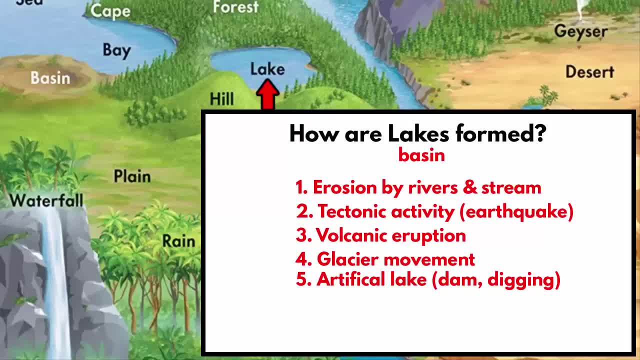 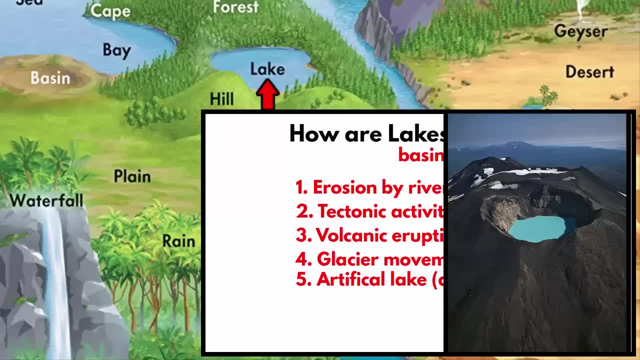 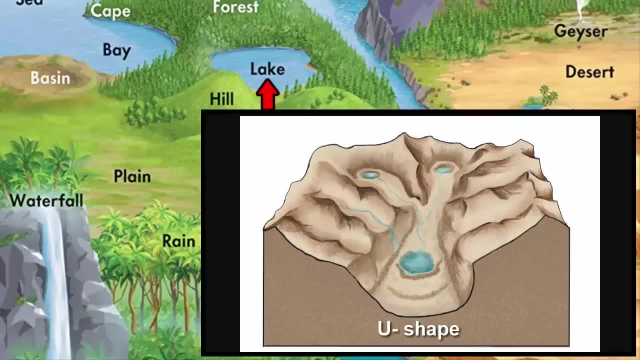 They are also formed due to tectonic activity like earthquake, which triggers a landslide. After a volcano becomes inactive, its crater gets filled with rain or melted snow. Many lakes form as a result of volcanoes. Even glacial activities can contribute towards the formation of 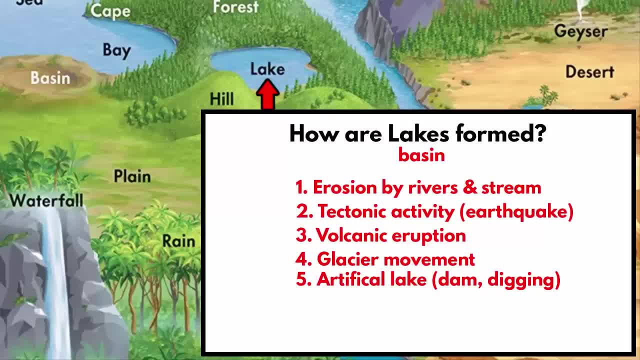 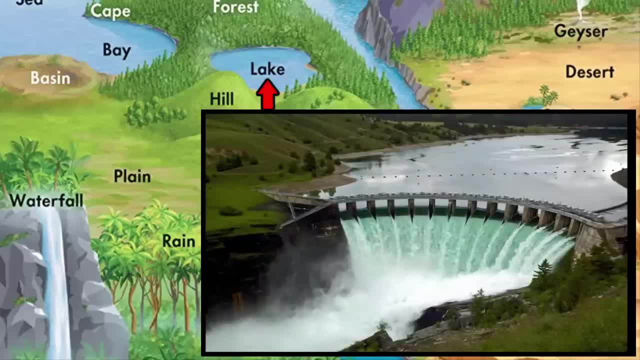 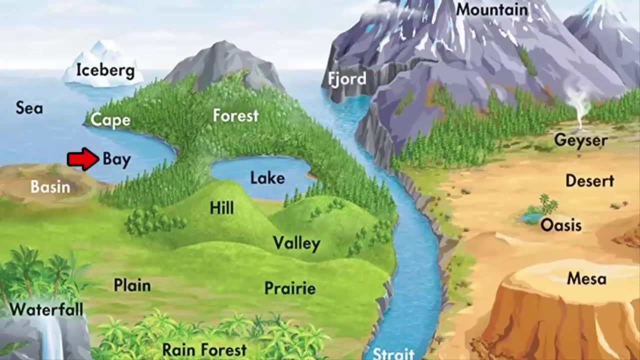 a basin. Then there is something called artificial lake. People make lakes by digging basins or by building a dam on a river. These artificial lakes can become reservoirs storing water for irrigation, hygiene and industrial use. The next term is bay. 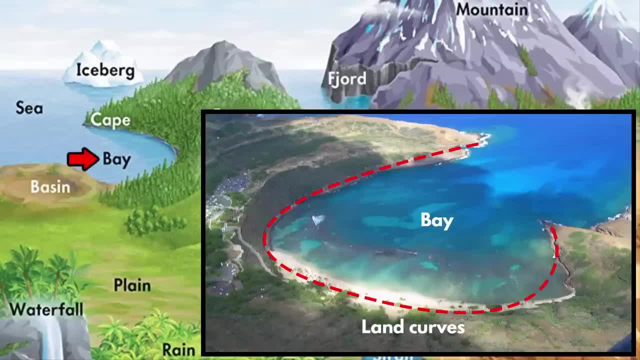 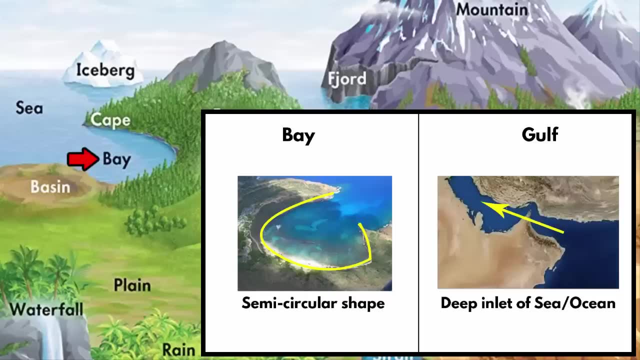 A bay is a broad inlet of the sea where the land curves inwards. A bay can also be called as a gulf, But the only noticeable difference you will find is that a bay is semi-circular in shape, Whereas a gulf is a deep inlet. 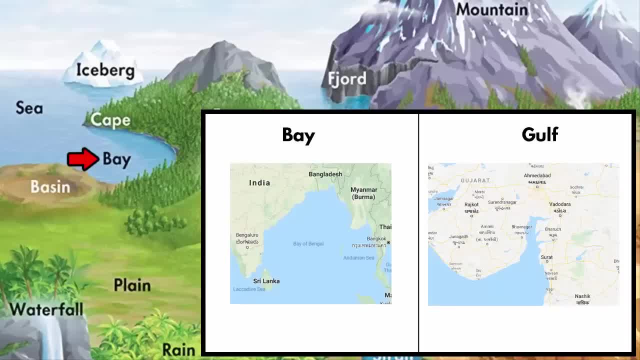 For example, have a look at the bay of Bengal and the gulf of Khambath. If you look at the landmass around the bay of Bengal, it is in semi-circular shape. On the other hand, if you look at the gulf of Khambath, the sea or 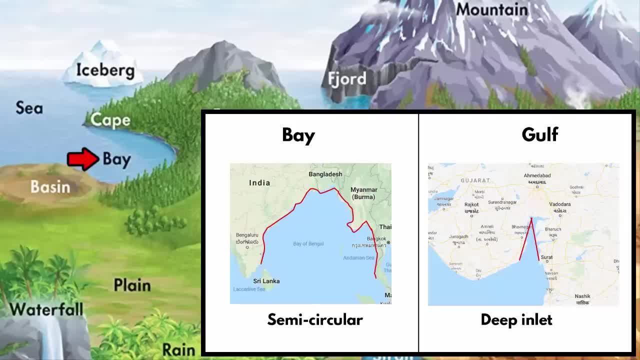 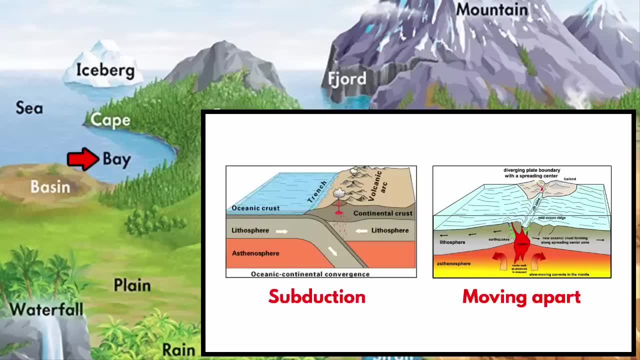 ocean water goes deep inside the landmass. That means a gulf has a deep inlet of the sea or ocean Bays form in many ways. One of it is plate tectonics. The process of continents drifting together and drifting apart causes the formation of many 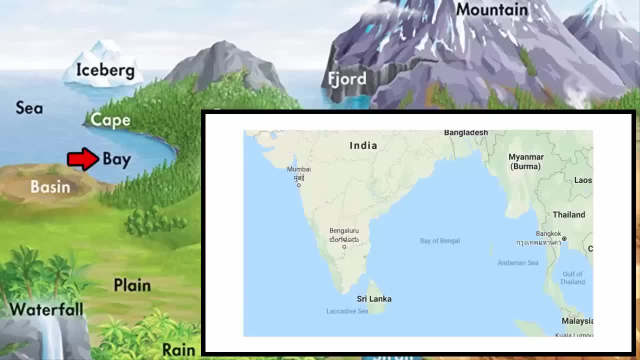 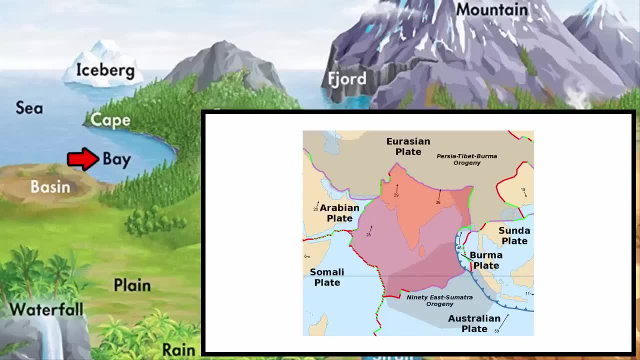 large bays. The bay of Bengal, which is the largest bay in the world, was formed by plate tectonics Millions of years ago. the Indian subcontinent crashed and continues to crash into the massive Eurasian plate. Near the bay of Bengal region, the Indian 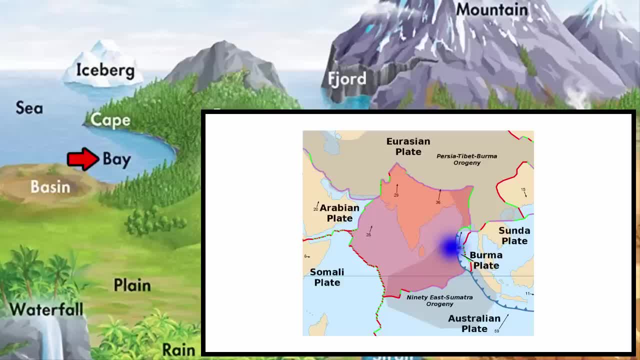 plate is subducting beneath the small Burma plate Plate. tectonics remain an active force in the bay of Bengal today. This region is home to underwater earthquakes and tsunamis. Bays are also formed when the ocean overflows a coastline. 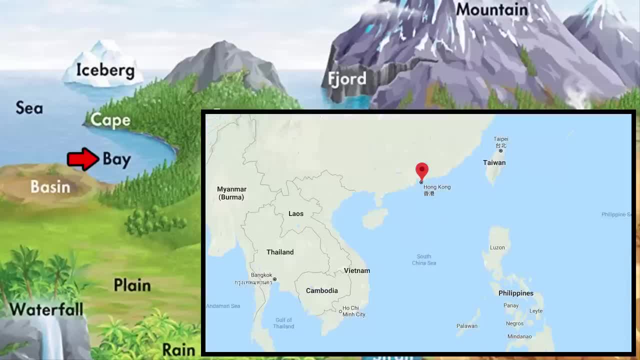 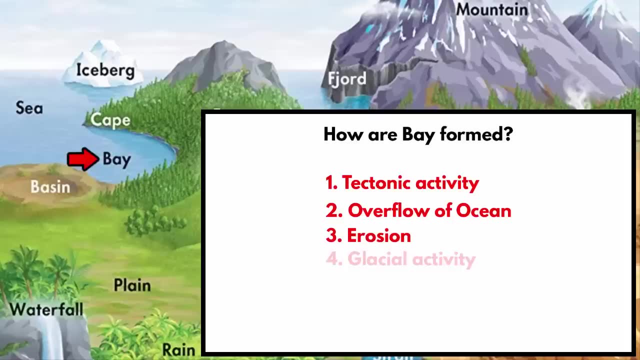 The Kowloon Bay in Hong Kong was formed as the South China Sea overflowed the coastline of the Kowloon Peninsula. Bays are also formed due to erosion. Many times the ocean erodes the entire coastline, forming a bay, For example. 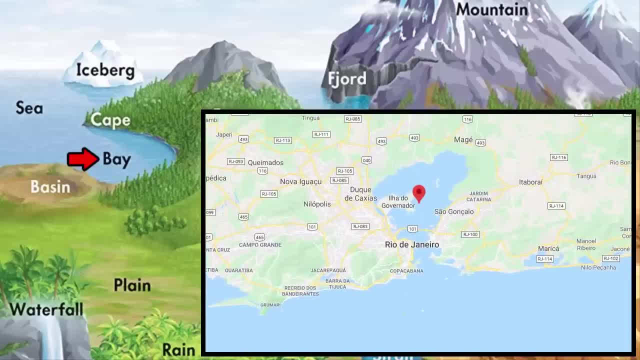 the Guanabara Bay. It is located in Southeast Brazil, in the state of Rio de Janeiro. This bay was formed as the Atlantic Ocean eroded an inlet in South America. I want you to recollect jods, If you remember they are. 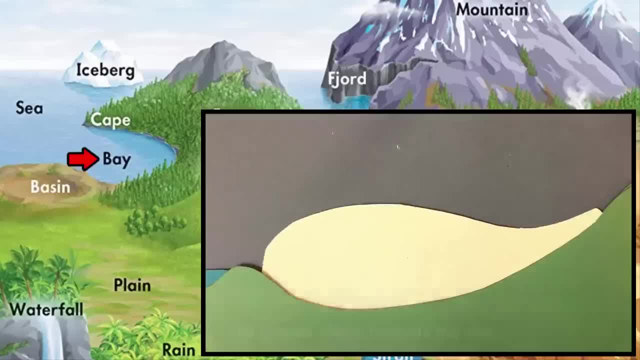 formed by slow movement of glaciers. A glacier slices through the bedrock of an area, leaving a long, steep canyon which gets filled up with sea water. So even a jod is a bay. The next one is Cape. A cape is a narrow. 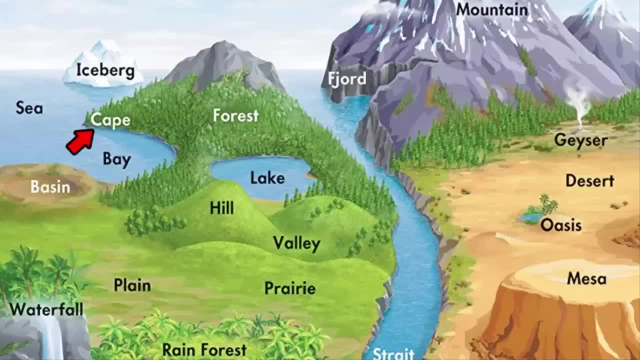 portion of land that extends into a river, lake or ocean. Now, this narrow portion of land can be a part of a large land mass, or it can also be a part of an island. If you look at the shape of a cape carefully, it does look like. 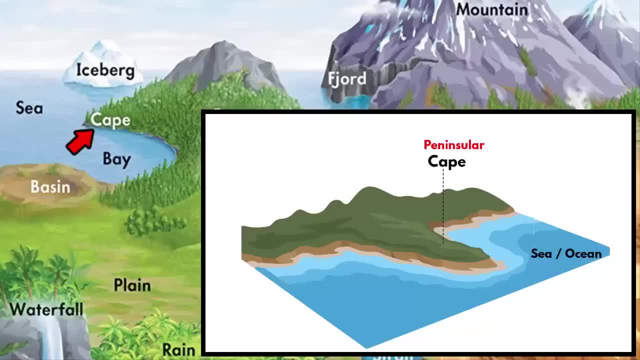 a peninsula, isn't it? Many geographers consider capes to be smaller than peninsulas. The only difference is that a cape is a narrow feature and a peninsula is a large, Since the land form is a narrow extension into the sea or ocean. you can easily figure out.